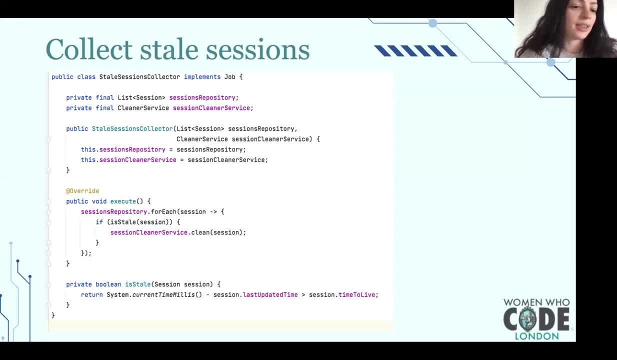 Which means that this session is already expired And nobody wants to use it anymore. So we say that this is some property of session. It means that session is stale. So we create with isStale session method which means basically that current time minus session, last updated time more than. 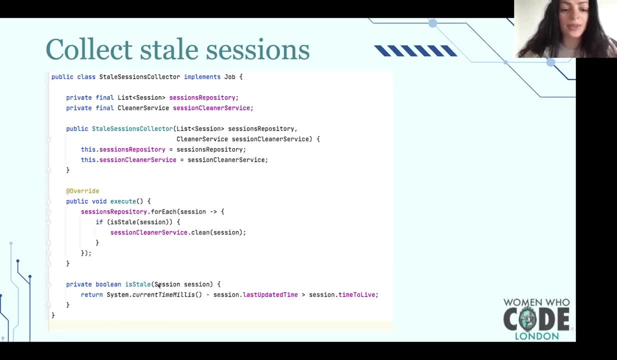 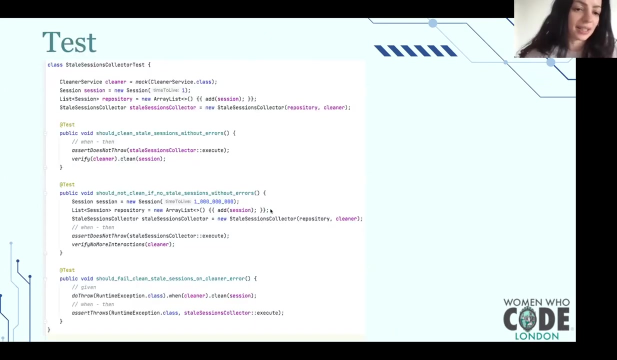 session time to leave. if you see, it's on the bottom and we want to collect all this, all the style sessions, and we will clean them. so looks good and looks simple and looks clean. now we need to cover it by tests. so how tests will look like under here. okay, someone please mute yourself. okay, I need to check. so. 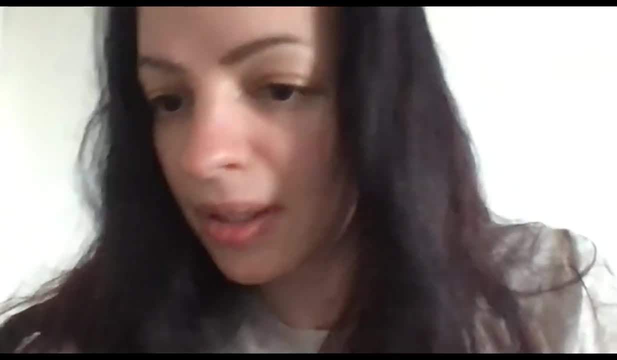 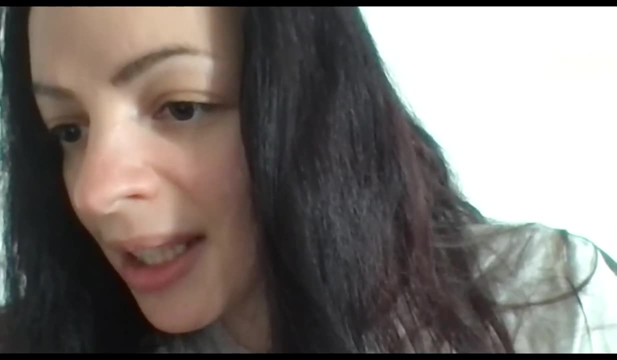 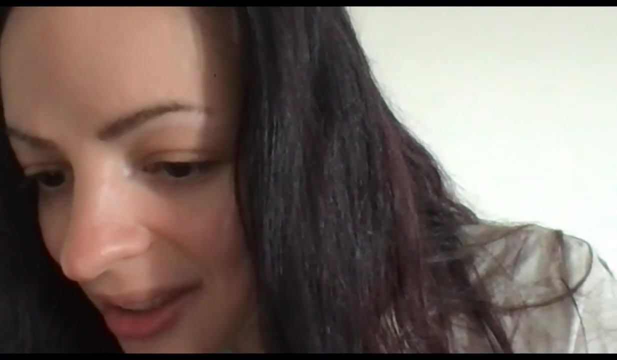 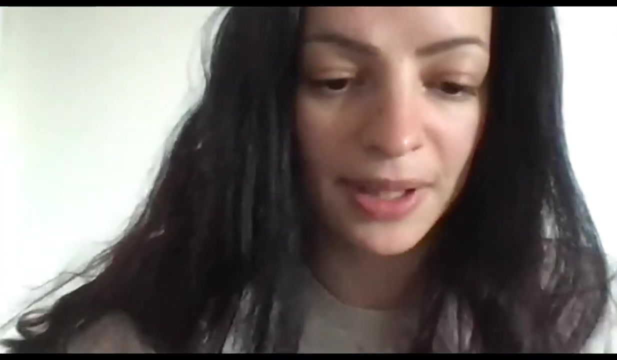 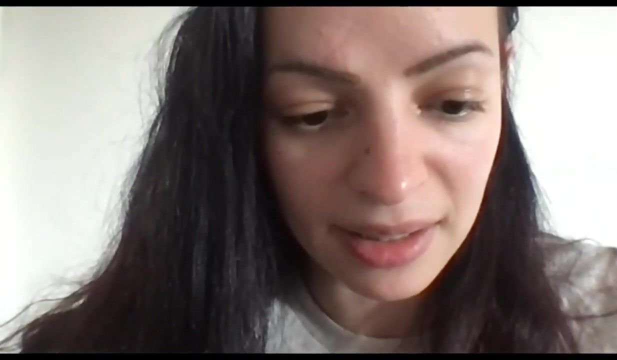 probably. I stopped pairing because I need to check who hasn't been muted. okay, see several people who I need to mute. sorry for this, and now I can check. okay, so I think it should be fine. please let me know again if you will have any questions and 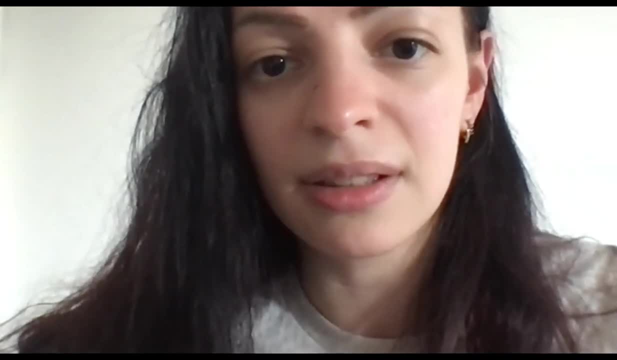 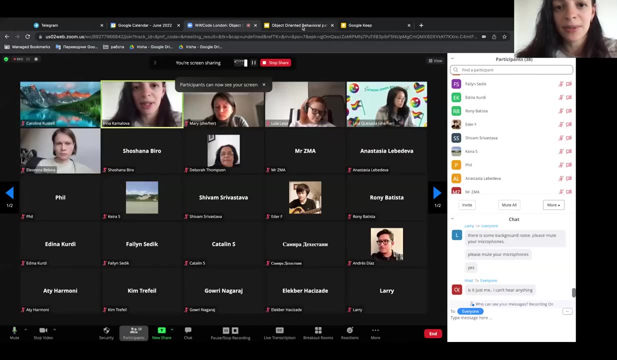 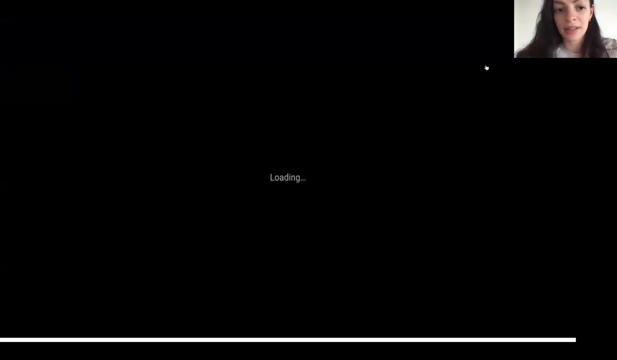 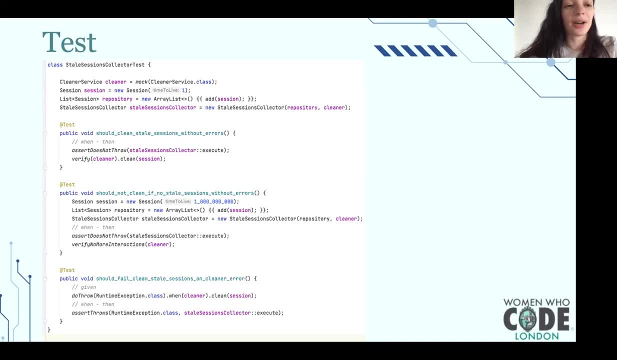 yeah and we are here. so how are we going? yeah and we are here. so how are we going? yeah and we are here. so how are we going to test our application? we should create to test our application. we should create to test our application. we should create at least three tests. 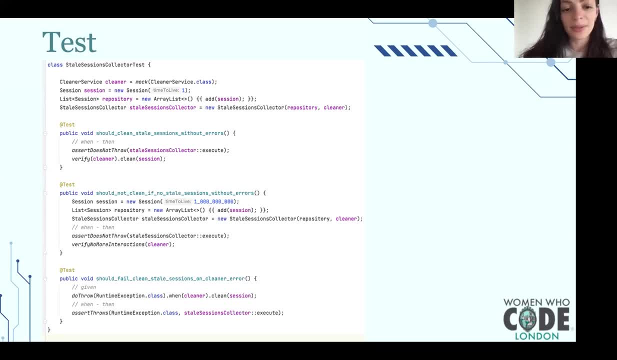 at least three tests. at least three tests, because first of all we need to check that, because first of all we need to check that, because first of all we need to check that everything, everything, everything can work without any errors, can work without any errors, can work without any errors. so 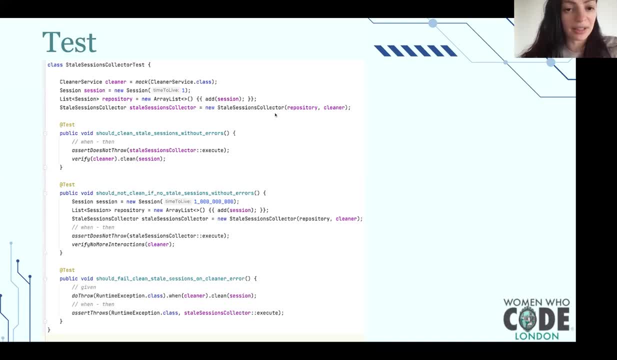 so so we create our object style session. we create our object style session. we create our object style session. collector with some, collector with some, collector with some, any mocked repository, for example, a release, can be repository. for example, a release can be repository. for example, a release can be repository. we just put them in the list. 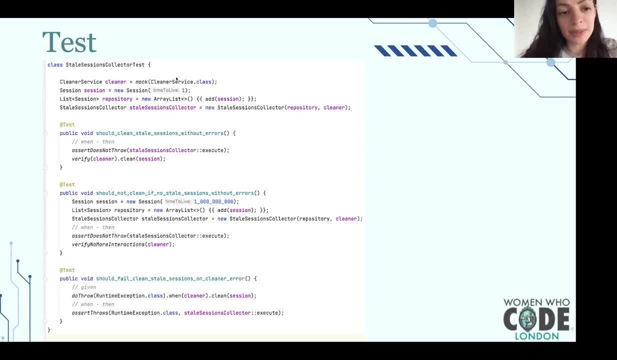 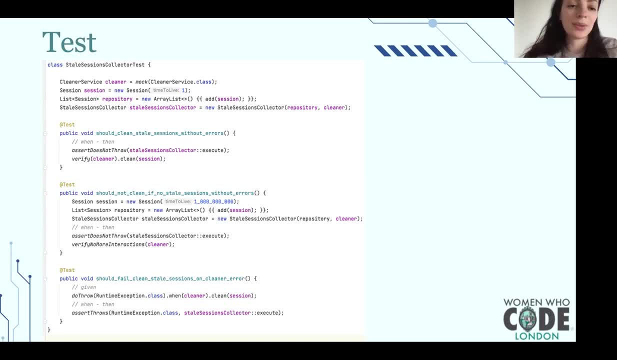 this is called mock and it's used by. this is called mock and it's used by: mockita in java. it's powerful instrument, mockita in java. it's powerful instrument, mockita in java, it's powerful instrument to test everything you like by just to test everything you like by just. 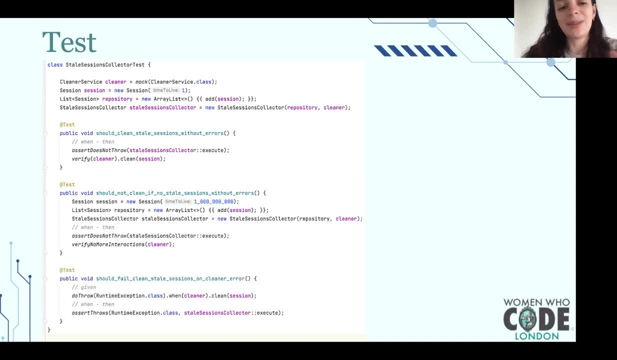 to test everything you like by just mocking objects, by just pretending that mocking objects, by just pretending that mocking objects, by just pretending that this object exists, this object exists, this object exists, and you also can say what exactly the. and you also can say what exactly the. and you also can say what exactly the behavior of the object. 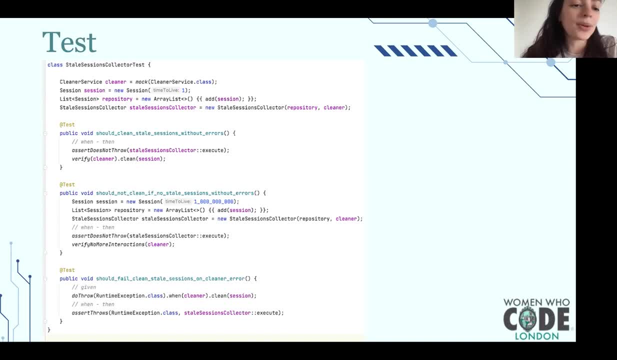 behavior of the object. behavior of the object. so the first test? uh, it's like we don't. so the first test? uh, it's like we don't. so the first test? uh, it's like we don't have to throw any exceptions, have to throw any exceptions. 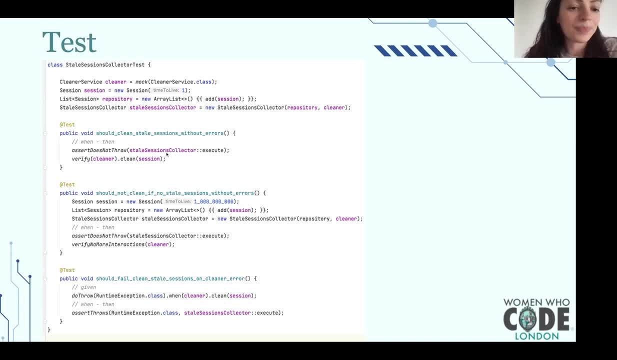 have to throw any exceptions. everything should work when we do. everything should work when we do. everything should work when we do style session collector, when we do style session collector, when we do style session collector when we do execute method, execute method, execute method. also with this, with this reference, i hope you know a bit about. 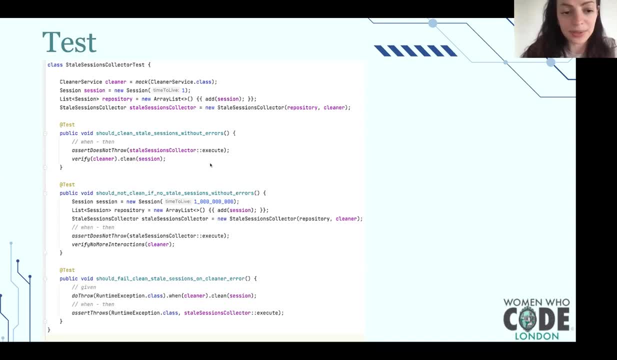 with this reference i hope you know a bit about. with this reference, i hope you know a bit about java 8 syntax. but again, if you don't know java 8 syntax, but again, if you don't know java 8 syntax, but again, if you don't know, if you don't understand what's written, 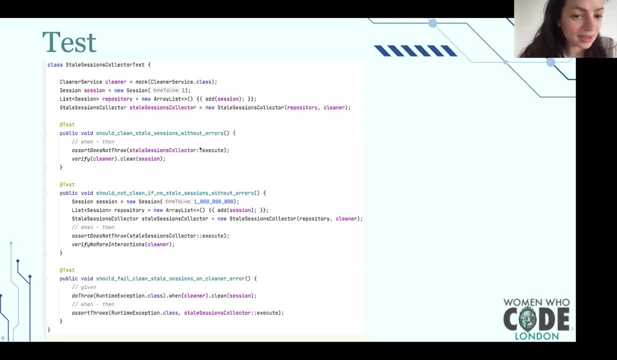 if you don't understand what's written. if you don't understand what's written here, please let me know here. please let me know here, please let me know. so here we just execute style session. so here we just execute style session. so here we just execute style session. collector. 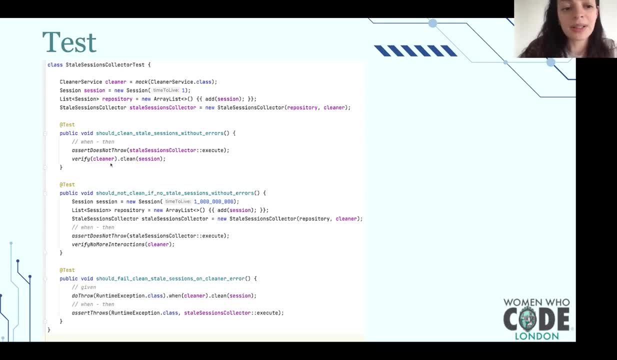 collector, collector, and we also verify that our mock and we also verify that our mock and we also verify that our mock cleaner, actually cleaned session. cleaner, actually cleaned session. cleaner, actually cleaned session. that's how we can check that our function. that's how we can check that our function. 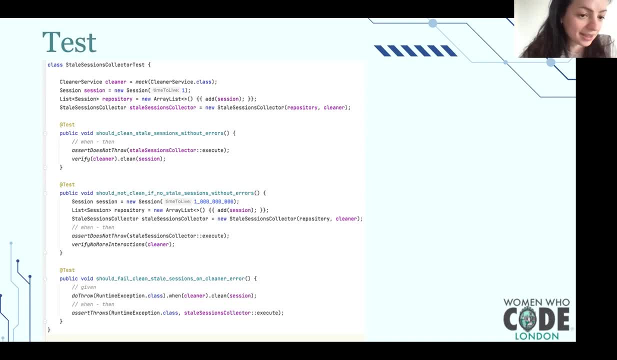 that's how we can check that our function come into method, come into method, come into method and did this method. so again, if you and did this method, so again if you and did this method. so again, if you looked at the code, looked at the code, looked at the code, we see that execute. basically, if 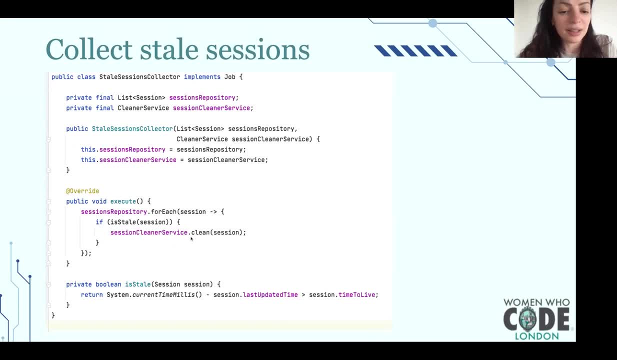 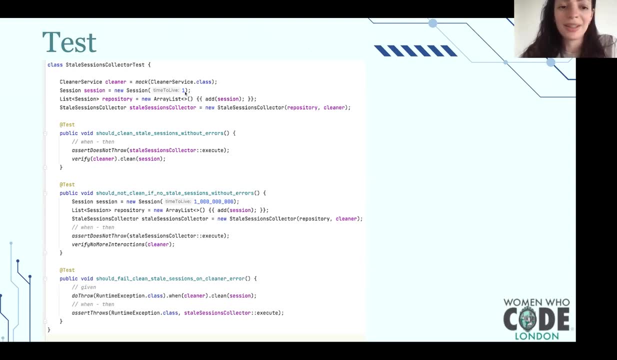 we see that, execute basically. if we see that, execute basically, if there are style session, there are style session, there are style session. we just clean this session. okay, we just clean this session. okay, we just clean this session. okay, we also created session. we also created session. we also created session, this time to live in one. 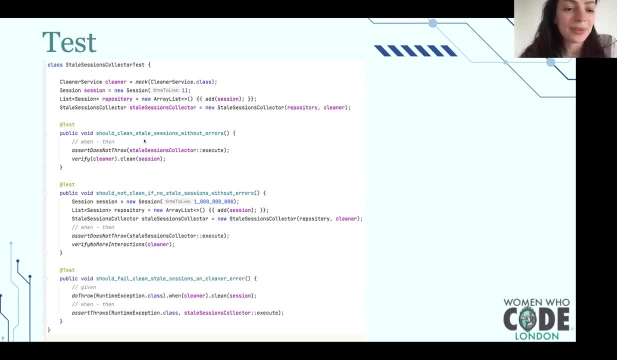 this time to live in one. this time to live in one, one mile second. that's why we can show one mile second. that's why we can show one mile second. that's why we can show when we come into this test, when we come into this test. 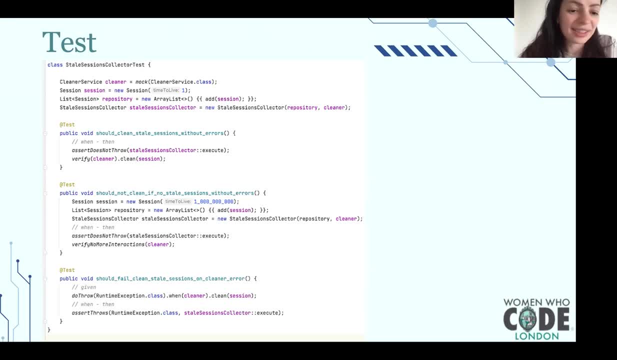 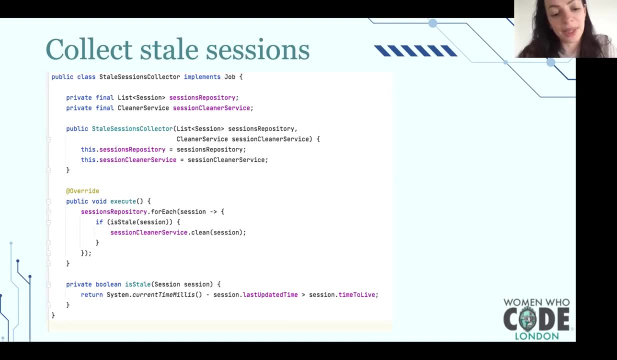 when we come into this test, it's already expired, it's already stay. it's already expired, it's already stay. it's already expired, it's already stay. yeah, because we do this method here. yeah, because we do this method here. yeah, because we do this method here in this private boolean is stale method. 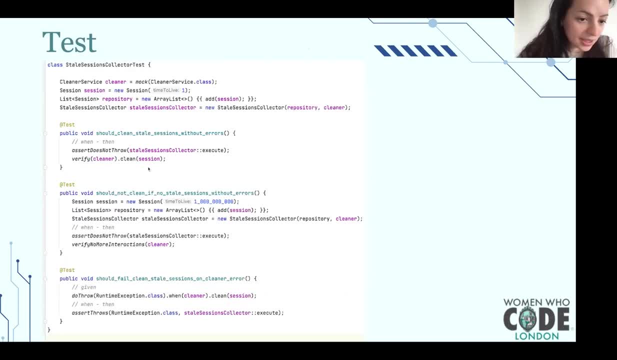 in this private boolean is stale method. in this private boolean is stale method. okay, so, okay so, okay. so we looked at the first test. we just, we looked at the first test. we just, we looked at the first test. we just checked that everything is worse, checked that everything is worse. 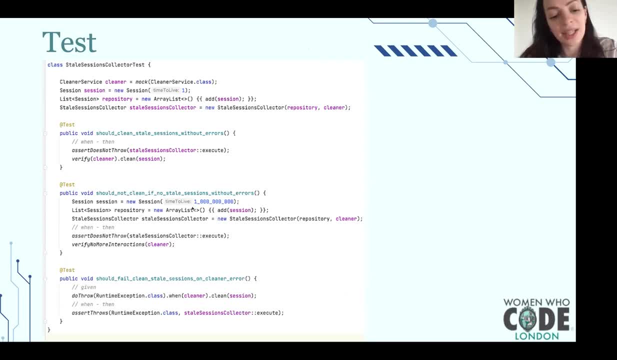 checked that everything is worse. then we look at the second test now we. then we look at the second test, now we. then we look at the second test, now we have to say, have to say, have to say, you know, there will be session with very, you know there will be session with very. 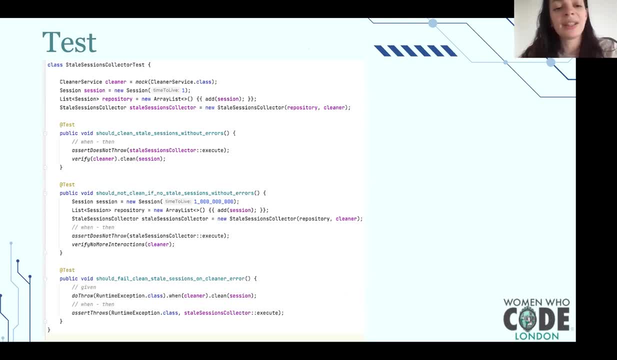 you know, there will be session with very long time to live, long time to live, long time to live. so, when we will try, when we will try to so, when we will try, when we will try to so, when we will try, when we will try to collect this session, 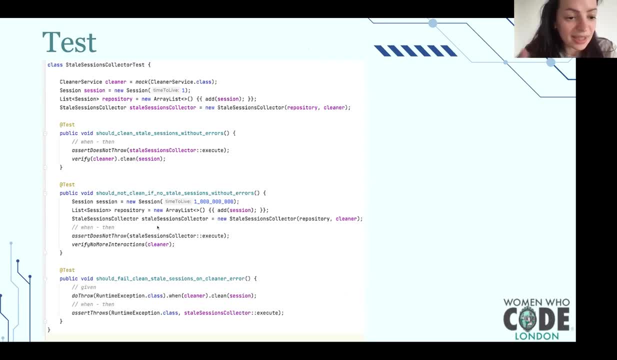 collect this session, collect this session. it won't be collected. so it won't be collected, so it won't be collected. so, at the second test, at the second test, at the second test, we just verify that there was, we just verify that there was, we just verify that there was no iteration with the object cleaner. 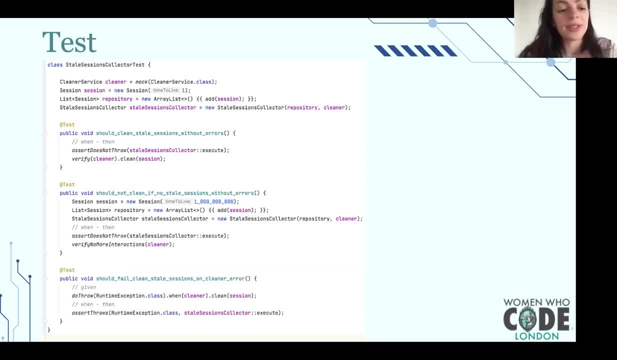 no iteration with the object cleaner. no iteration with the object cleaner. and yeah, that's it, and yeah, that's it, and yeah, that's it. we check that there are no years. no, we check that there are no years. no, we check that there are no years, no exceptions. so i say, does it not roll? 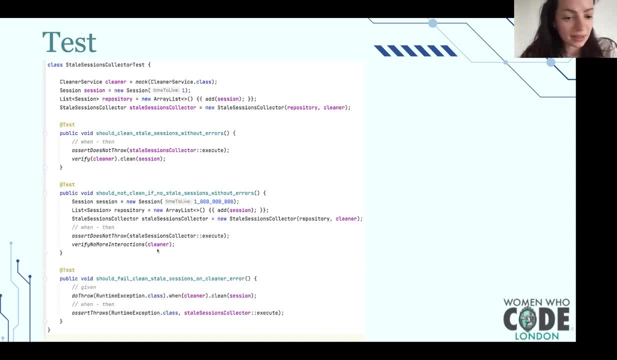 exceptions. so i say: does it not roll exceptions? so i say: does it not roll and verify there are no more interaction and verify there are no more interaction and verify there are no more interaction with, with, with, with our mocked option object, with our mocked option object, with our mocked option object. and at the third test we check that. 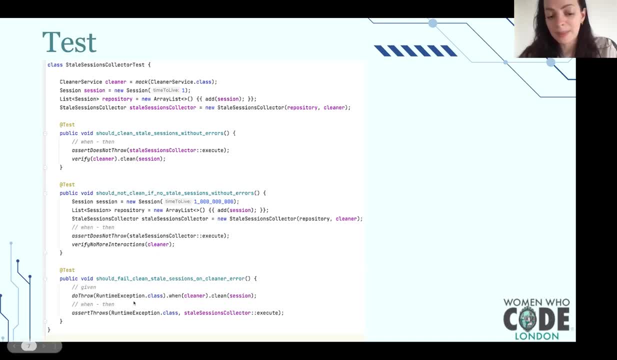 and at the third test, we check that. and at the third test, we check that if our object do throw, if our object do throw, if our object do throw, exception, exception, exception, when, when, when we need to, we need to, we need to check that our method, check that our method. 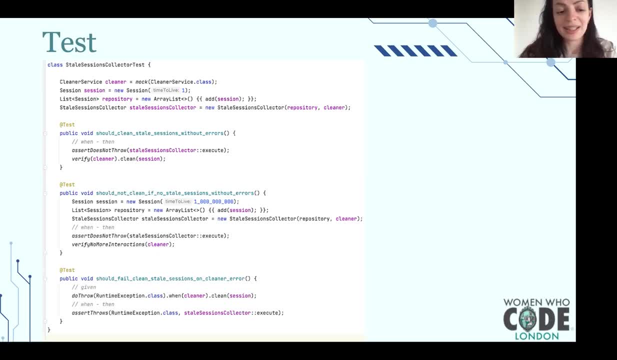 check that our method throw exception, anything that throw exception, anything that throw exception, anything that need to be clarified in this test. please need to be clarified in this test. please need to be clarified in this test. please ask me it's not about object oriented. ask me it's not about object oriented. 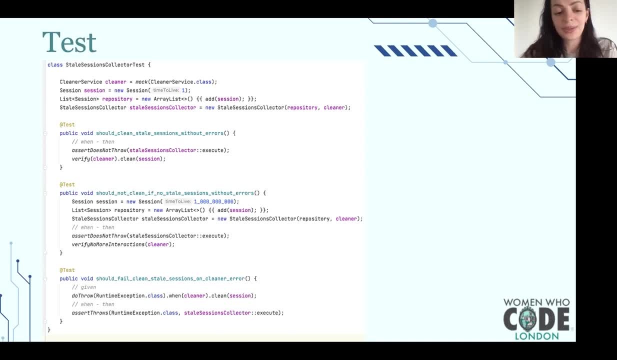 ask me: it's not about object oriented patterns, it's more about patterns. it's more about patterns. it's more about syntax and java and how to write test on syntax and java, and how to write test on syntax and java and how to write test on the function. 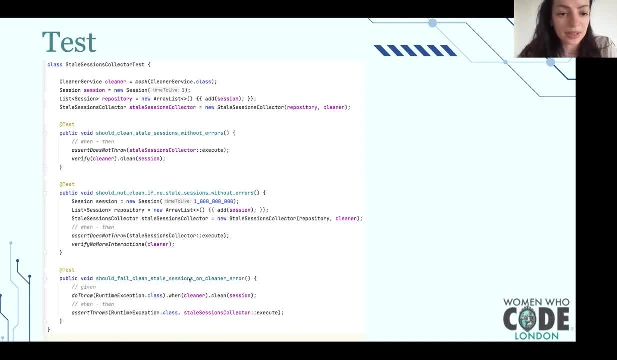 the function, the function. i'm waiting for a bit for a question. i i'm waiting for a bit for a question. i i'm waiting for a bit for a question. i also can also can also can check the chart, but it will be on the. check the chart, but it will be on the. 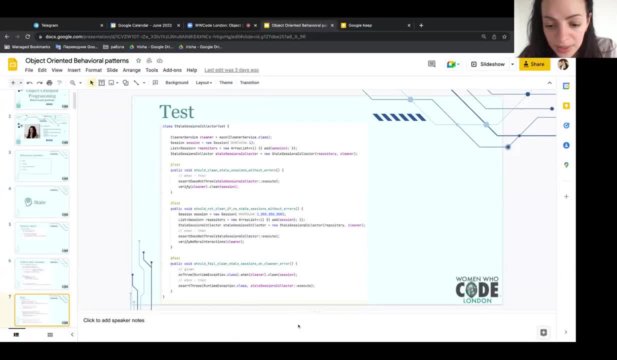 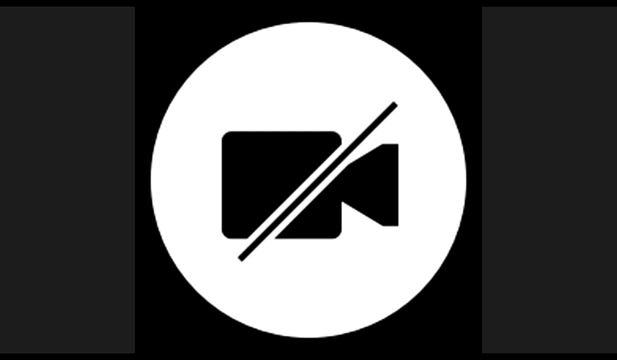 check the chart, but it will be on the same same, same on the same, on the same window, on the same, on the same window, on the same, on the same window, and i also need to check if anyone, and i also need to check if anyone, and i also need to check if anyone unmuted. okay, i see one person is. 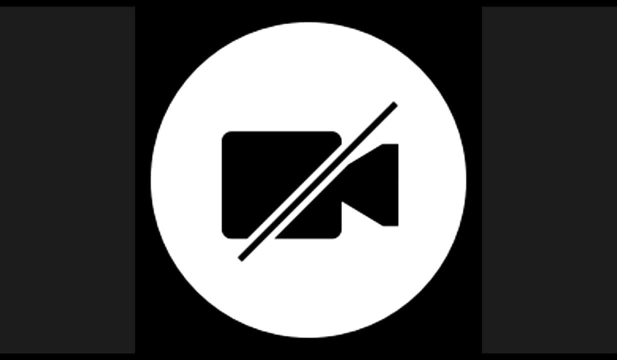 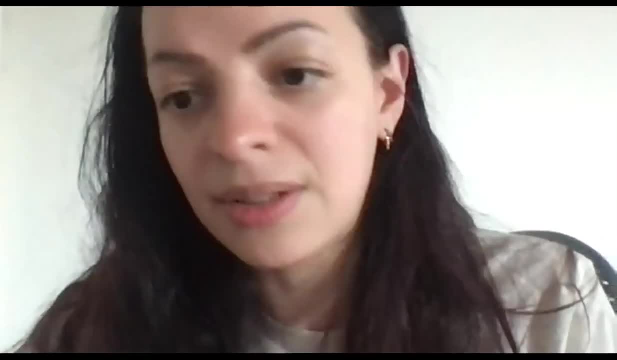 unmuted. okay, i see, one person is unmuted. okay, i see, one person is unmuted. i also have a property. i also have a property. i also have a property. mute participants on entry. mute participants on entry. mute participants on entry. yes, so, yes, so, yes. so i hope i wouldn't have problems with. 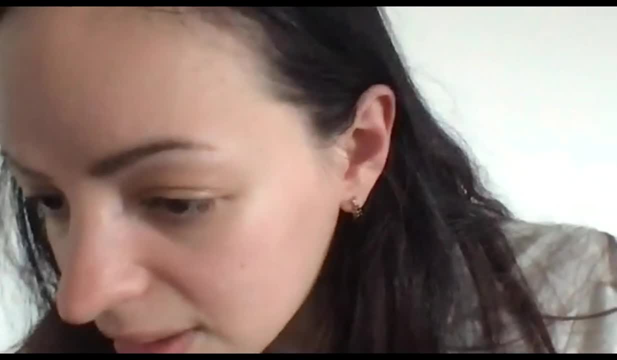 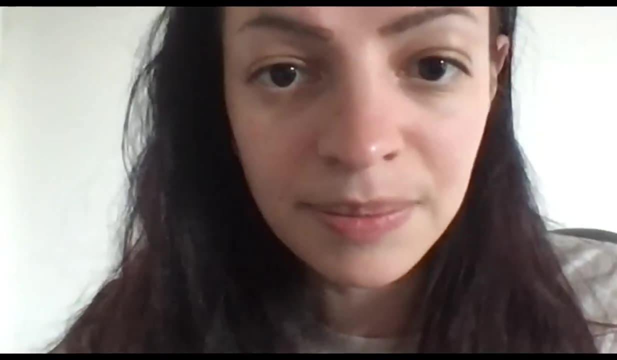 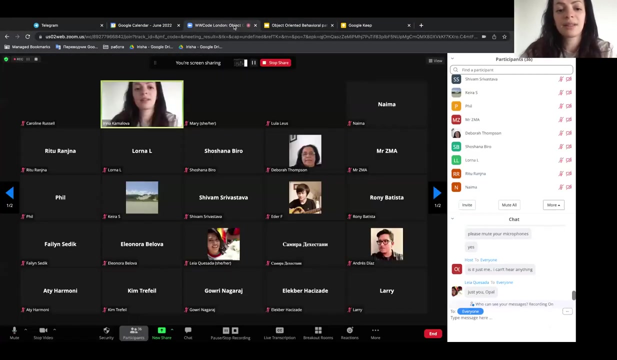 i hope i wouldn't have problems with. i hope i wouldn't have problems with background noise, background noise, background noise, and and and. okay, i don't see any questions so far. okay, i don't see any questions so far. okay, i don't see any questions so far. so i continue this presentation. 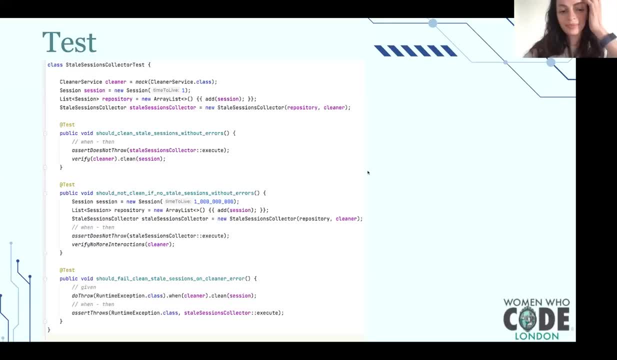 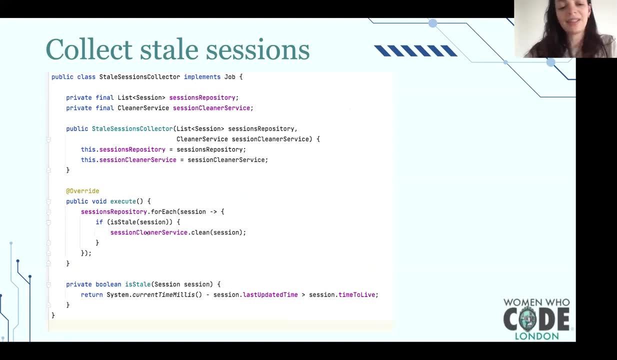 yeah, you see it. yeah, you see it. yeah, you see it. okay, okay, okay, okay, so method was pretty clear. we just okay, so method was pretty clear. we just okay, so method was pretty clear. we just check that session should be collected. check that session should be collected. 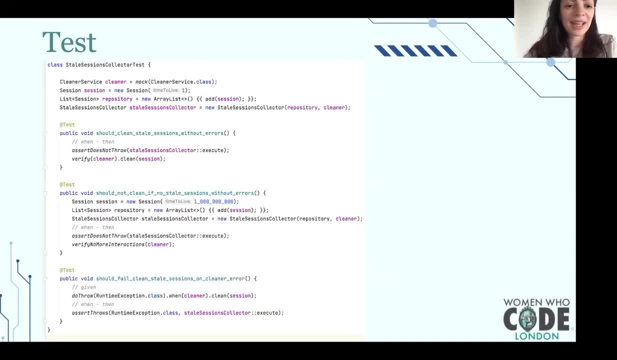 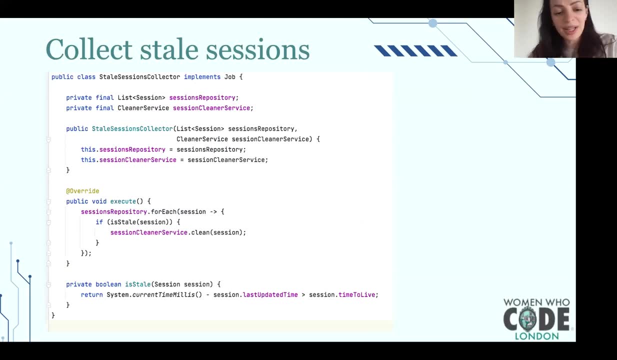 check that session should be collected if it's stable and still in the same. if it's stable and still in the same. if it's stable and still in the same class, class, class now. how do not test session behavior now? how do not test session behavior now? how do not test session behavior? the problem here? is that actually why i? 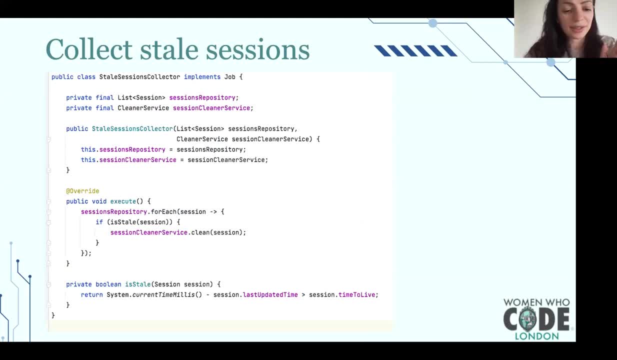 the problem here? is that actually why i the problem here? is that actually why i should also should also should also when. why i should test two methods i when why i should test two methods. i when why i should test two methods. i won't only test one method execute. 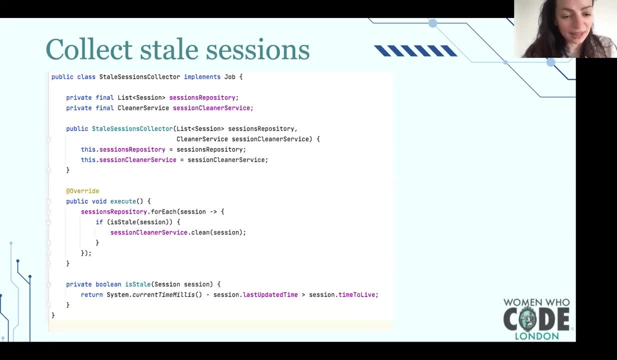 won't only test one method execute, won't only test one method execute, but i need to care about what's. but i need to care about what's, but i need to care about what's happening with stale session happening with stale session, happening with stale session. so i need to provide. 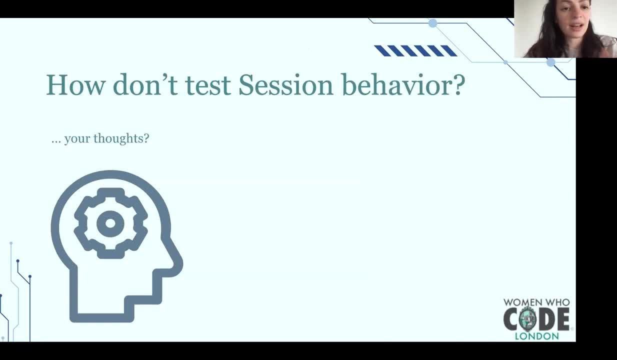 so i need to provide, so i need to provide exactly stale sessions, exactly stale sessions, exactly stale sessions. how, what can i do? how, what can i do? how, what can i do to avoid testing this session behavior, to avoid testing this session behavior, to avoid testing this session behavior? and what is your thoughts? 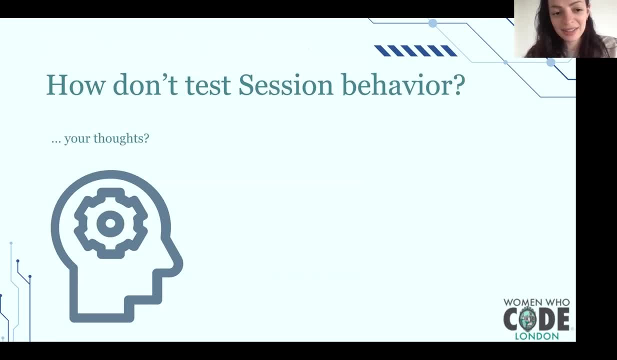 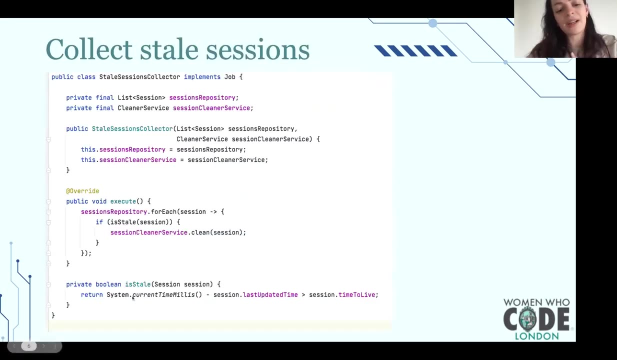 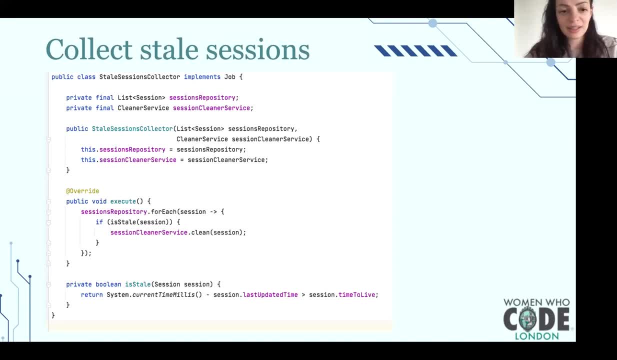 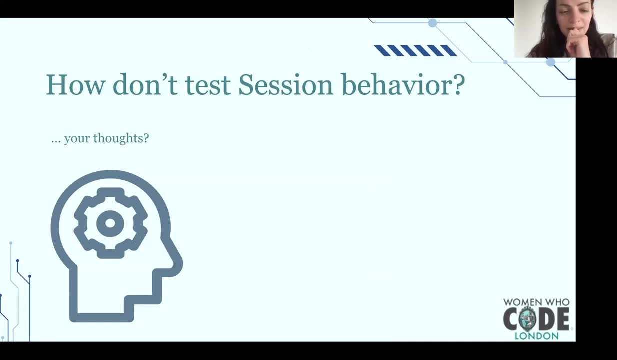 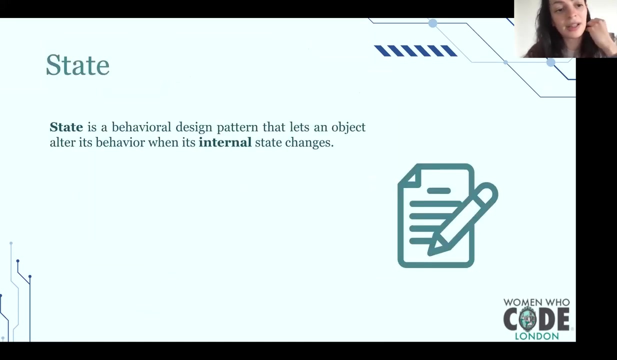 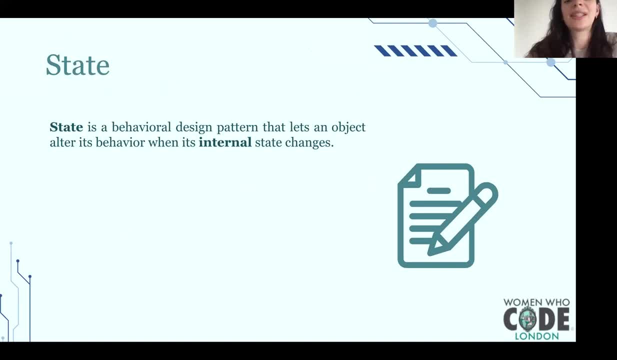 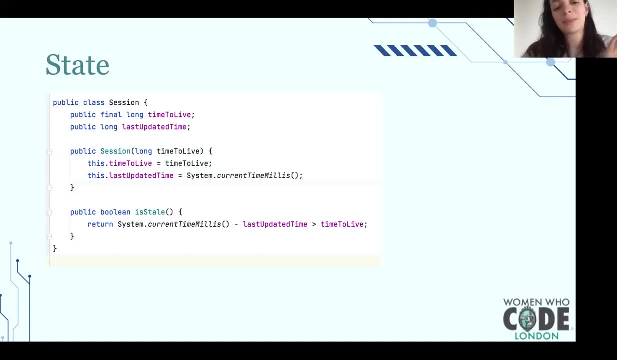 lets an object. lets an object alter its behavior, when its internal alter its behavior, when its internal alter its behavior, when its internal state changes, state changes, state changes. so actually, honestly, so, actually, honestly, so, actually honestly, i won't just have some property that, i won't just have some property that. 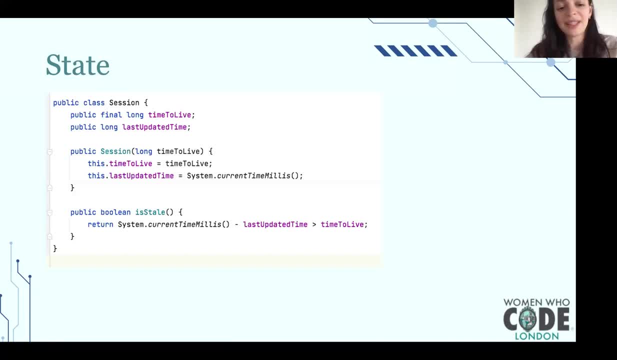 i won't just have some property. that session is stale. instead of putting this session is stale. instead of putting this session is stale. instead of putting this method, method, method into stale collector class because it's into stale collector class. because it's into stale collector class because it's collector. 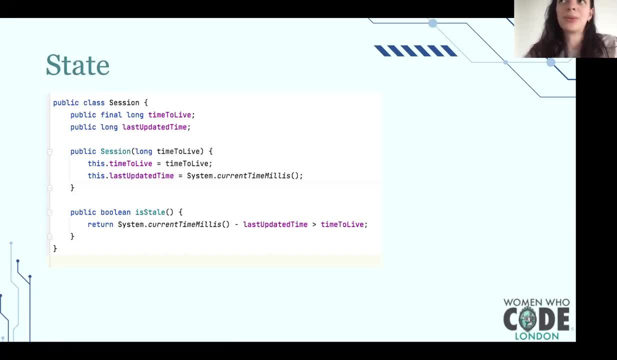 collector, collector, and i don't want to put their logic and i don't want to put their logic and i don't want to put their logic about, about, about. how state is how session, how state is how session, how state is how session, how session behavior is implemented. 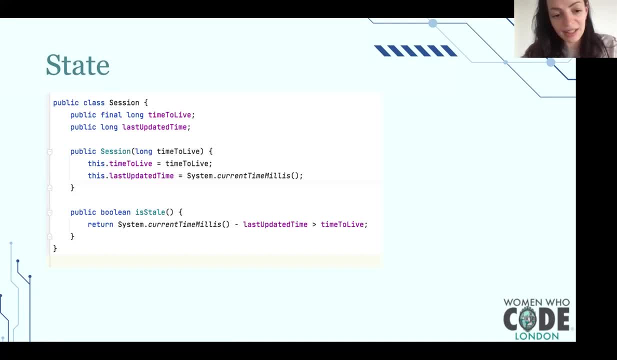 how session, how session behavior is implemented, how session, how session behavior is implemented actually, actually, actually the thing that state is stale. the thing that state is stale, the thing that state is stale when this condition, that, when this condition, that, when this condition, that current time is more than difference. 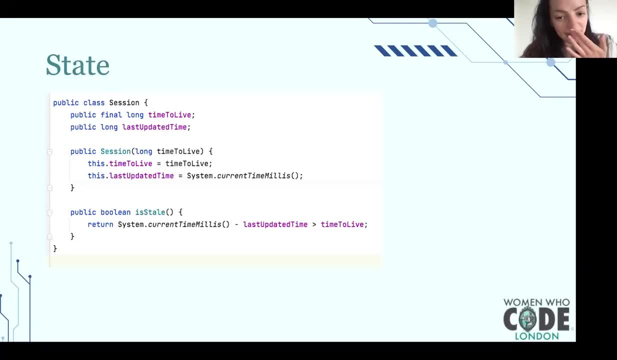 current time is more than difference. current time is more than difference between between between last update time, last update time, last update time and time to leave, and time to leave and time to leave. so so so i just put it in session class for now. i just put it in session class for now. 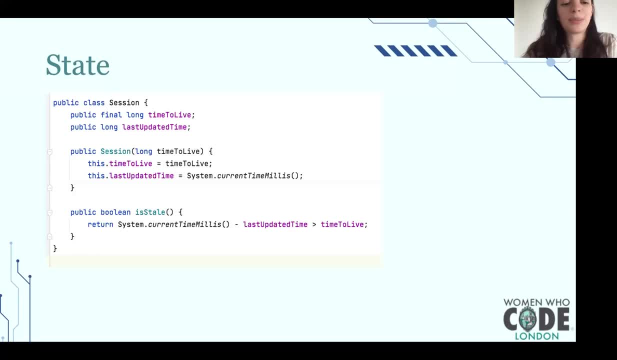 i just put it in session class for now and that's already, and that's already and that's already like the first step. to like the first step, to like the first step to state pattern where i say you know state pattern, where i say you know state pattern, where i say you know session have. 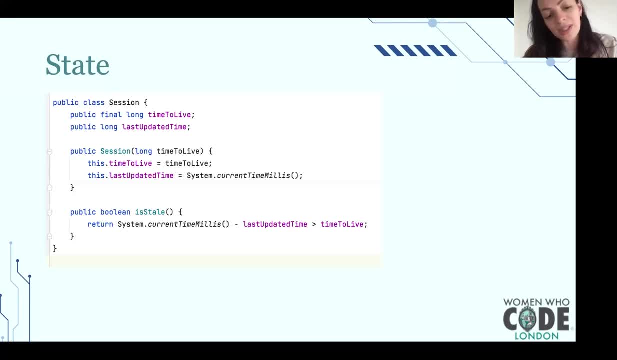 session have session have its own state and if its own state, its own state, its own state is stale, i can check it directly from: is stale. i can check it directly from: is stale. i can check it directly from state and directly from session. state and directly from session. 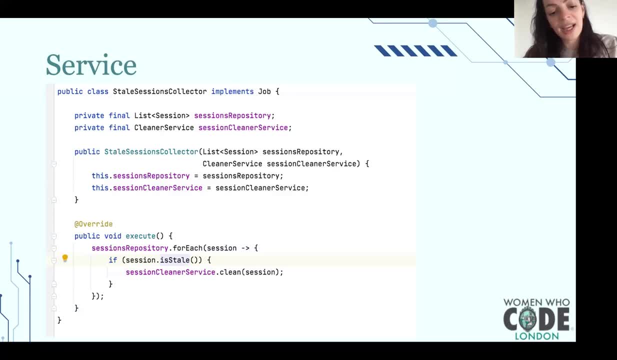 state and directly from session, and in this case, i just drop this method. and in this case, i just drop this method. and in this case, i just drop this method and i already have this session object and i already have this session object and i already have this session object as a parameter. 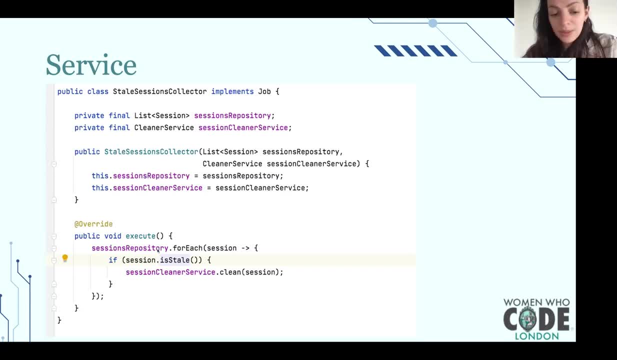 as a parameter. as a parameter, so i just get this session object from. so i just get this session object from. so i just get this session object from repository, repository, repository, and if it's stale i clean it, and that's. and if it's stale i clean it and that's. 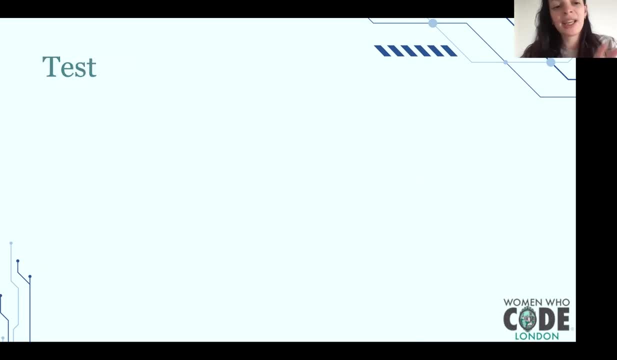 and if it's stale, i clean it and that's it. it. it, my service becoming lighter, my service becoming lighter, my service becoming lighter. and now i have first of all test the, and now i have first of all test the, and now i have first of all test the session. object: 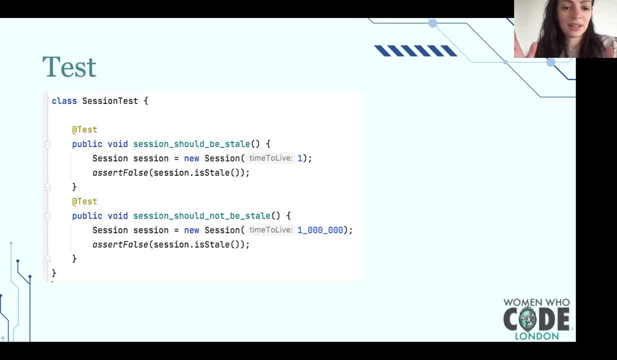 session object: session object. now i say you know i can have just now. i say you know i can have just now. i say you know i can have just sessions that i created, sessions that i created, sessions that i created, uh, some one mile seconds ago and right. 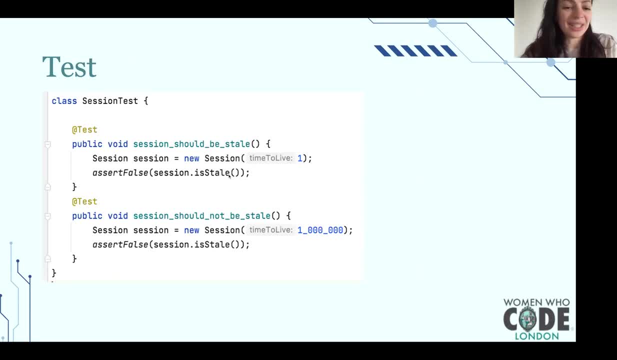 uh, some one mile seconds ago, and right, uh, some one mile seconds ago, and right now it's now. it's now it's two mile seconds and it's already stale, two mile seconds and it's already stale, two mile seconds and it's already stale. so, yeah, this is basically a third. 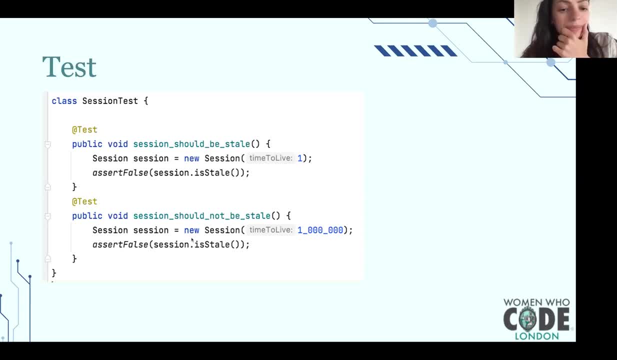 so, yeah, this is basically a third. so, yeah, this is basically a third. true, true, true, and this will, and this will, and this will be a third, false be a third, false, be a third, false, um, um, um. now my test for sure is becoming a bit. now my test for sure is becoming a bit. 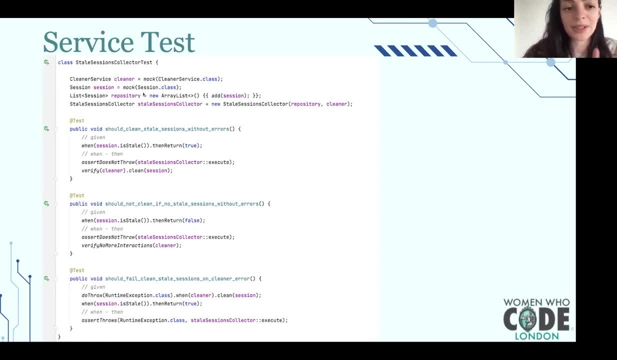 now my test for sure is becoming a bit lighter because i can mock session lighter. because i can mock session lighter, because i can mock session object as well, object as well, object as well. now i can say that. now i can say that. now i can say that if i ask session is it stale, then i 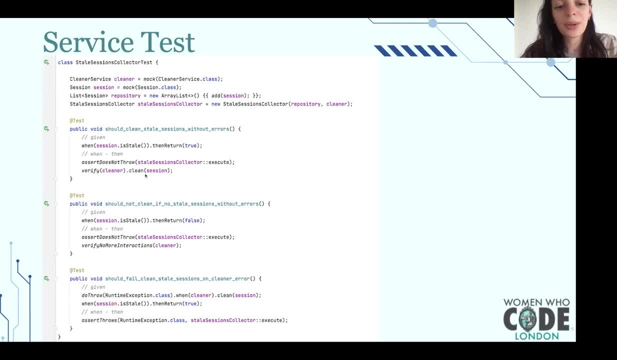 if i ask session is it stale, then i. if i ask session is it stale, then i return true, and in this case my cleaner return true, and in this case my cleaner return true, and in this case my cleaner should clean this session, should clean this session, should clean this session. that's it. 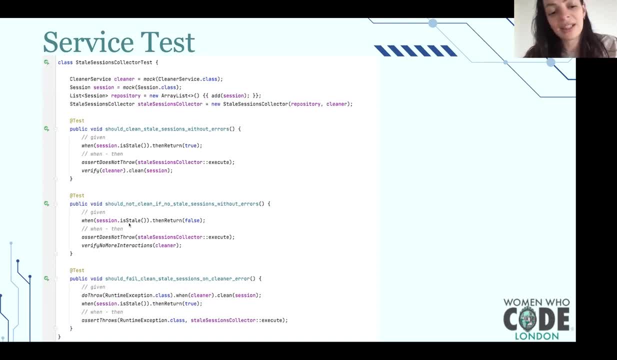 that's it. that's it. and if i say that my session and if i say that my session and if i say that my session on the question, if it is stale on the question, if it is stale on the question, if it is stale returning false, it's not stale. 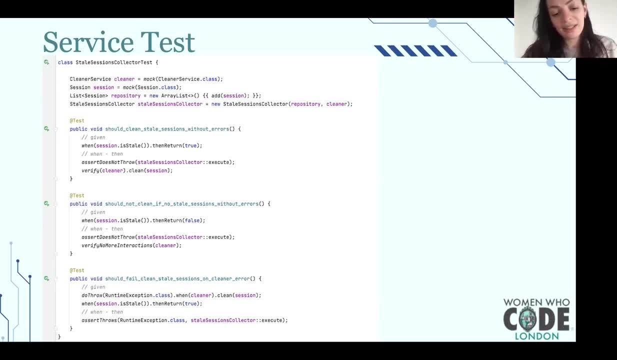 returning false: it's not stale. returning false: it's not stale. i verify that there were no cleaning. i verify that there were no cleaning. i verify that there were no cleaning. yeah, and the third one is just the same. yeah, and the third one is just the same. 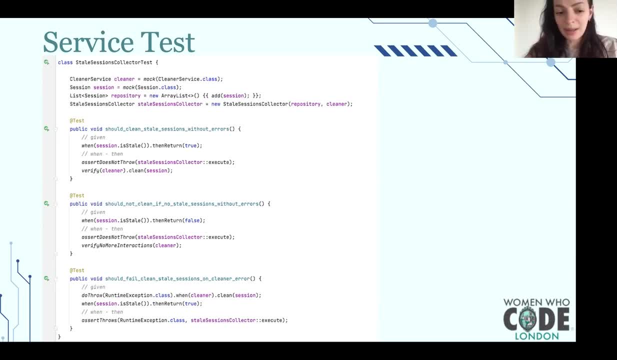 yeah, and the third one is just the same, so, so so it's like the first step to understand. it's like the first step to understand. it's like the first step to understand why it's could be interesting to check, why it's could be interesting to check. 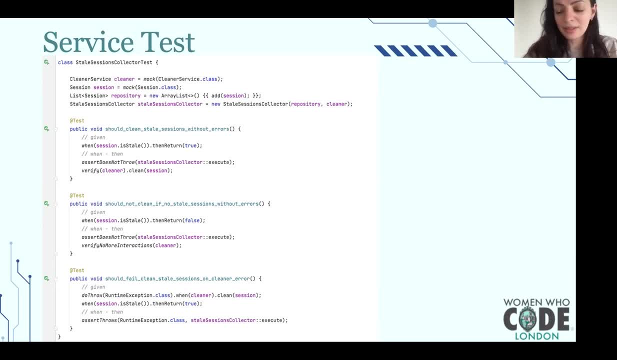 why it's could be interesting to check session state, this session state, this session state, this state pattern, state pattern, state pattern, and and and let's think that session action, let's think that session action, let's think that session action actually more complex object, actually more complex object. 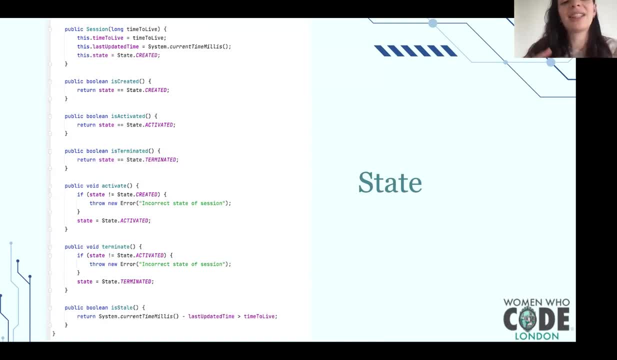 actually more complex object and it's also have several states and it's also have several states and it's also have several states. session can be created. session can be. session can be created. session can be. session can be created. session can be activated- activated. activated session can be terminated. 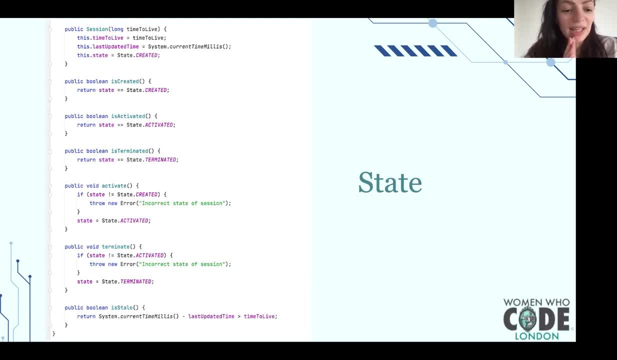 session can be terminated. session can be terminated. session, session, session. if, for example, now i can say if session. if, for example, now i can say if session. if, for example, now i can say if session is stale, is stale, is stale, she, she, she session, session, session coming in the state of terminated. 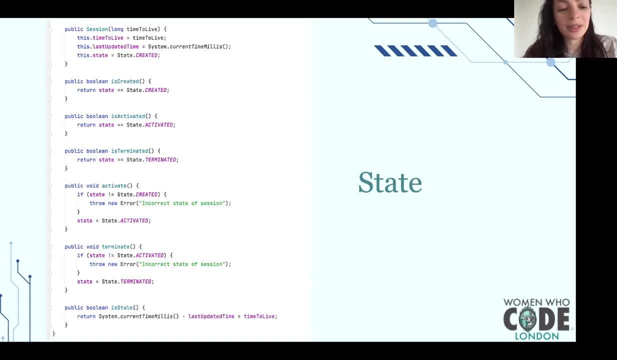 coming in the state of terminated, coming in the state of terminated and the cleaner and the cleaner and the cleaner could also, could also, could also terminate session and then terminate session and then terminate session and then then clean it from repository, then clean it from repository, then clean it from repository to mark it terminated, for example, and 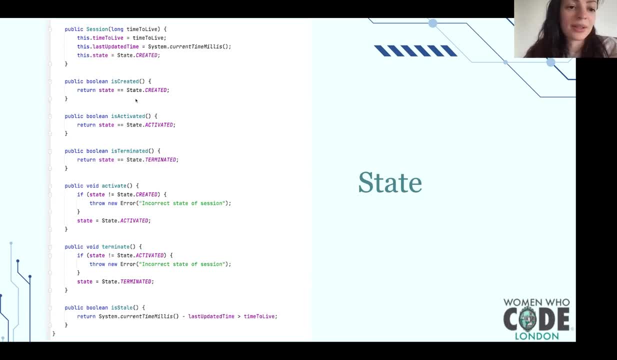 to mark it terminated, for example. and to mark it terminated, for example, and save, save, save. so you see we can create several methods. so you see we can create several methods. so you see we can create several methods depending on the state, depending on the state, depending on the state, and every time you just check if session. 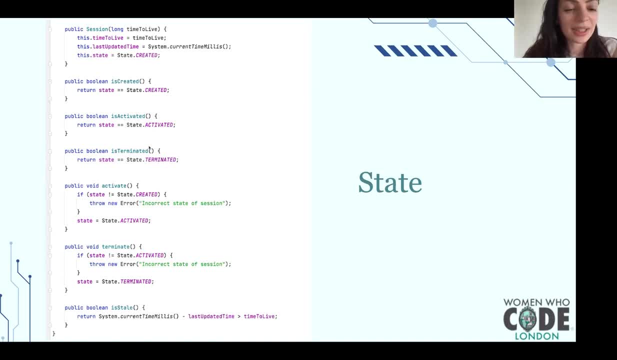 and every time you just check if session. and every time you just check if session is created or if session is activated is created, or if session is activated is created, or if session is activated, or if session is terminated, or if session is terminated or if session is terminated, and you just 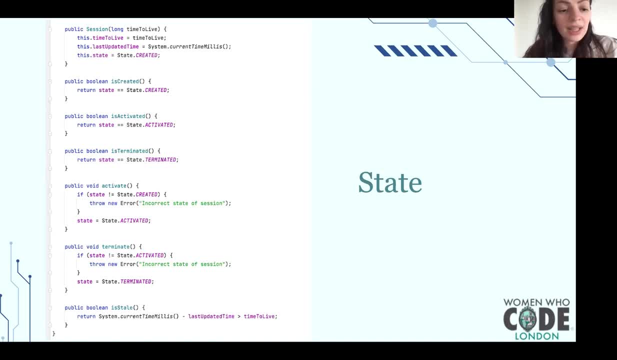 and you just, and you just, check, check, check this. you just, you just check this this, you just, you just check this this. you just, you just check this and it's very powerful, like you don't- and it's very powerful, like you don't- and it's very powerful like you don't need actually to know. 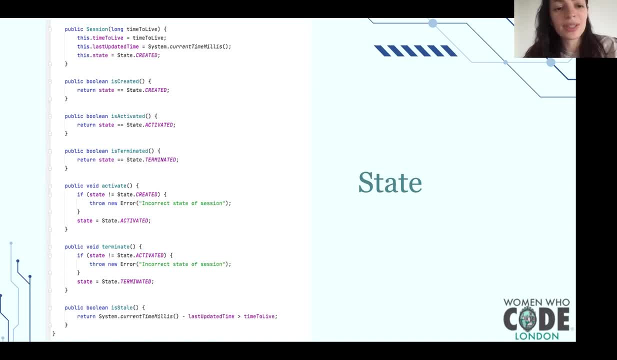 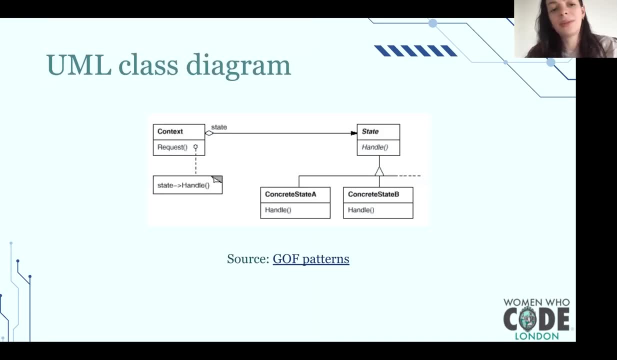 need actually to know, need actually to know what internal things sorry for the, what internal things sorry for the? what internal things sorry for the background noise, background noise, background noise. you don't need to check internal things, you don't need to check internal things. you don't need to check internal things. uh, so if we would see, if we would. 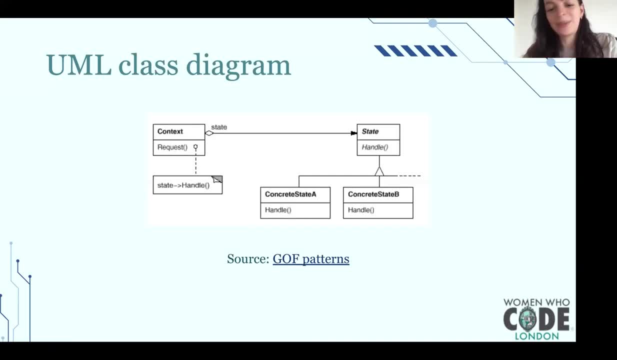 uh. so if we would see, if we would uh. so if we would see, if we would go to golf patterns official website. go to golf patterns official website. go to golf patterns official website. we will see a durable diagram there. we will see a durable diagram there. we will see a durable diagram there which uh. 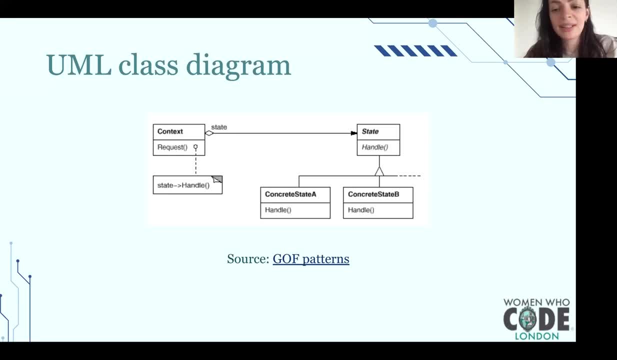 which uh, which uh, how to how to implement this pattern. how to, how to how to implement this pattern, how to how to how to implement this pattern. state, state, state. so they say that basically status class. so they say that basically status class. so they say that basically status class, and you have several implementations. 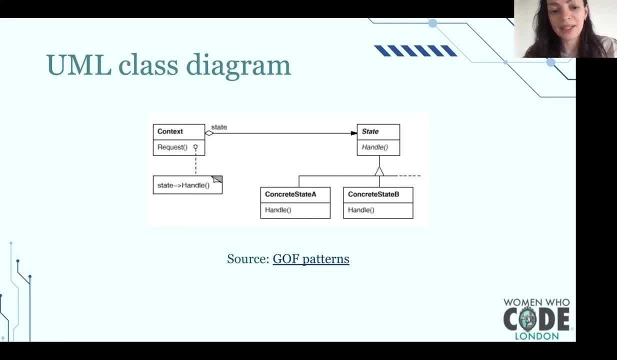 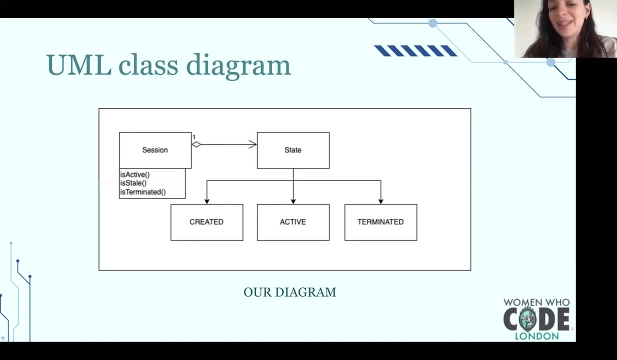 and you have several implementations, and you have several implementations, and, and, and. you can have also handle as a method in our example. i am using, in our example, i am using. in our example, i am using. i'm using enums in java, so they allow me. i'm using enums in java, so they allow me. 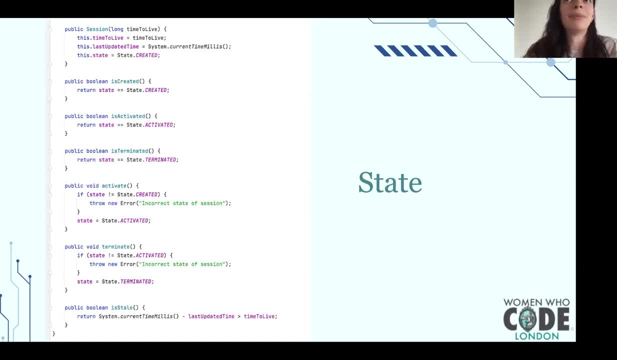 i'm using enums in java, so they allow me to create, to create, to create several, several implementations of the several, several implementations of the several, several implementations of the state of the session, state of the session, state of the session. so, state, basically enough. so state, basically enough. 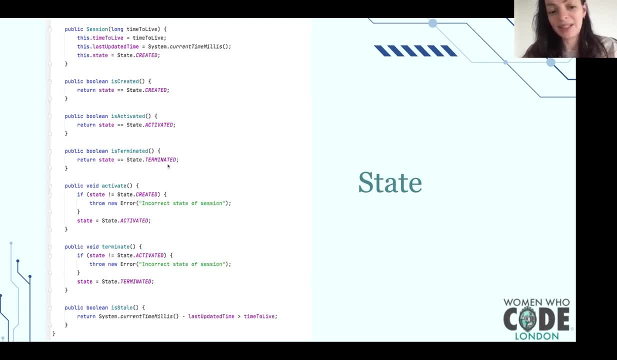 so state basically enough, and implementation is created, activated, and implementation is created, activated, and implementation is created, activated, terminated, terminated, terminated. and if i will draw the same diagram that, and if i will draw the same diagram that, and if i will draw the same diagram that, gov, gov. 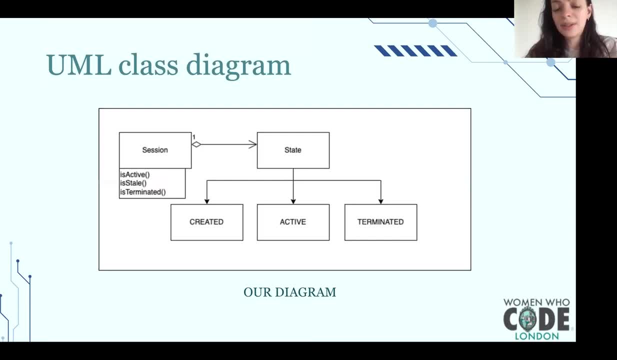 gov. gang of forward roll. gang of forward roll. gang of forward roll. i will say that, okay, my state i have. i will say that, okay, my state i have. i will say that, okay, my state i have. instead in session, i have state. instead in session, i have state. 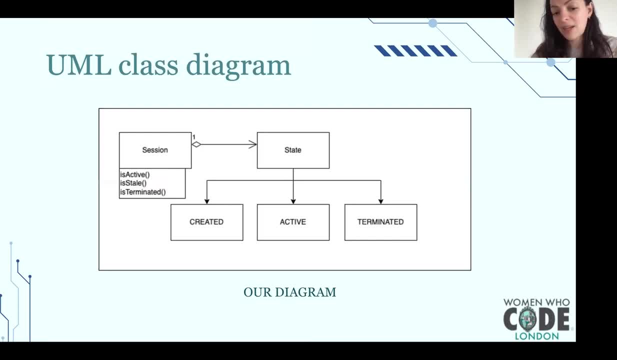 instead in session, i have state: this state, this state, this state have three states, basically it's created. have three states, basically it's created. have three states, basically it's created, activated, activated creative. creative creative created, activated, terminated. created, activated, terminated. created, activated, terminated. i also could use: 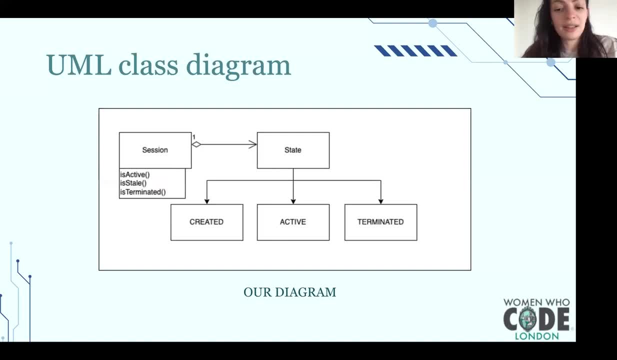 i also could use. i also could use active instead of activated, active instead of activated, active instead of activated, and and and yeah, it makes sense to use active as. yeah, it makes sense to use active as yeah, it makes sense to use active as well. well, well, and i can ask. session, uh, session. 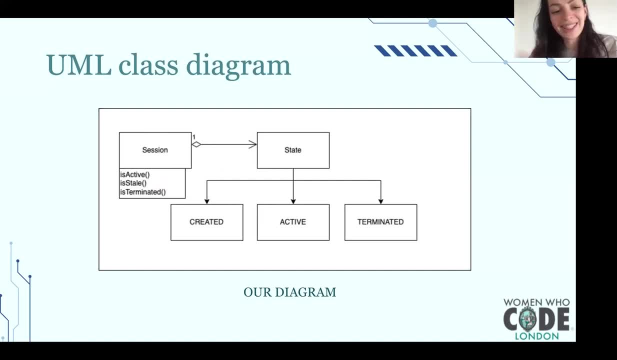 and i can ask session uh session and i can ask session uh session. are you active? are you stale? are you are you active? are you stale? are you are you active? are you stale? are you terminated? are you created like and terminated? are you created like and terminated? are you created like and session have just methods. it's active is. 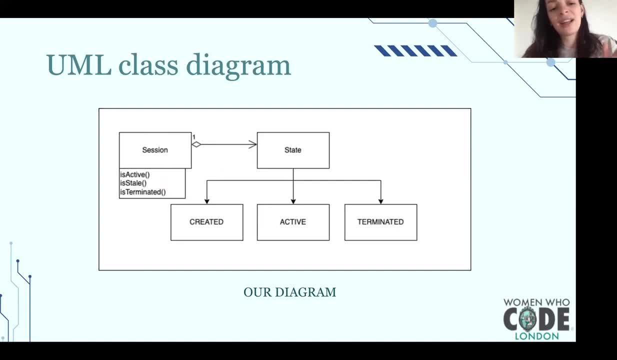 session: have just methods. it's active is session: have just methods. it's active is: state tail is terminated is created. state tail is terminated is created. state tail is terminated is created. uh, maybe i don't need is created because. uh, maybe i don't need is created because. 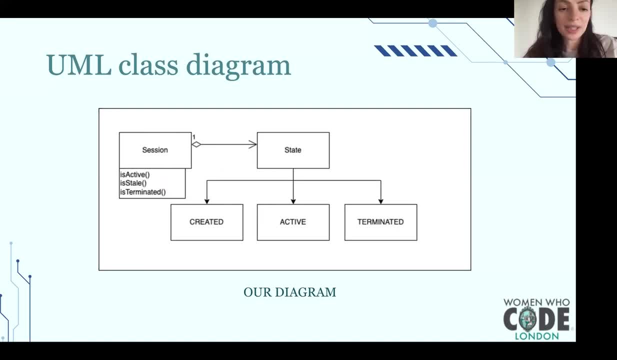 uh, maybe i don't need is created because this is like the first. this is like the first. this is like the first, the first state of the session. so here is the first state of the session. so here is the first state of the session. so here is. you can be flexible. 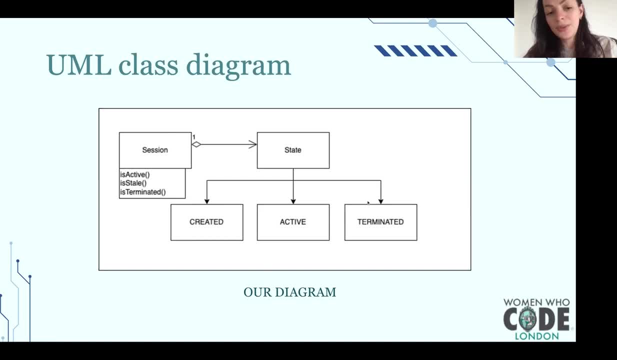 you can be flexible. you can be flexible, but the most idea of this state that you, but the most idea of this state that you, but the most idea of this state that you say object has has some state say object has has some state say object has has some state yeah, and 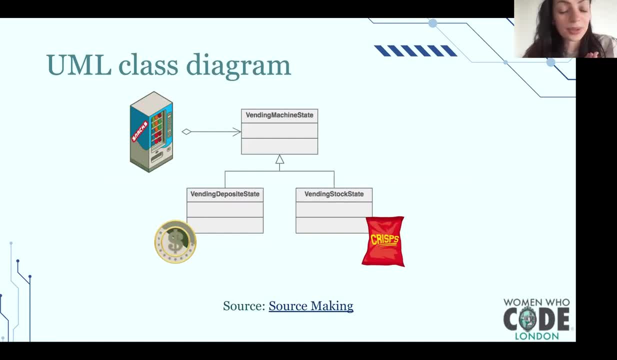 yeah and yeah, and here i put more here, i put more here, i put more links for resources, links for resources, links for resources, and this state basically it's, and this state basically it's, and this state basically it's: uh, it's applying in software design, uh, it's applying in software design. 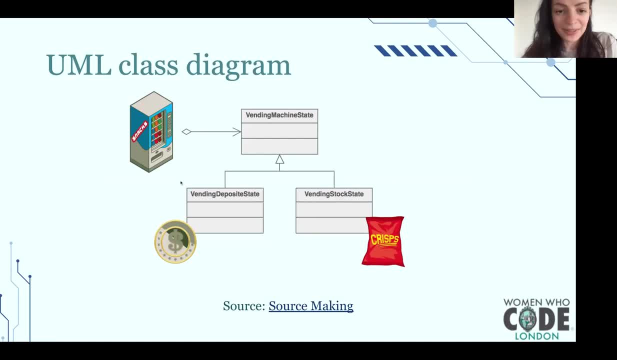 uh, it's applying in software design everywhere, everywhere, everywhere. suppose you have vending machine with. suppose you have vending machine with. suppose you have vending machine with snacks, snacks, snacks, and you can say that your vending machine and you can say that your vending machine and you can say that your vending machine state is vending deposit state. 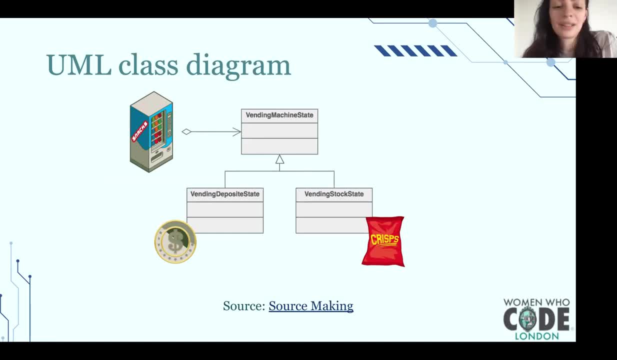 state is vending deposit state, state is vending deposit state and vending stock state. so in vending and vending stock state. so in vending and vending stock state. so in vending deposit state you put money there. deposit state you put money there. deposit state you put money there. and in stock state you're just waiting. 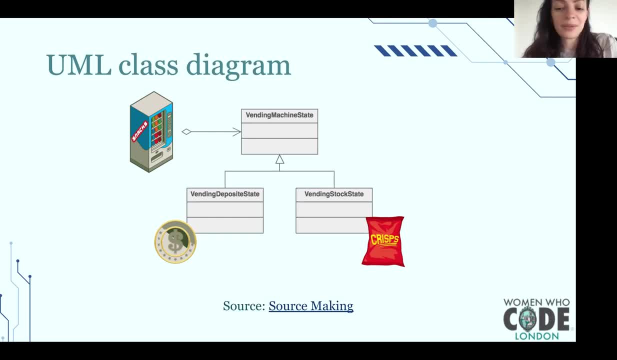 and in stock state you're just waiting and in stock state you're just waiting for someone put money there, for someone put money there, for someone put money there and you gave crisps, for example, and you gave crisps, for example, and you gave crisps, for example. i also added the source. so after this: 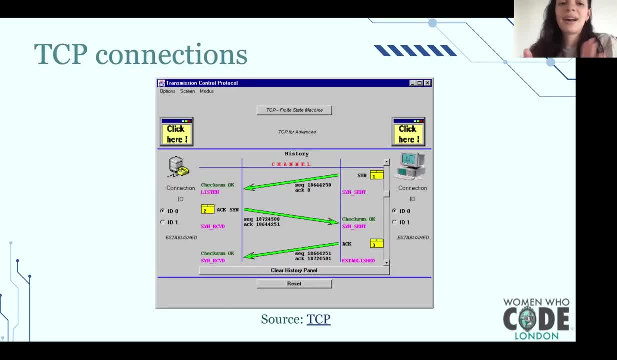 i also added the source. so after this, i also added the source. so after this presentation, you can check this example presentation. you can check this example presentation. you can check this example as well. as well as well: tcp connections, tcp sessions, tcp connections, tcp sessions, tcp connections, tcp sessions. so it also has several states and it's. 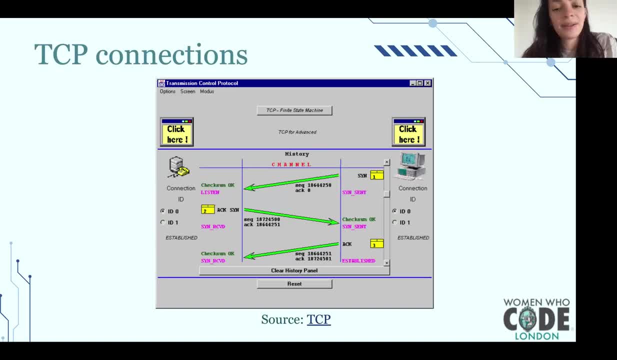 so it also has several states and it's so it also has several states and it's very easy to describe these states, very easy to describe these states, very easy to describe these states, this state pattern, this state pattern, this state pattern. so, if you would like, on actually states of 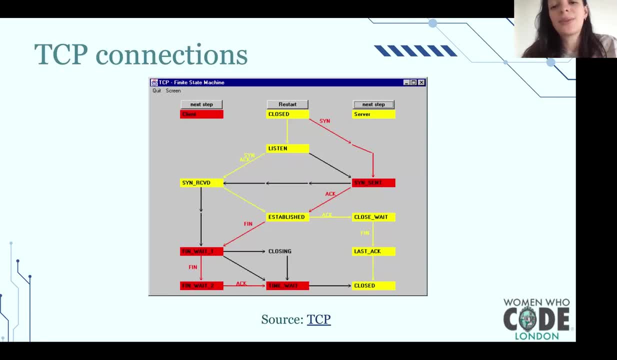 so, if you would like, on actually states of so, if you would like, on actually states of tcp, tcp connection, connection, connection. it's different states for client and it's different states for client and it's different states for client and server, server server. some of them are the same, but you can say: 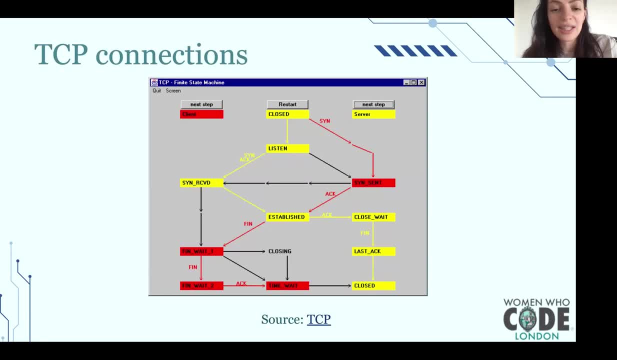 some of them are the same, but you can say some of them are the same, but you can say that you have that, you have that you have all these states as implementation of all these states, as implementation of all these states, as implementation of tcp connection state. tcp connection state. 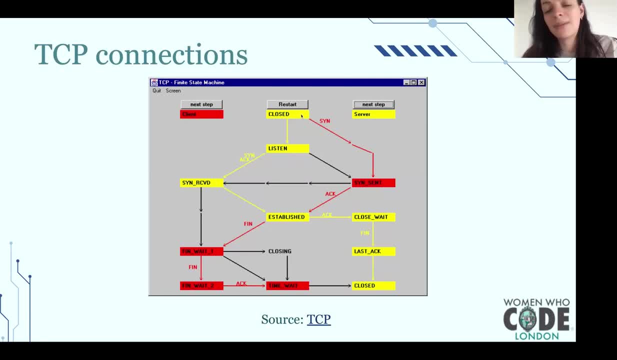 tcp connection state in java. they all could be in java. they all could be in java. they all could be. you know in our variables, you know in our variables, you know in our variables it's very easy to use enums but the. it's very easy to use enums but the. 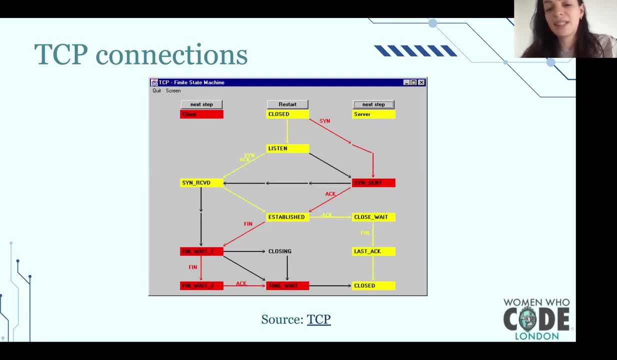 it's very easy to use enums, but the idea, idea, idea, like you use them as a state, like you use them as a state, like you use them as a state of your object- in this case, tcp connection of your object, in this case, tcp connection of your object. in this case, tcp connection state. 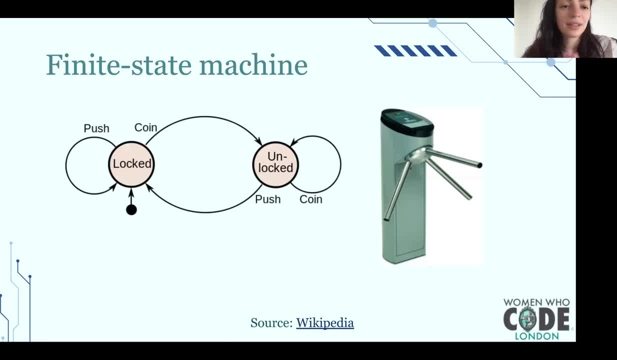 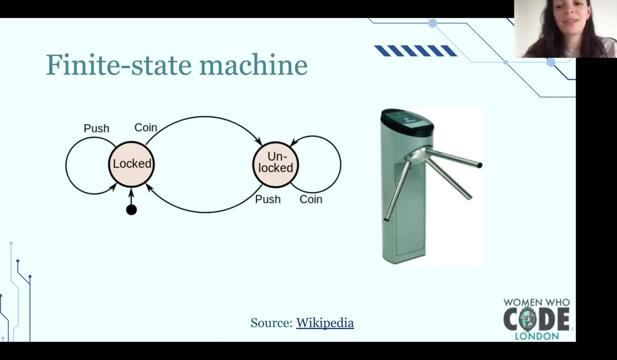 design software, design software, and the idea is you have states for, and the idea is you have states for, and the idea is you have states, for example, you have example, you have example, you have this, this, this beauty, this beauty, this beauty, beautiful, truly, cat, where you can. 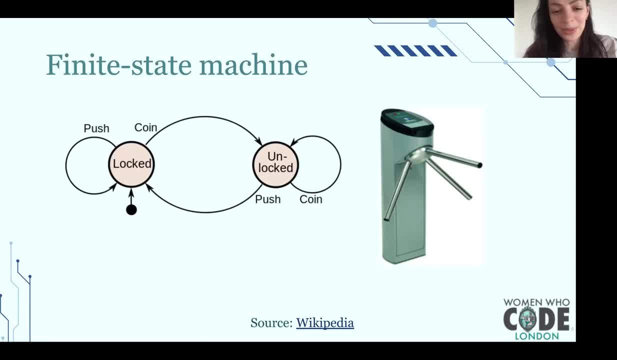 beautiful, truly cat where you can, beautiful, truly cat where you can. you know that if you put the card like, you know that if you put the card like, you know that if you put the card like in the modern world, we just put the card in the modern world, we just put the card. 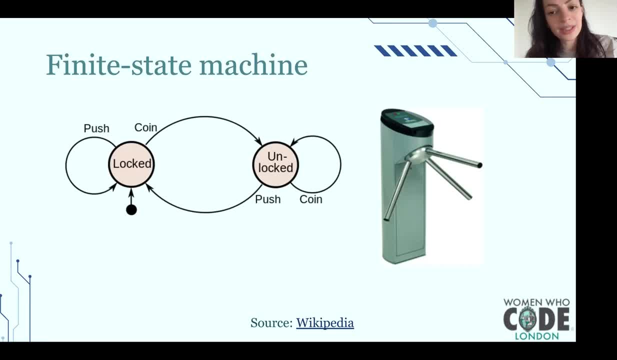 in the modern world, we just put the card and it's unlocked, but, and it's unlocked, but and it's unlocked, but it, it always it, it always it, it always locked, locked, locked. it has basically two states, it has basically two states, it has basically two states, and 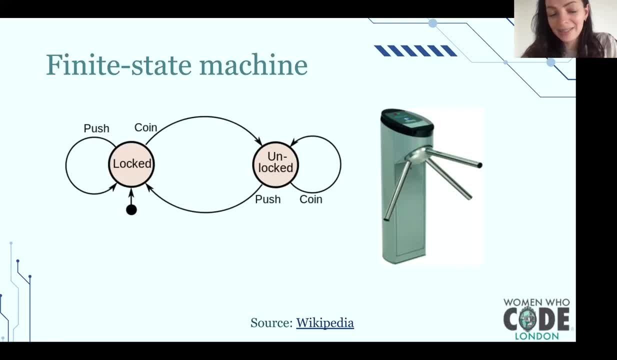 and and in previous ages we put coins there. in previous ages we put coins there. in previous ages we put coins there. that's why in the example on wikipedia, that's why in the example on wikipedia, that's why in the example on wikipedia you can find them and check and they have. 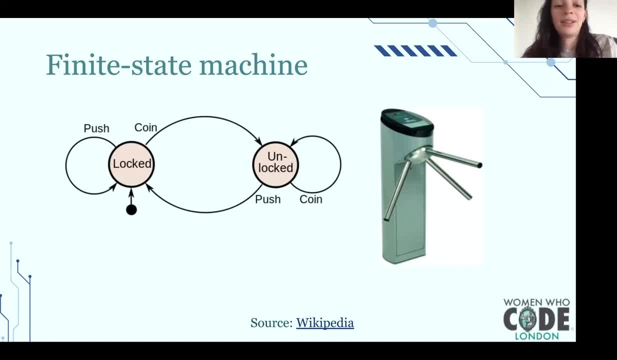 you can find them and check and they have. you can find them and check and they have coins. so you put coin coins. so you put coin coins, so you put coin and this becoming in the state unlocked and this becoming in the state unlocked and this becoming in the state unlocked. and when you push this 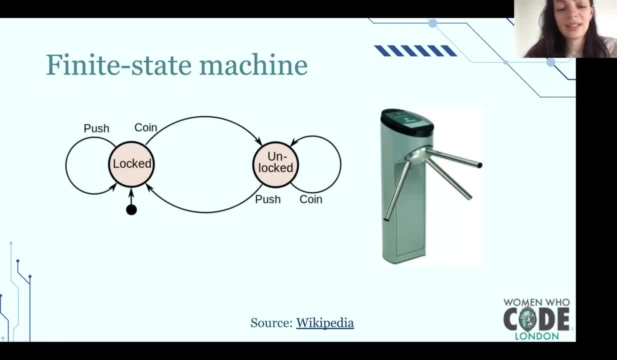 and when you push this and when you push this, and it's coming to the state, locked again, and it's coming to the state, locked again, and it's coming to the state locked again. so only two states, so only two states, so only two states, and and. 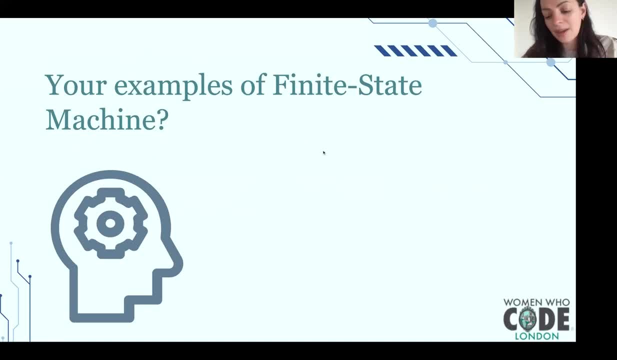 and why finit yeah? why finit yeah? why finit yeah? because we have finit number of states, because we have finit number of states, because we have finit number of states. so so, so would you, would you would you able to share example that you think? 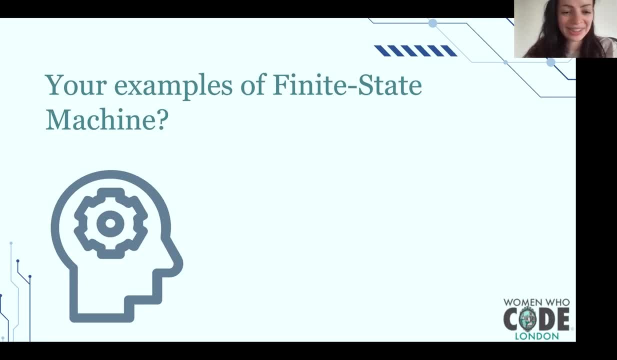 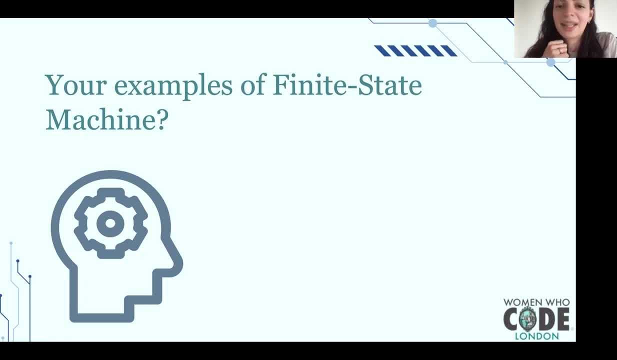 also, also, also, also, also, fit, fit, fit, because you have several states, and this is because you have several states, and this is because you have several states, and this is finit number of states. hello, any ideas? what else could be the state? okay, we will, we will left it as a, as a. 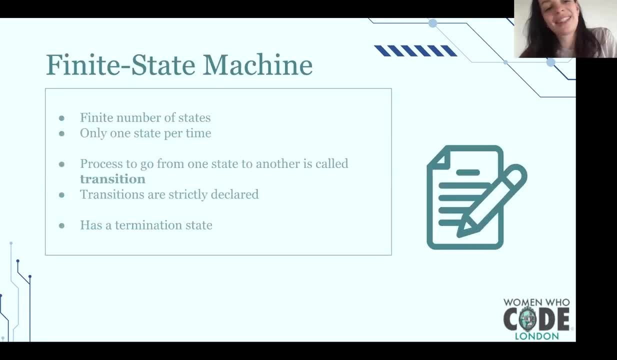 okay, we will. we will left it as a as a. okay, we will. we will left it as a as a small homework for research. small homework for research. small homework for research. uh, some properties of finite state. uh, some properties of finite state. uh, some properties of finite state machine. 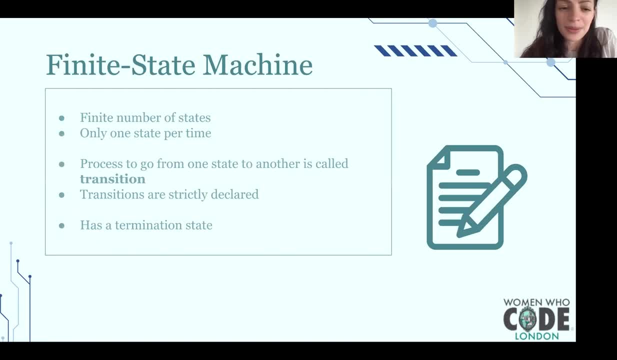 machine, machine. finite number of states. only one state per finite number of states. only one state per finite number of states. only one state per time. like your object can't exist in two time. like your object can't exist in two time. like your object can't exist in two states per time. 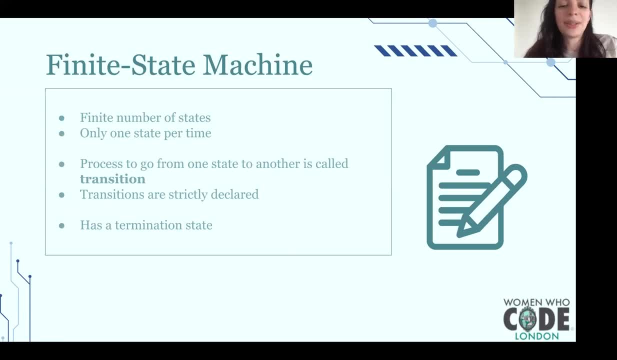 states per time. states per time- uh process to go from one state to uh process, to go from one state to uh process, to go from one state to another is called transition, another is called transition, another is called transition. so you can say: you know my model in. 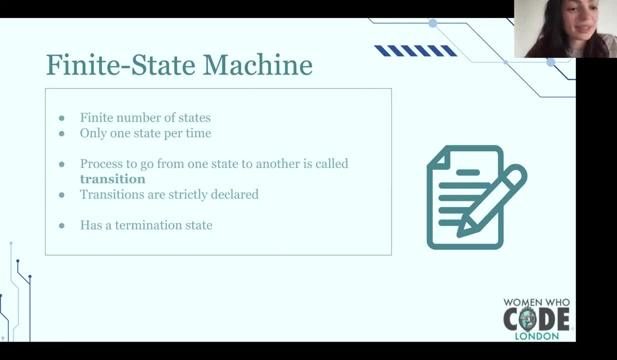 so you can say: you know my model in, so you can say you know my model in this state, this state, this state, then the transition is happening and my then the transition is happening and my then the transition is happening and my model becoming in this state, then the transition is happening and my model becoming in this state. 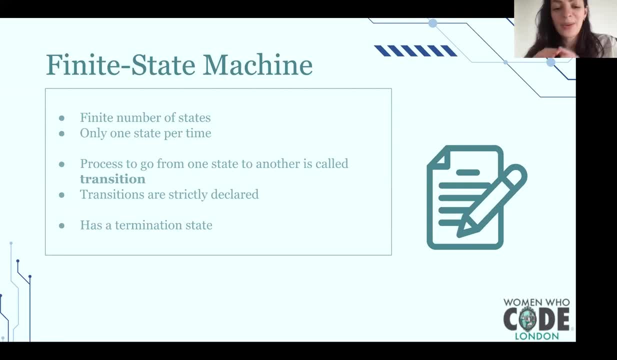 then the transition is happening and my model becoming in this state, strictly declared, so you can say that strictly declared, so you can say that strictly declared, so you can say that you go from, you, go from, you go from this state to another state and only in this state. to another state and only in. 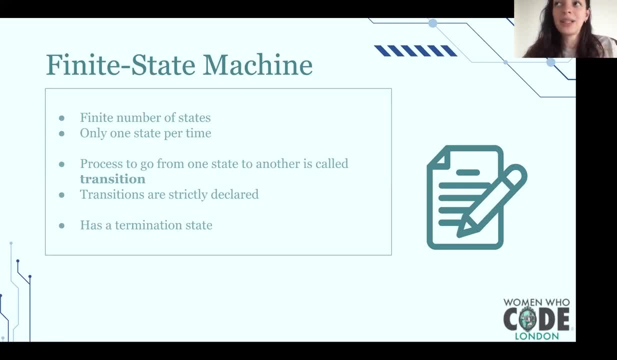 this state to another state and only in this way, this way, this way, for example, you go from created to active, for example, you go from created to active. for example, you go from created to active, and and and from active to terminate it, but you can go from active to terminate it, but you can go. 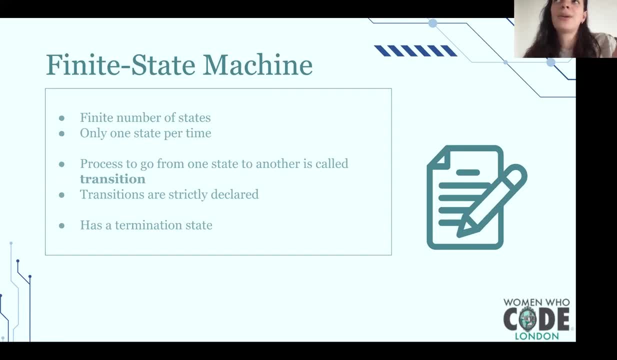 from active to terminate it. but you can go from created to terminate it, from created to terminate it, from created to terminate it. or okay, that could be, or okay that could be, or okay that could be. but you can go from active to create it's, but you can go from active to create it's. 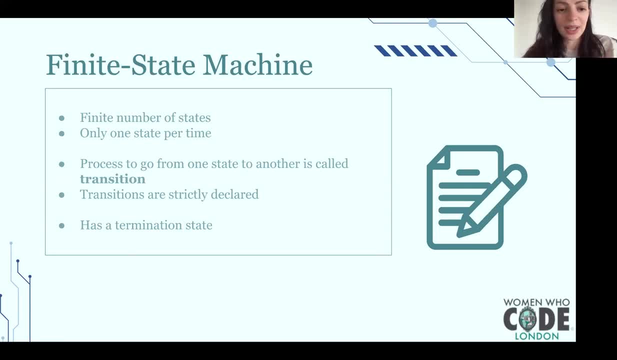 but you can go from active to create. it's strictly declared, strictly declared, strictly declared. if you, if you try to go to active for if you, if you try to go to active for if you, if you try to go to active, for example, from example, from example, from create, from terminated, you can say now: 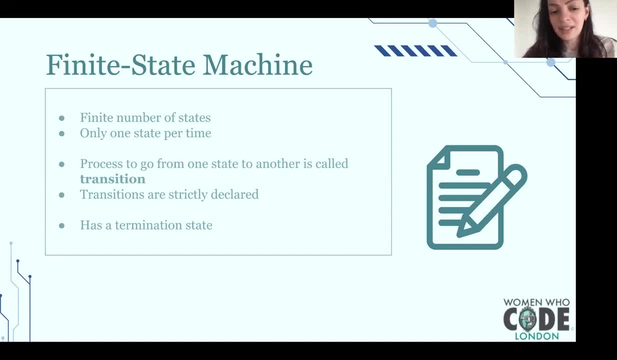 create from terminated. you can say: now create from terminated. you can say: now, it's an error, it's an error, it's an error. so that's mean transitions. so so, that's mean transitions. so so that's mean transitions, so ways from one state to another state. 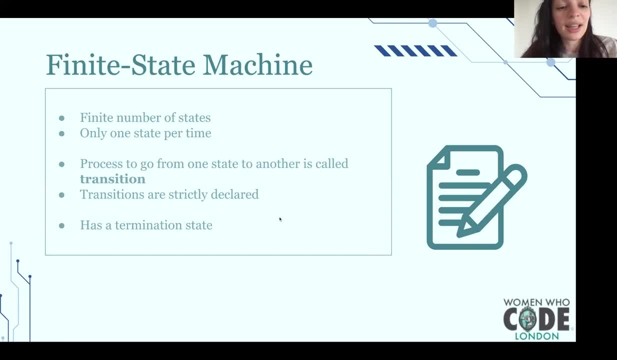 ways from one state to another state, ways from one state to another state. they're strictly. they're strictly, they're strictly declared, declared. declared and and and finite machine, finite machine. finite machine has a termination state, has a termination state, has a termination state. but you can. but you can. 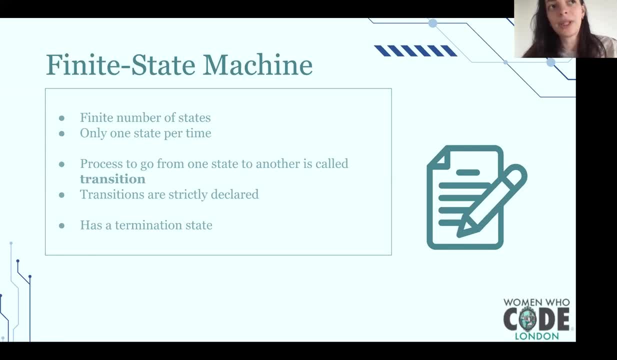 but you can, for example, declare that, for example, declare that, for example, declare that, even if my model terminated, it can be, even if my model terminated it can be. even if my model terminated, it can be created again, created again, created again, so you can have transition from. 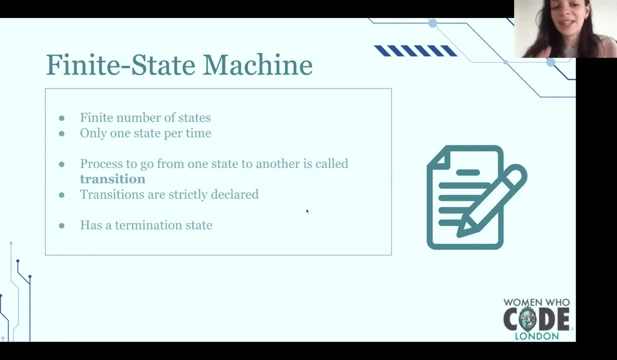 so you can have transition from. so you can have transition from termination state to the first state, termination state to the first state, termination state to the first state. okay, i hope everything is clear, please. okay, i hope everything is clear, please. okay, i hope everything is clear. please let me know if you have any questions. 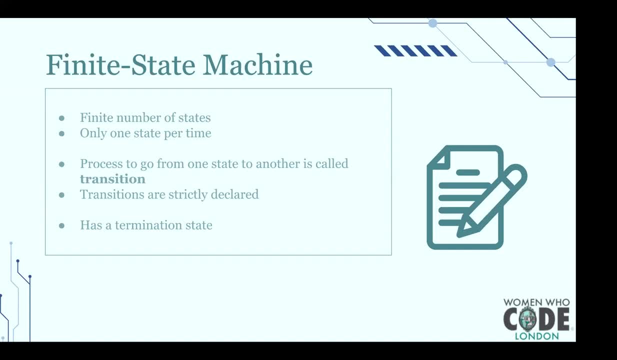 let me know if you have any questions. let me know if you have any questions. can we see as? can we see as can we see as something like payment, something like payment. something like payment as a state, uh behavioral as a state, uh behavioral as a state, uh behavioral state machine. 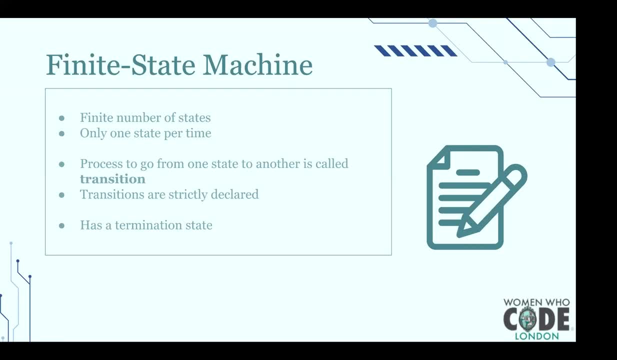 state machine. state machine. like you know, the payment is started. like you know, the payment is started. like you know, the payment is started and at the end it will be paid so money and at the end it will be paid so money and at the end it will be paid so money. transaction. 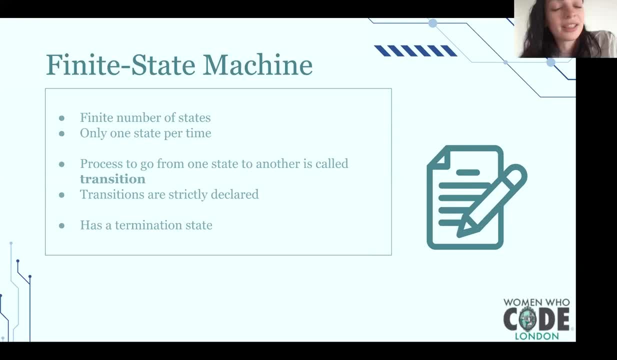 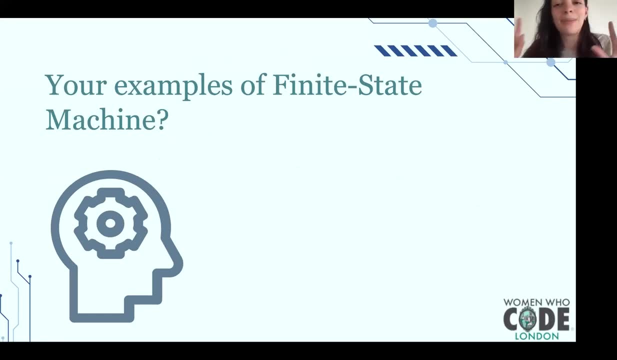 transaction, transaction. is it something? is it something? is it something? yes, yes, yes, yes, it's exactly the example transaction. yes, it's exactly the example transaction. yes, it's exactly the example transaction: money transaction. it can be especially money transaction. it can be especially money transaction. it can be especially in our world where we have 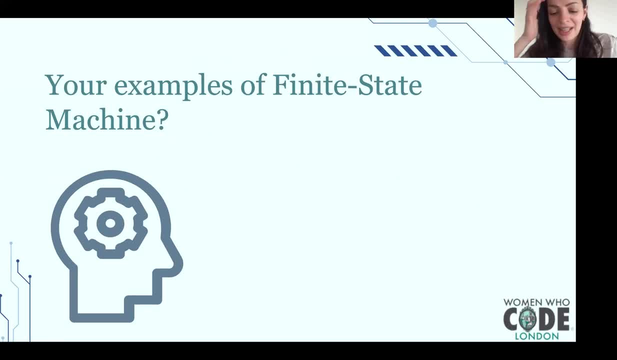 in our world, where we have in our world, where we have a lot of parties, which a lot of parties, which a lot of parties which participate in these transactions, participate in these transactions, participate in these transactions. so, yes, it's applied to transaction. so, yes, it's applied to transaction. 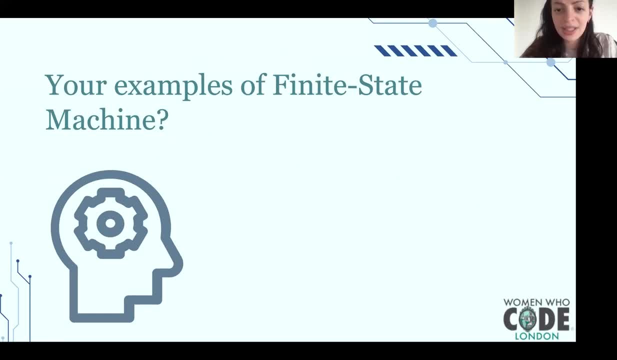 so, yes, it's applied to transaction. perfectly, perfectly, perfectly. transactions can be created, transactions can be created. transactions can be created. can be, can be. can be processed by visa, by mastercard, processed by visa, by mastercard, processed by visa by mastercard, can be- i don't know- can be also. 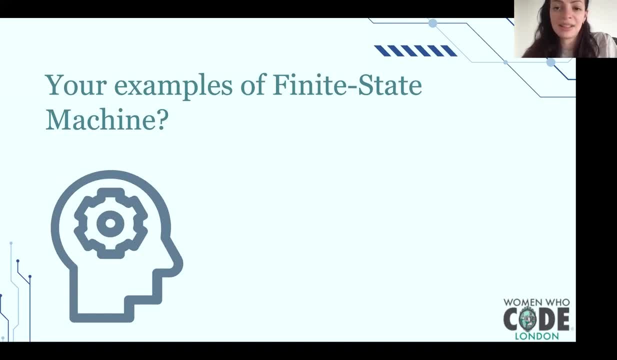 i don't know, can be also, i don't know, can be also charged or paid, charged or paid, charged or paid, and and and completed, for example, completed, for example, completed, for example. so, yeah, that's so, yeah, that's so, yeah, that's exactly, exactly, exactly, exactly also. 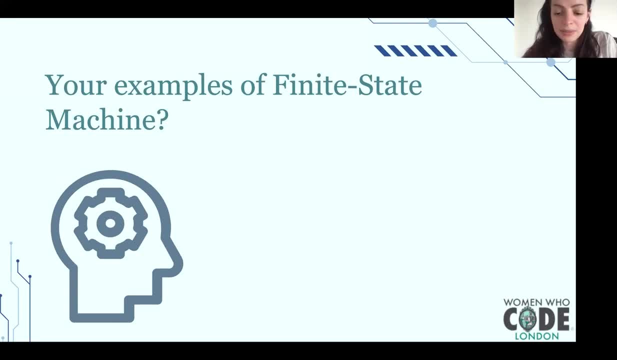 also also user life of user in your system. user life of user in your system. user life of user in your system. it's also perfectly fit with finite state. it's also perfectly fit with finite state. it's also perfectly fit with finite state. machine like, machine like. 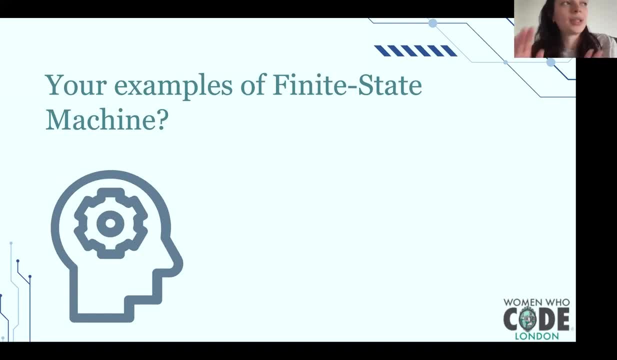 machine like user, user, user, authorization, so it can be created, but authorization, so it can be created, but authorization, so it can be created, but not, not, not go through authorization state or not go through authorization state or not go through authorization state or not. prove their documents. prove their documents. 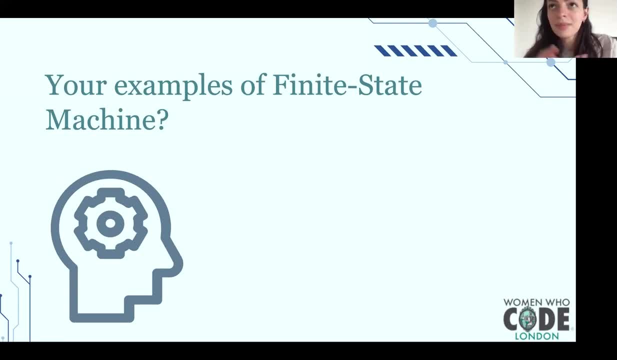 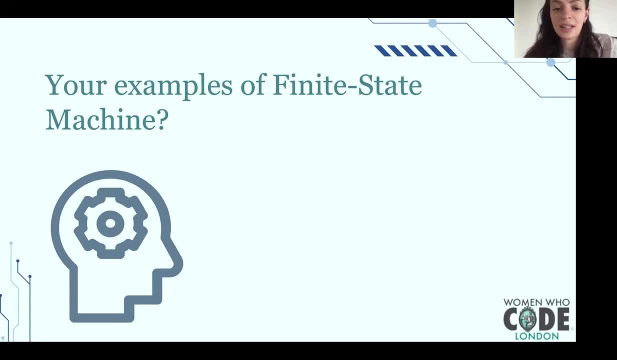 and then it's active state and it also. and then it's active state and it also can, can, can, left your system. decide to sign off from left. your system decide to sign off from left your system decide to sign off from your service, your service, your service, and now you say it's in terminated state. 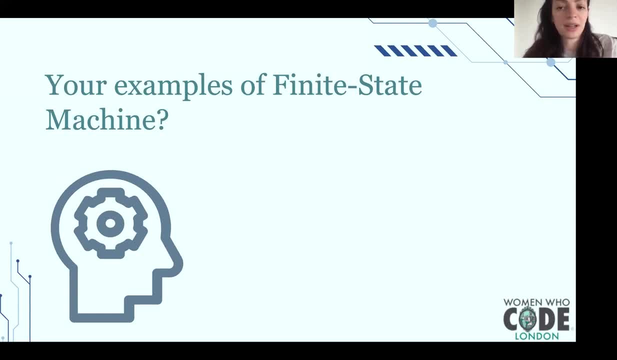 and now you say it's in terminated state. and now you say it's in terminated state, or it can shut down your subscription, or it can shut down your subscription, or it can shut down your subscription and be shut downed and be shut downed and be shut downed. or, for example, it's can be terminated, but 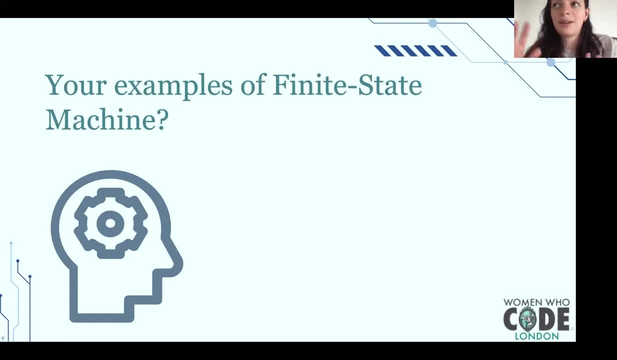 or, for example, it's can be terminated, but. or, for example, it's can be terminated, but also it can be deleted, so you can have like 10 different states. so you can have like 10 different states, so you can have like 10 different states for user. 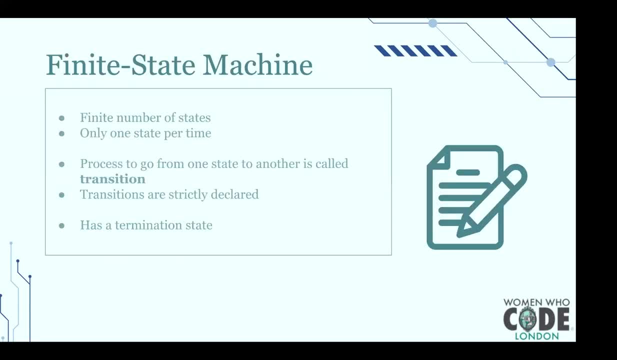 for user, for user in your system, in your system, in your system, and also some, and also some, and also some other example would be. other example would be. other example would be: access token, i guess, access token, i guess access token. i guess which, which which started it has a lifespan. 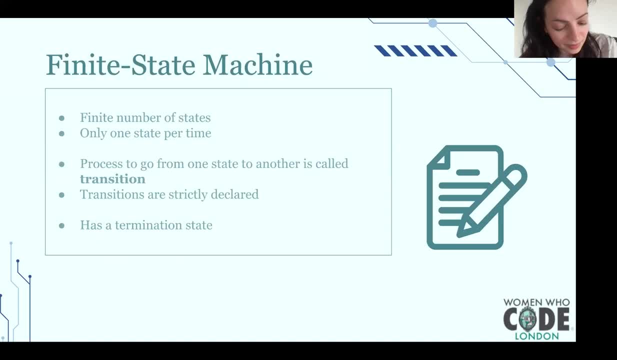 started. it has a lifespan, started, it has a lifespan, and after that, some, and after that, some, and after that some, depending on the. this similar to this, depending on the. this similar to this, depending on the. this similar to this. session, for example, one hour, or session, for example, one hour or. 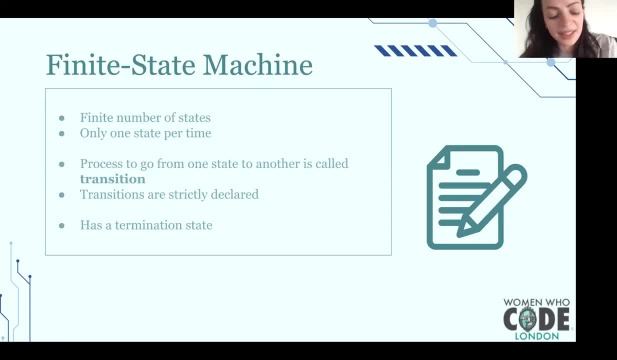 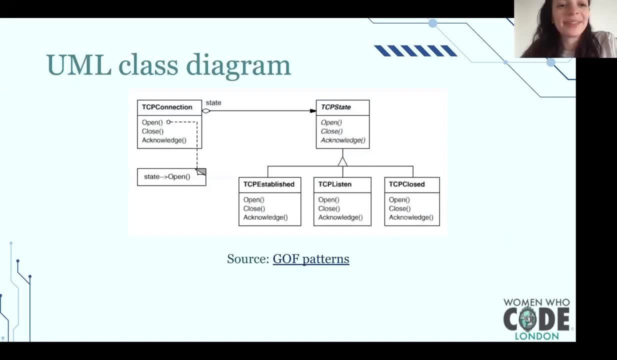 session, for example, one hour or a few hours. yes, a few hours. yes, a few hours. yes, yes, i totally agree, it's a good example. yes, i totally agree, it's a good example. yes, i totally agree, it's a good example. thank you so much. okay, so if you will look at tcp state, 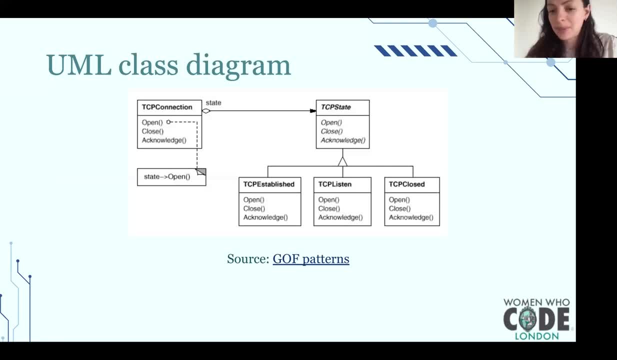 okay, so if you will look at tcp state, okay, so if you will look at tcp state, here is example of how state can be. here is example of how state can be. here is example of how state can be implemented, implemented, implemented. this is example on official gov. 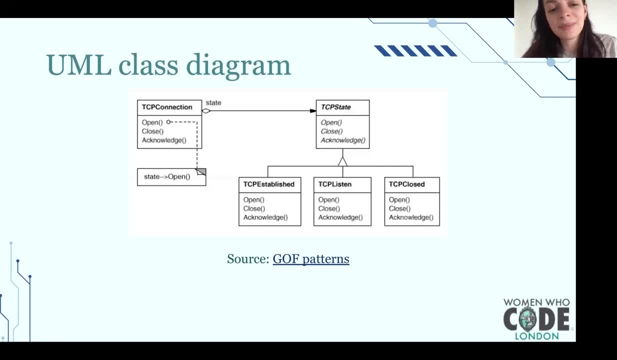 this is example on official gov. this is example on official gov: pattern site. so pattern site, so pattern site. so if you'd like, you can check as well. if you'd like, you can check as well. if you'd like, you can check as well. tcp connection: have tcp state which is: 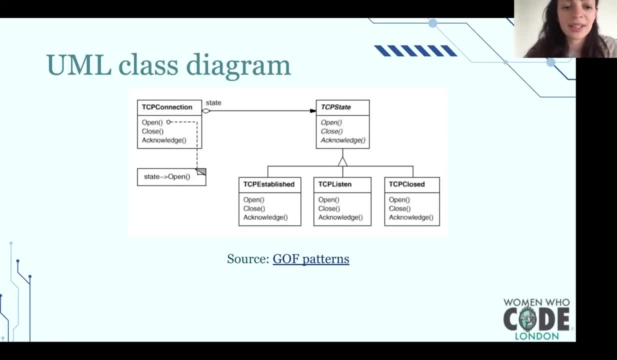 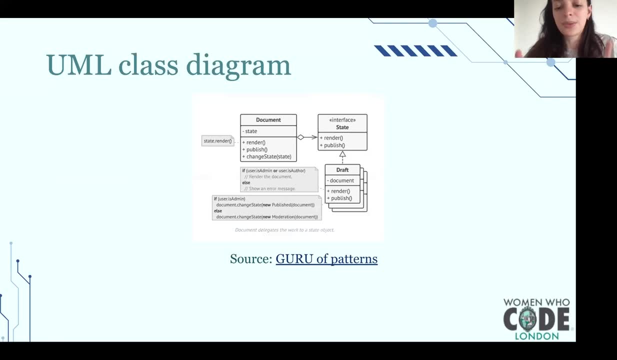 tcp connection, have tcp state which is tcp connection. have tcp state which is established, established. another good example. it's a site- another good example. it's a site. another good example. it's a site that's called google of patterns, that's called google of patterns, that's called google of patterns, and they have very beautiful catalog of. 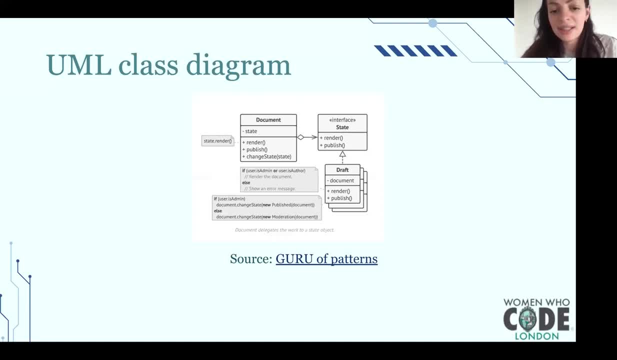 and they have very beautiful catalog of, and they have very beautiful catalog of patterns as well, patterns as well, patterns as well. i will recommend it. they say i will recommend it. they say i will recommend it. they say about document. so document, about document. so document about document. so document has also stayed. 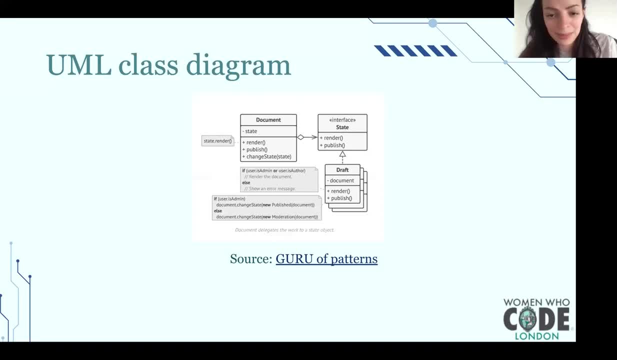 has also stayed, has also stayed, and draft is a state of document so, and draft is a state of document so, and draft is a state of document. so example is pretty simple. like example is pretty simple. like example is pretty simple, like: only draft state, only draft state. 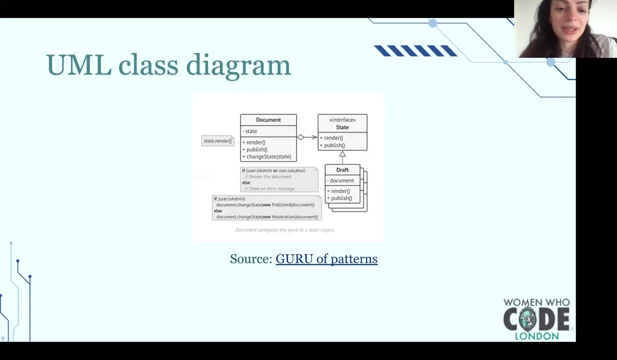 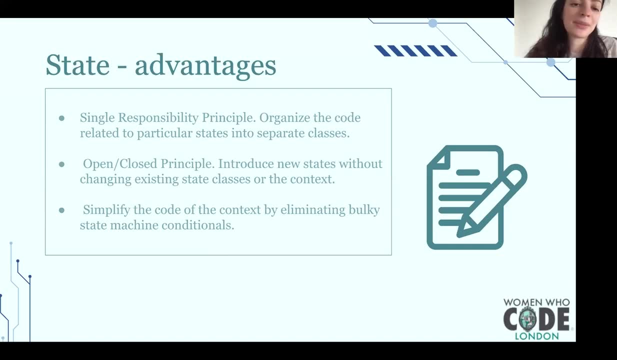 only draft state, and it also applied to, and it also applied to, and it also applied to documenting the system. advantages of this pattern. first of all, advantages of this pattern. first of all, advantages of this pattern. first of all, single responsibility principle. single responsibility principle, single responsibility principle. you organized code beautiful. 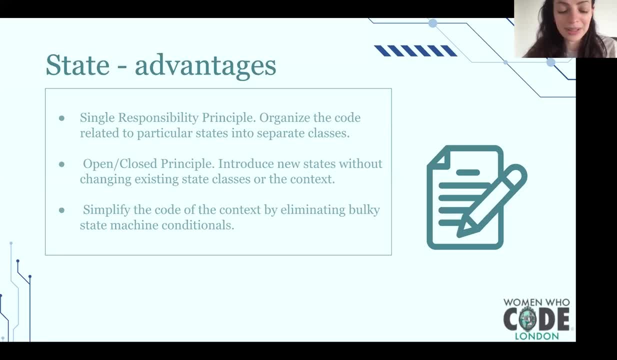 you organized code beautiful. you organized code beautiful. if you remember about our solid solid, if you remember about our solid solid, if you remember about our solid, solid principles, lecture principles, lecture, principles, lecture. and, as i promised, we repeat a bit at, and, as i promised, we repeat a bit at. 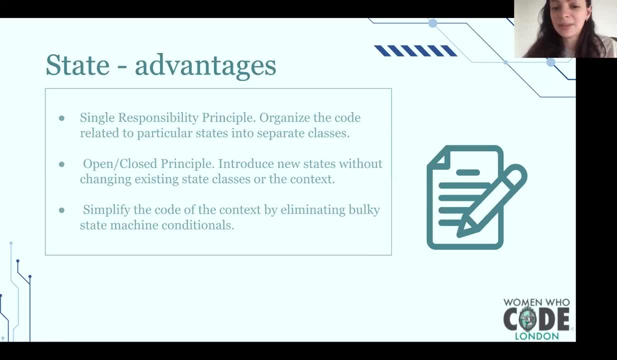 and, as i promised, we repeat a bit at here, here, here. so single responsibility now. so single responsibility now. so single responsibility now, your class responsible, your object, your class responsible, your object, your class responsible, your object responsible responsible, your object responsible for its state, and you don't need to. 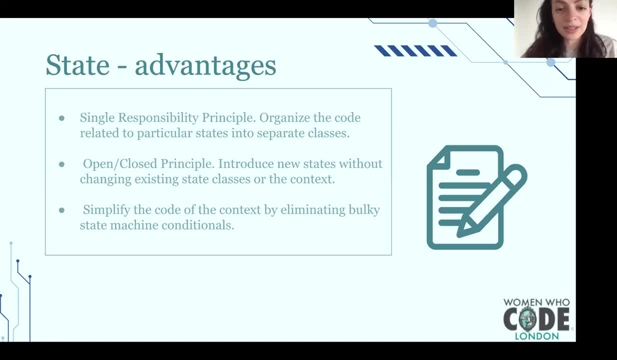 for its state and you don't need to for its state and you don't need to make some another class like collector. make some another class like collector. make some another class like collector for sessions, for sessions, for sessions to be responsible for their state, to be responsible for their state. 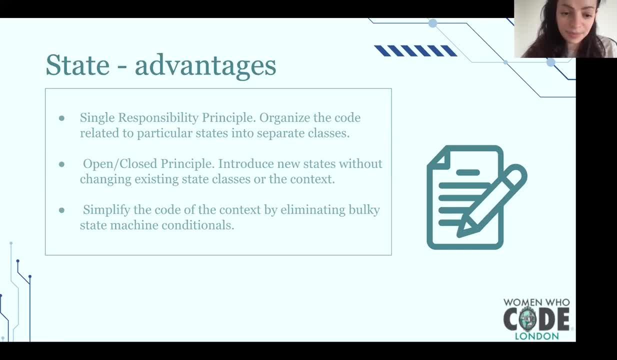 to be responsible for their state- often closed principle. so new states, often closed principle. so new states, often closed principle. so new states, it's very good to. it's very good to. it's very good to say that you know this state, say that you know this state. 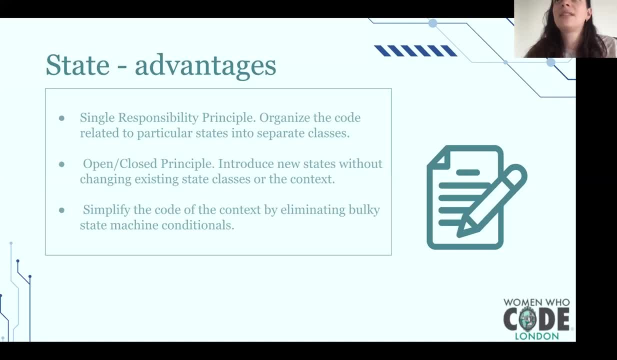 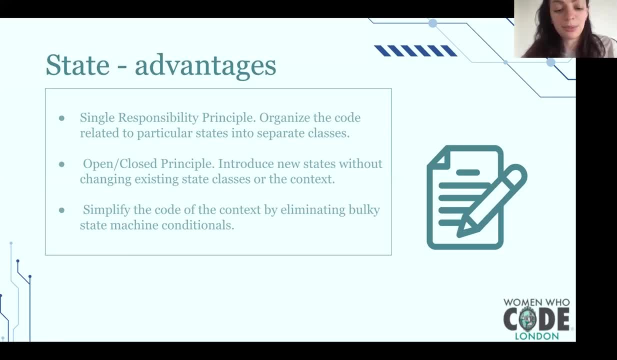 you say that your model become stale. you say that your model become stale and in this, in this case, the method to and in this, in this case, the method to and in this, in this case, the method to make your, make, your, make your objects stale, for example, is closed. 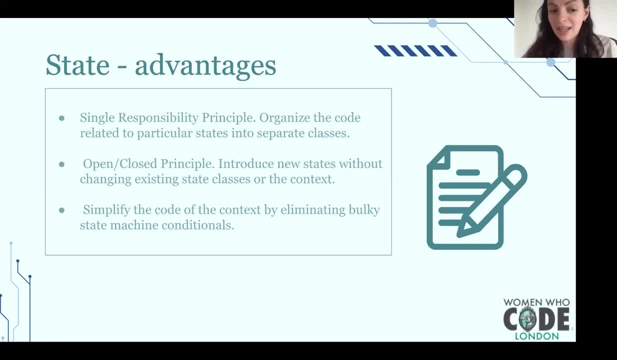 objects stale, for example, is closed. objects stale, for example, is closed. but actual information that now it's. but actual information. that now it's but actual information that now it's stale in the state it's open, stale in the state it's open, stale in the state it's open. and it simplifies the code that 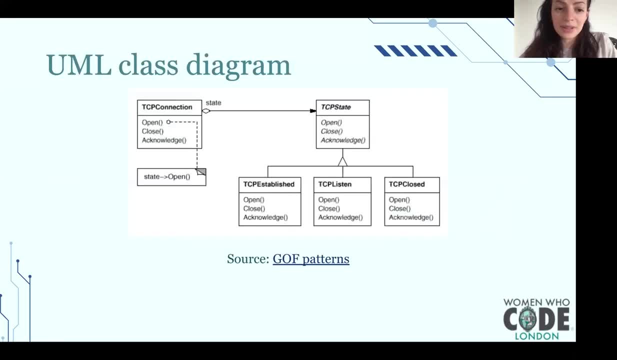 and it simplifies the code that and it simplifies the code that in the context, in the context, in the context, for example, ptp connection, now code. for example, ptp connection, now code. for example, ptp connection, now code. really simplified because you could, really simplified because you could. 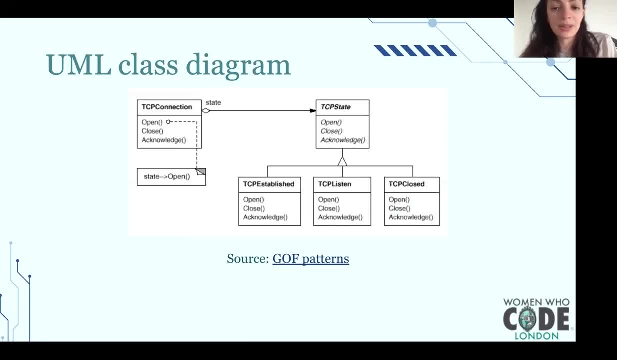 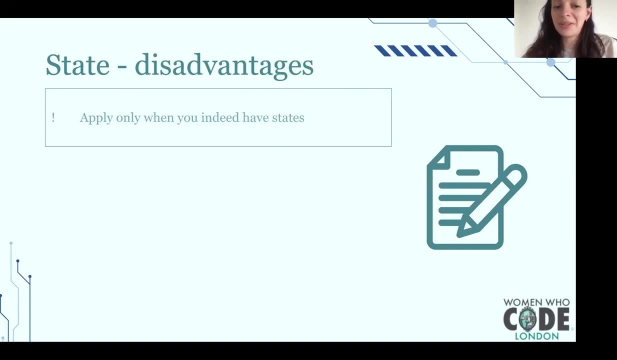 really simplified because you could always logic about established. listen a always logic about established. listen a always logic about established. listen a. closed tcp, closed tcp. closed tcp. state in state okay. state in state, okay. state in state okay. and this advantage apply only when you. and this advantage apply only when you. 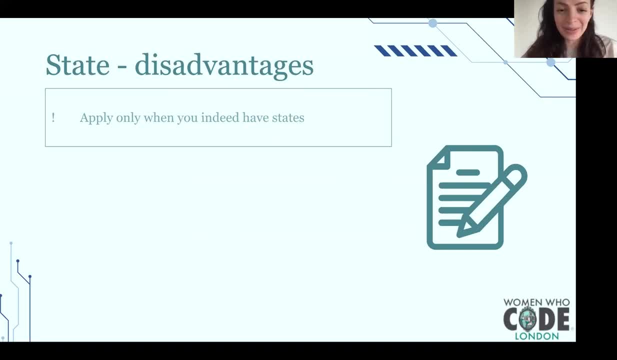 and this advantage apply only when you indeed have states, indeed have states, indeed have states. do not over overuse this pattern, do not over overuse this pattern, do not over overuse this pattern. okay, okay, okay. any questions about state, okay, any questions about state, any questions about state. and now let's go to strategy. 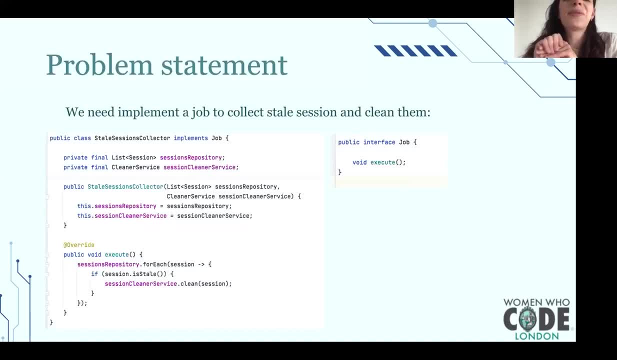 and now let's go to strategy. and now let's go to strategy. i love this pattern, i love this pattern, i love this pattern. so so so, the example here now. the example here now. the example here now: again, our style session collector, again our style session collector. 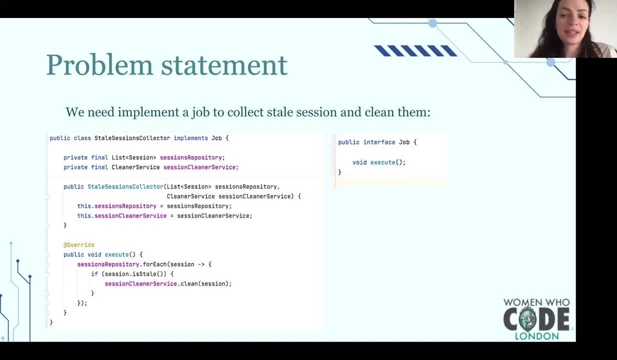 again our style session collector. we need to implement a job to collect. we need to implement a job to collect. we need to implement a job to collect stale sessions and clean them stale sessions, and clean them, stale sessions and clean them. so basically, we have interface and job. 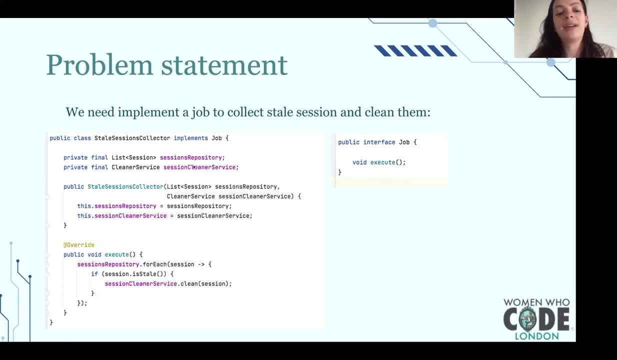 so basically we have interface and job. so basically we have interface and job, which which which execute something, and we have this execute something, and we have this execute something, and we have this session repository again session repository, again session repository, again session cleaner service and if session session cleaner service and if session. 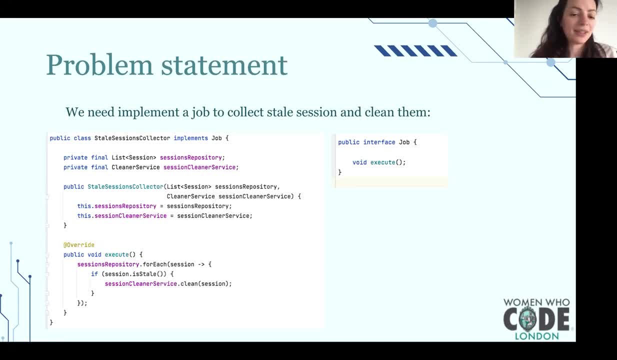 session cleaner service. and if session is stale, is stale, is stale, we clean them. everything is perfect, we clean them. everything is perfect, we clean them. everything is perfect now, ah yeah, and as i promised, now, ah yeah, and as i promised, now, ah yeah, and as i promised, solid principles. so here we implement. 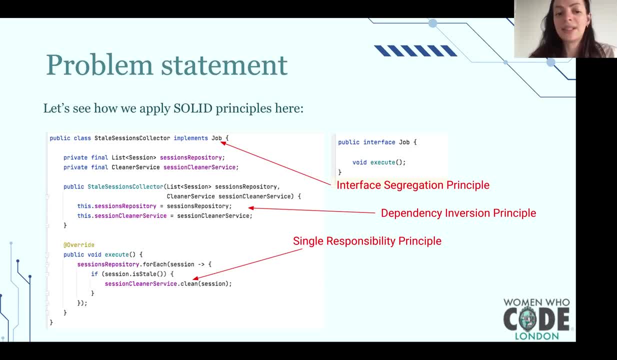 solid principles. so here we implement solid principles. so here we implement interface, but interface, but interface. but when we want to use this session, when we want to use this session, when we want to use this session, collector, collector, collector, job, we just say: you know, i want to. 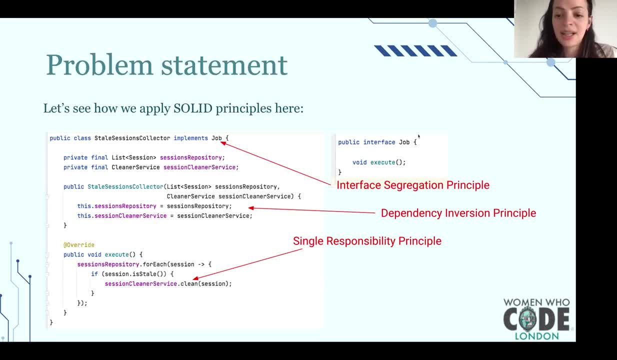 job. we just say you know i want to job. we just say you know i want to execute, execute, execute, job, and i don't care what is job and i don't care what is job and i don't care what is implementation, implementation, implementation. so, with this interfacing relation, 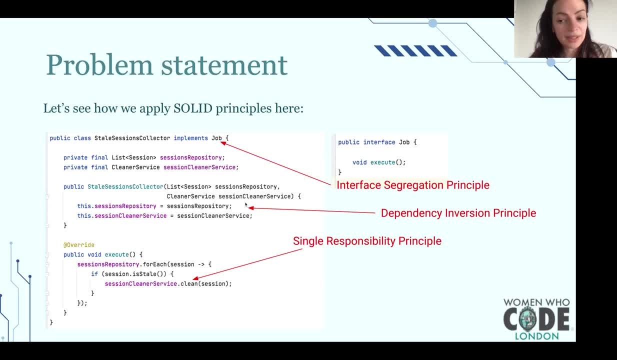 so with this interfacing relation, so with this interfacing relation, principle, principle, principle. we use here dependency inversion. we use here dependency inversion. we use here dependency inversion principle, principle, principle, which means that we could create this, by which means that we could create this, by which means that we could create this by new array list. 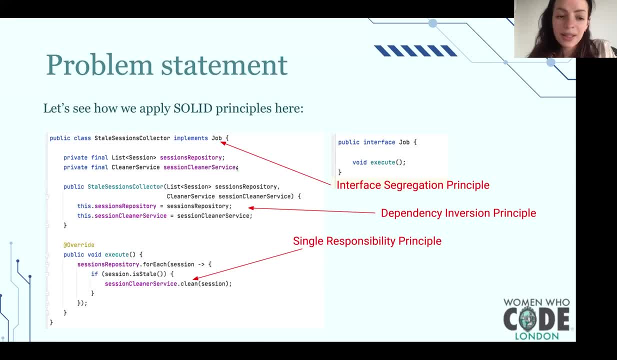 new array list, new array list and the new cleaner service, and the new cleaner service and the new cleaner service, just here in this stale session, just here in this stale session, just here in this stale session. collector, collector, collector. but we instead of for doing it, but we instead of for doing it. 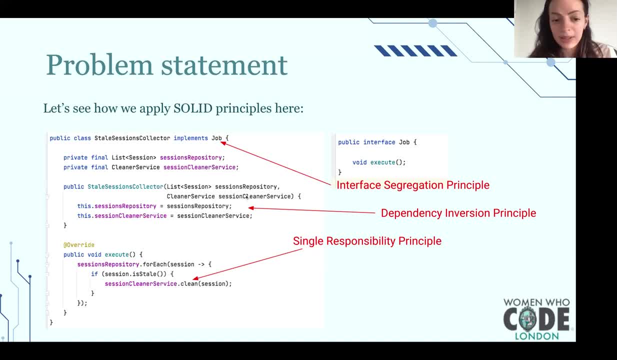 but we, instead of for doing it, we provided it to constructor. so we provided it to constructor, so we provided it to constructor. so this is a very simple step to be. this is a very simple step to be. this is a very simple step to be good person and follow dependency. 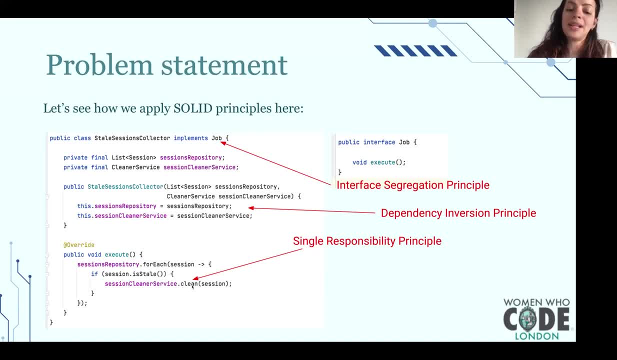 good person and follow dependency. good person and follow dependency, inversion principle, inversion principle, inversion principle. and we have only one method execute and we have only one method execute and we have only one method execute: which, which, which. check method in session and check method in session. and check method in session and get method from session cleaner service. 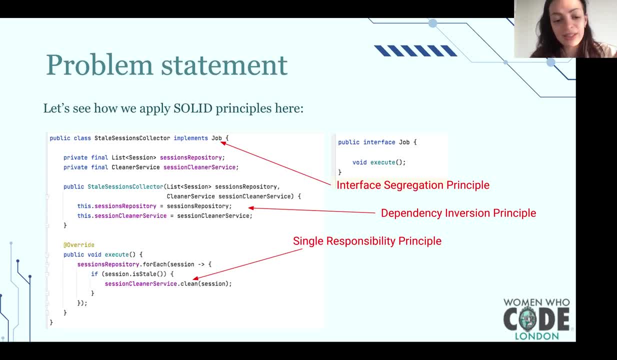 get method from session cleaner service. get method from session cleaner service. clean, so clean, so clean. so our service also have one method. i mean our service also have one method. i mean our service also have one method. i mean we do not try to clean sessions here. we do not try to clean sessions here. 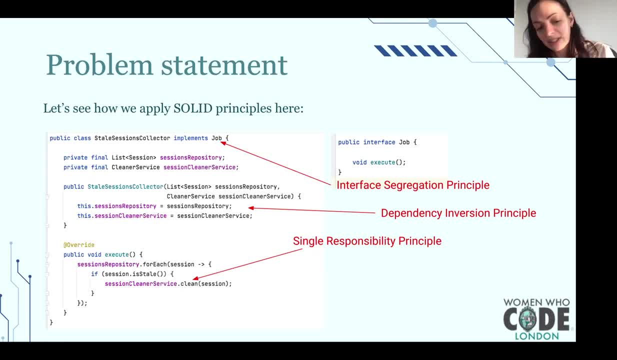 we do not try to clean sessions here, because because because here here we already get them from repository, we already get them from repository, we already get them from repository and check them and check them, and check them and the logic to clean them and the logic to clean them. 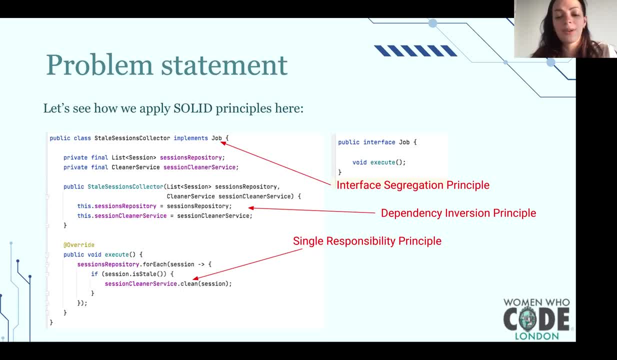 and the logic to clean them, we delegate it to another service, which we delegate it to another service, which we delegate it to another service which allows our, allows our, allows our, our job to be single responsible, only our job to be single responsible, only our job to be single responsible, only for this execution. 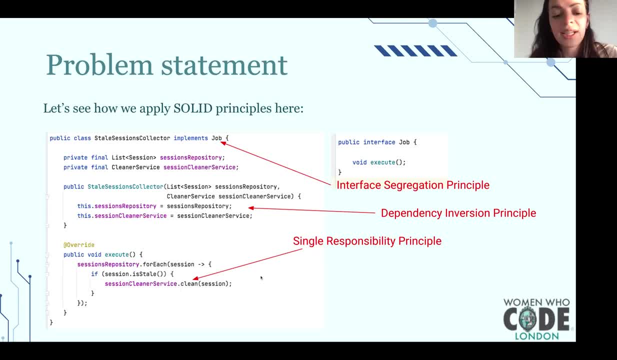 for this execution, for this execution only for with collection of style, only for with collection of style, only for with collection of style. session, session, session, and that's it. it's just step session and that's it. it's just step session and that's it. it's just step session. collector, it's not cleaner. 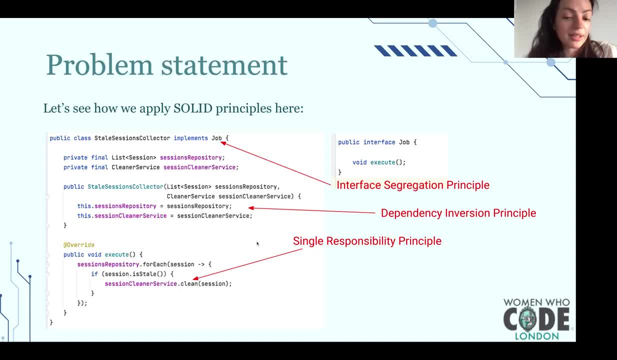 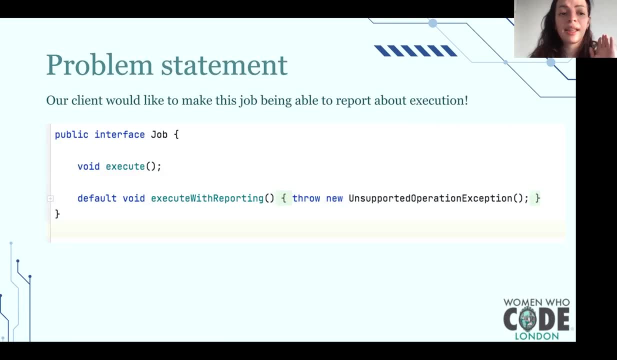 collector: it's not cleaner. collector: it's not cleaner. so we denigrated this. so it's single responsibility principle. so it's single responsibility principle. so it's single responsibility principle. now we already seen how we can test it. now we already seen how we can test it. 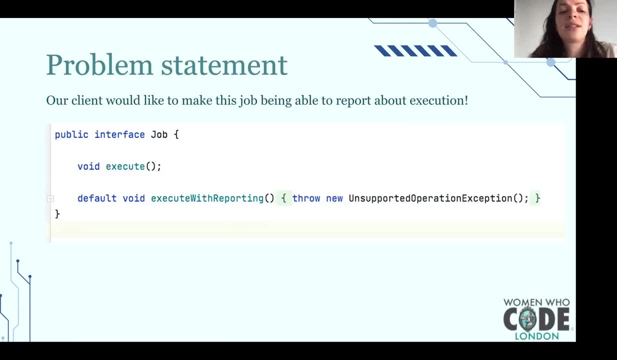 now. we already seen how we can test it now, now, now, our client- our clients- wants to make our client our clients wants to make our client, our clients- wants to make this job, being able to report about this job, being able to report about this job, being able to report about execution, which makes sense. 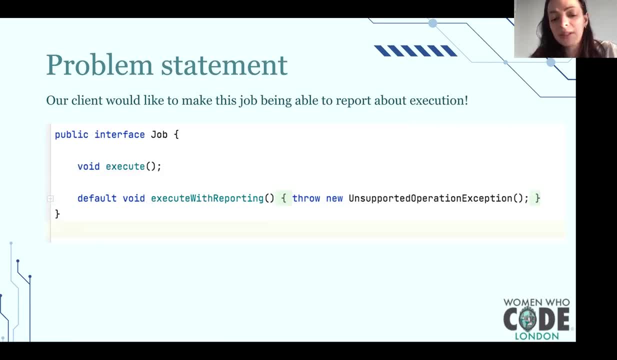 institution which makes sense, institution which makes sense, and and and we decided to create a new method. we decided to create a new method. we decided to create a new method with reporting, with reporting, with reporting. so, in case, if we have reporter, we need. so, in case, if we have reporter, we need. 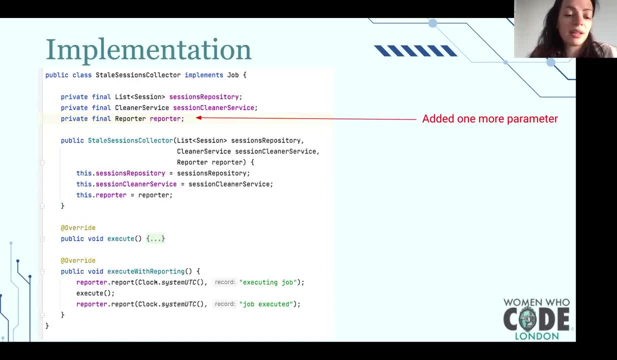 so, in case, if we have reporter, we need to add a reporter. to add a reporter. to add a reporter. we, we, we add their method execute with reporting. add their method execute with reporting. add their method execute with reporting. we do all this reporting and then do it. 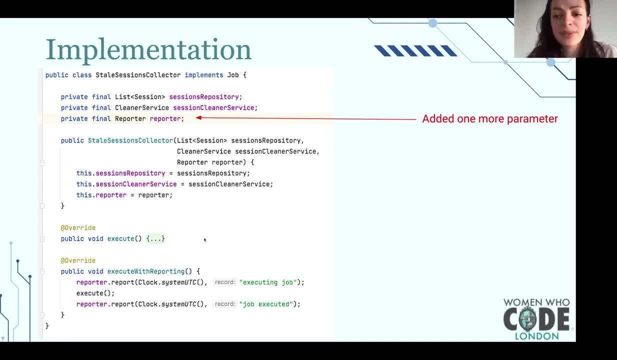 we do all this reporting and then do it. we do all this reporting and then do it securely, securely, securely, we just reuse methods that we already have. we just reuse methods that we already have. we just reuse methods that we already have, and we have more parameters and we have more parameters. 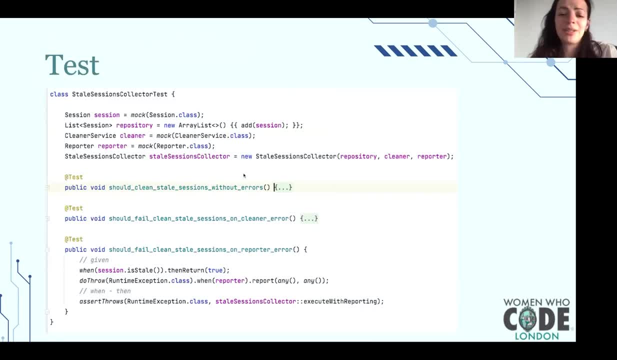 and we have more parameters. now we changed a bit our tests. because now we changed a bit our tests, because now we changed a bit our tests? because we need to create style session. we need to create style session. we need to create style session collector with three parameters. 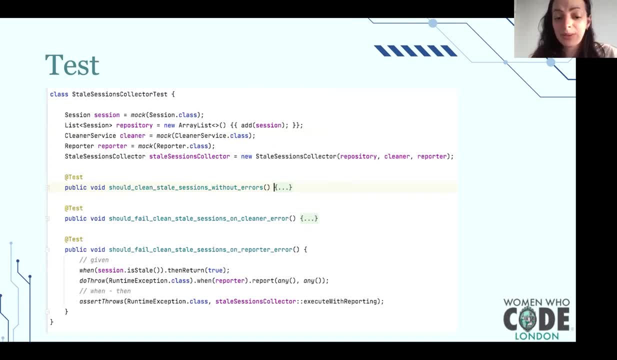 collector with three parameters. collector with three parameters. well, well, well, two, two, two. previous methods to test: they pretty the previous methods to test. they pretty the previous methods to test. they pretty the same, it's good, same. it's good, same, it's good. and we add a new, a new method. 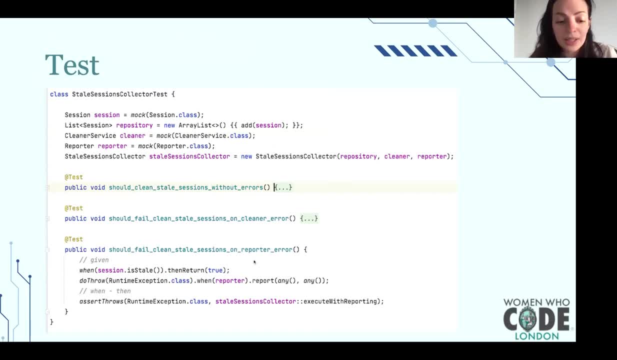 and we add a new, a new method. and we add a new, a new method to test, to test our, to test, to test our, to test, to test our reporter. what if our reporter will fail reporter? what if our reporter will fail reporter? what if our reporter will fail? so we mock with behavior because we mocked. 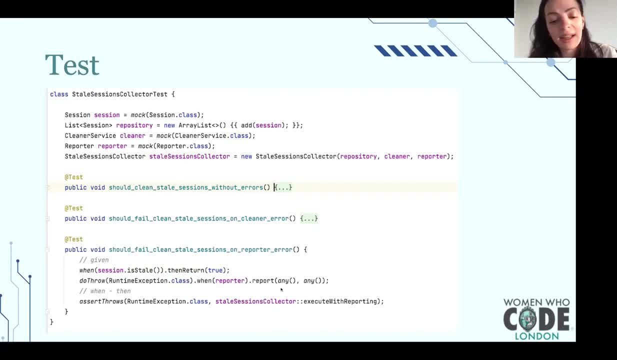 so we mock with behavior because we mocked, so we mocked with behavior because we mocked basically reporter remote with basically reporter remote with basically reporter remote with behavior, behavior, behavior. and we say that and we say that and we say that when we try to report anything which, when we try to report anything which, 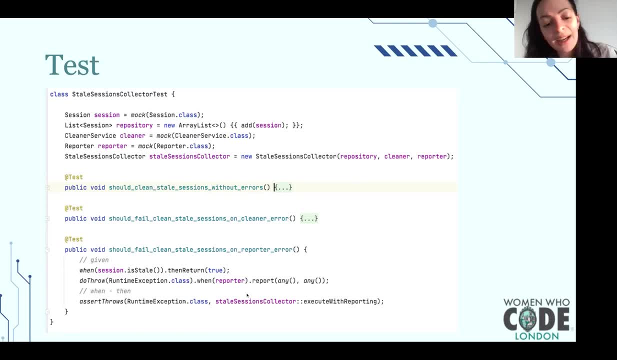 when we try to report anything which market allows. my kit is powerful thing, market allows my kit is powerful thing. market allows my kit is powerful thing. uh, we throw exception. uh, we throw exception. uh, we throw exception. that if something you wrong with reporter, that if something you wrong with reporter. 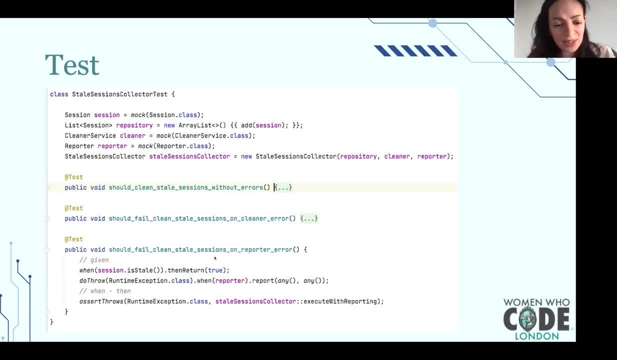 that if something you wrong with reporter, we will also have exception, we will also have exception. we will also have exception. which makes sense, which pretty simple, which makes sense, which pretty simple, which makes sense, which pretty simple. but but but because you want to test it, you would 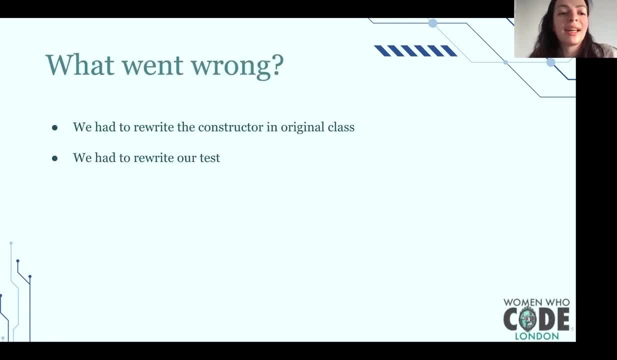 because you want to test it. you would. because you want to test it, you would like to like, to like to create more tests on it and create more tests on it, and create more tests on it. and what went wrong? what went wrong? what went wrong? first of all, we had to rewrite the 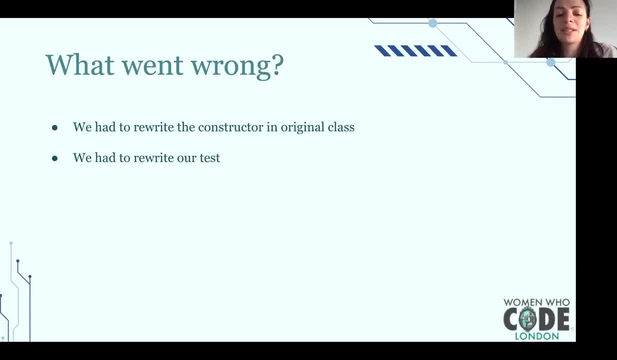 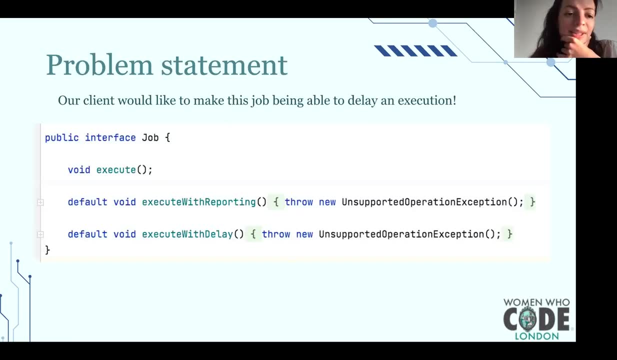 first of all, we had to rewrite the first of all, we had to rewrite the constructor, constructor, constructor. and we had to rewrite our tests, and we had to rewrite our tests, and we had to rewrite our tests a bit, but yet a bit, but yet a bit, but yet. okay, we can survive with it. now our 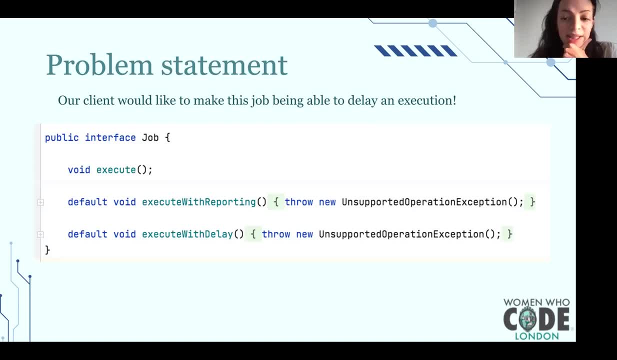 okay, we can survive with it now. our okay, we can survive with it now. our client would like to make this job. being client would like to make this job. being client would like to make this job being able to delay in execution, able to delay in execution, able to delay in execution. so 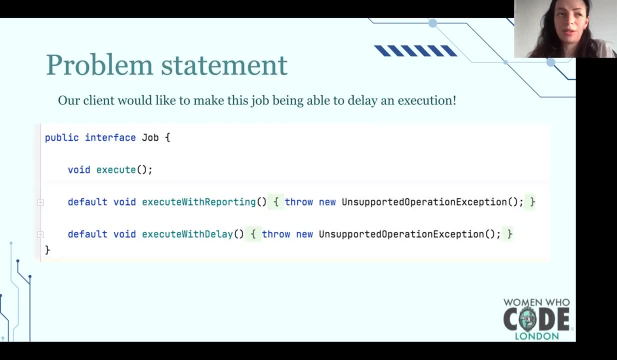 so. so this is a job, but some application need: this is a job, but some application need: this is a job, but some application need job to be not at the start of application. job to be not at the start of application. job to be not at the start of application but after some time to be sure that all 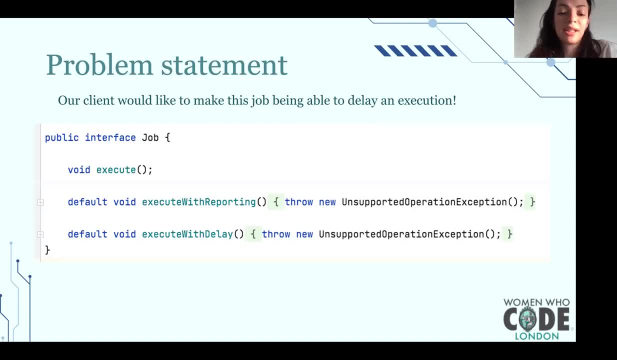 but after some time to be sure that all, but after some time to be sure that all resources, for example resources, for example resources, for example, all resources initialized, all resources initialized, all resources initialized. okay, okay, okay. we say okay, now we have new parameter. we say okay, now we have new parameter. 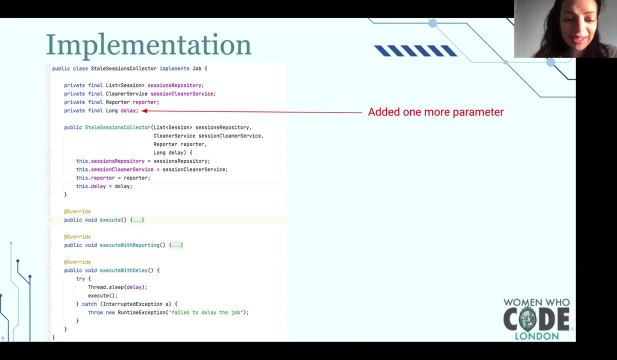 we say: okay, now we have new parameter on delay. we put it in constructor. we put on delay. we put it in constructor, we put on delay, we put it in constructor. we put a new method: execute this delay. a new method, execute this delay. a new method, execute this delay. we say that you know we can suspend our. 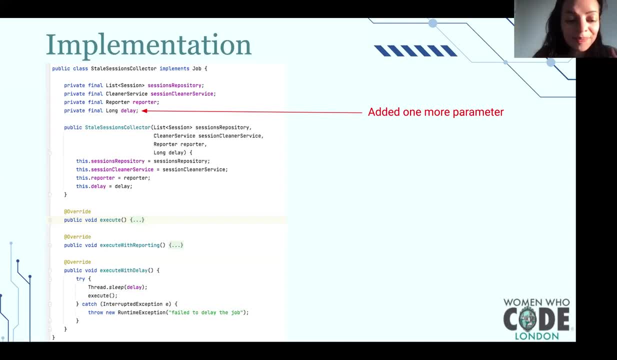 we say that you know we can suspend our. we say that you know we can suspend our program, program program, for example, by thread sleep delay. for example by thread sleep delay. for example by thread sleep delay. this is just for this thread sleep delay. this is just for this thread sleep delay. 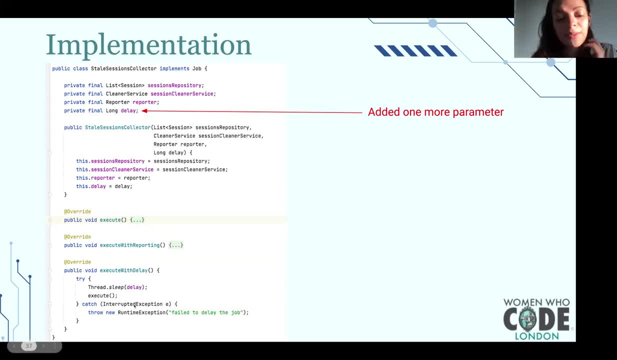 this is just for this thread: sleep delay method method, method to, because it's thread to, because it's thread to, because it's thread, we also need to catch interruption. we also need to catch interruption. we also need to catch interruption. exception, exception, exception, and we just, and we just. 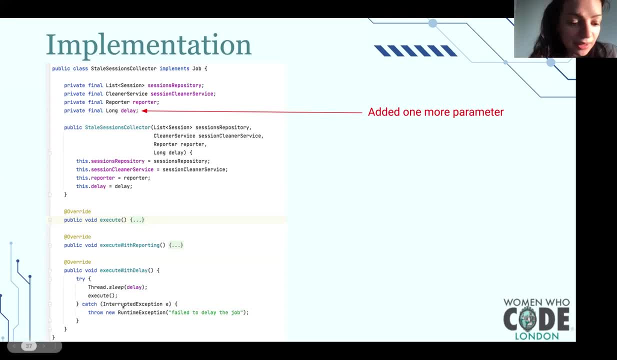 and we just create new exception, but with some details: create new exception, but with some details, create new exception, but with some details of what's happening, of what's happening, of what's happening, and we just execute the method or execute and we just execute the method or execute. 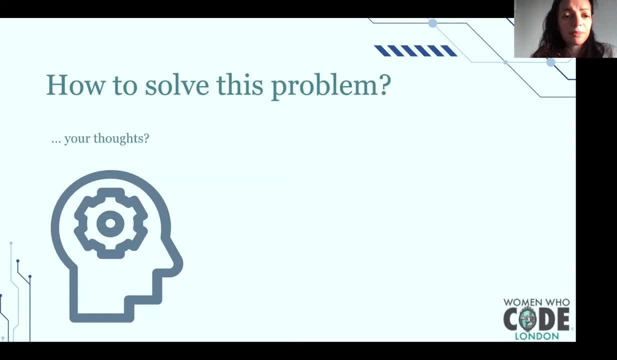 and we just execute the method, or execute with reporting, with reporting, with reporting, so so. so it's not really beautiful, it's not really. it's not really beautiful, it's not really. it's not really beautiful, it's not really flexible, flexible, flexible. and what are your thoughts how we can? 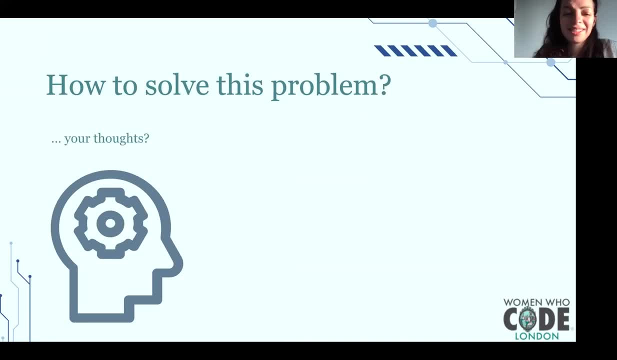 and what are your thoughts how we can, and what are your thoughts how we can make it better, make it better, make it better? any ideas, any ideas, and my solution here is execution and my solution here is execution and my solution here is execution, strategy, strategy, strategy. so we say that. 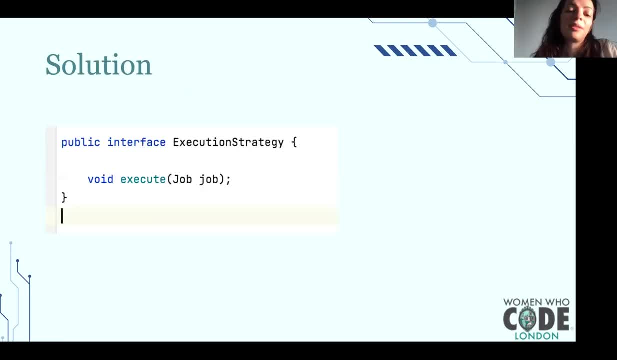 so we say that. so we say that execute method, execute method, execute method, uh of, uh of, uh of. job is the same, but we also have some job is the same, but we also have some job is the same, but we also have some strategy, strategy, strategy: how to execute this job. 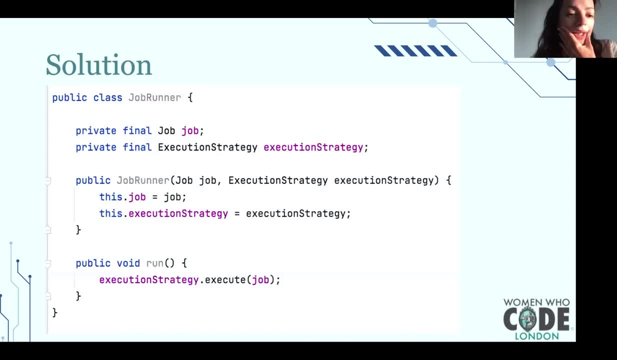 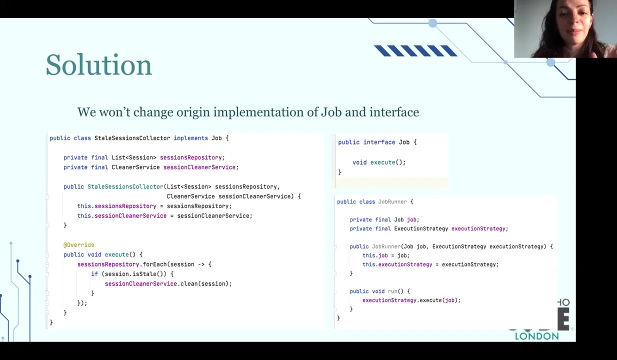 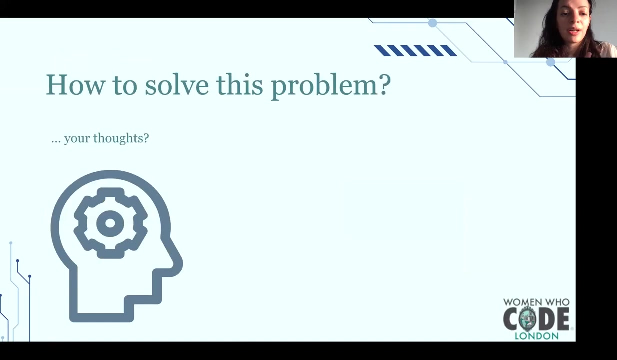 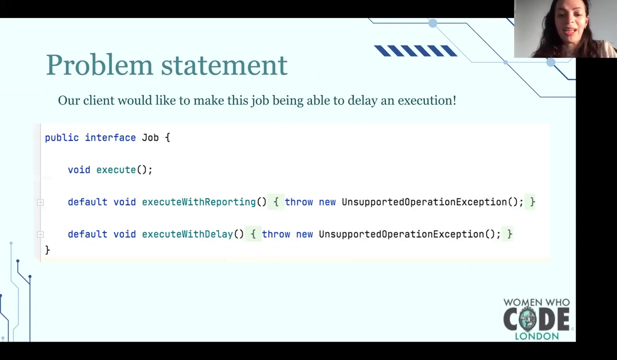 how to execute this job, how to execute this job, and and and and this job, this job, this job should execute with reporting, even if should execute with reporting, even if should execute with reporting, even if it doesn't have to execute with reporting. it doesn't have to execute with reporting. 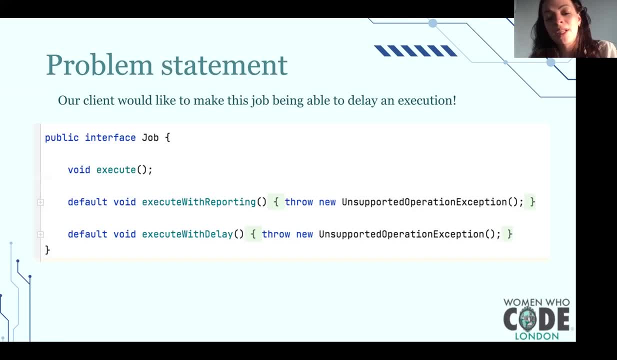 it doesn't have to execute with reporting. so so so another class, another, any job, another class, another any job, another class, another, any job, could, could, could, create, execute with reporting, create, execute with reporting, create, execute with reporting and throw their exception like, and throw their exception like. 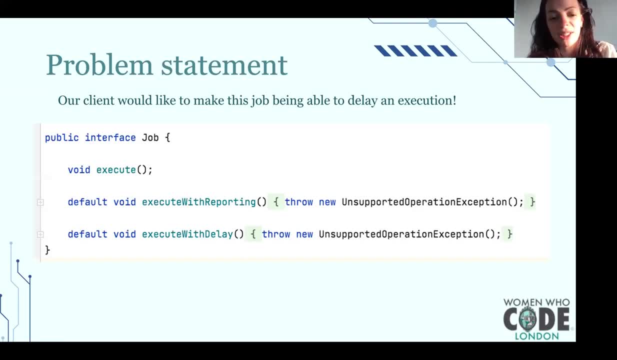 and throw their exception like unsupported exception. i do not support unsupported exception. i do not support unsupported exception. i do not support this method, this method, this method. but yeah, java 8, allow us to do it in. but yeah, java 8, allow us to do it in. 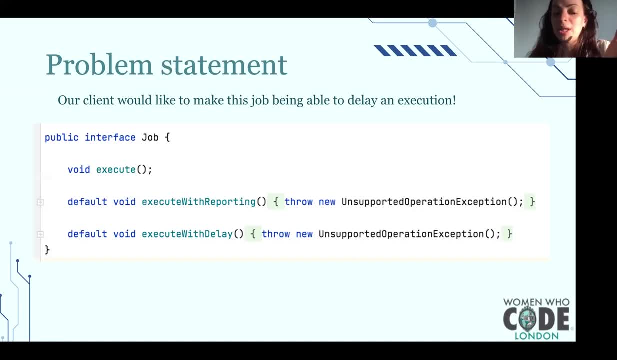 but yeah, java 8, allow us to do it in interface, which means that we can make interface, which means that we can make interface, which means that we can make our interfaces more flexible, our interfaces more flexible, our interfaces more flexible, and, and, and. but now we don't need even do it. we. 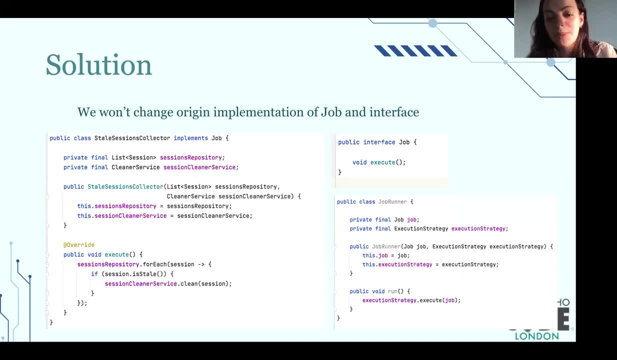 but now we don't need even do it we, but now we don't need even do it, we, just just just. we just remain the same job with the. we just remain the same job with the. we just remain the same job with the method execute, which pretty simple, which. 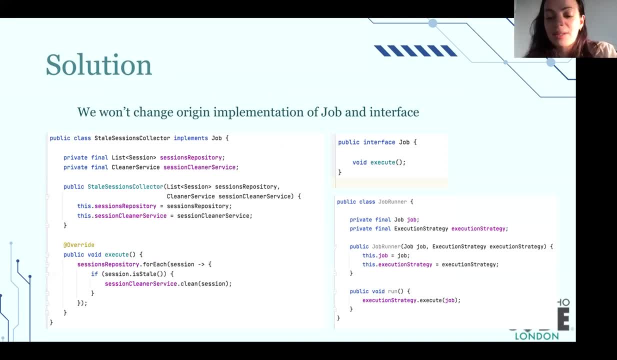 method execute, which pretty simple, which method execute, which pretty simple, which can be, can be, can be even functional interface, even functional interface, even functional interface. that's very beautiful, that's very beautiful, that's very beautiful, and we say that now we have job, and we say that now we have job. 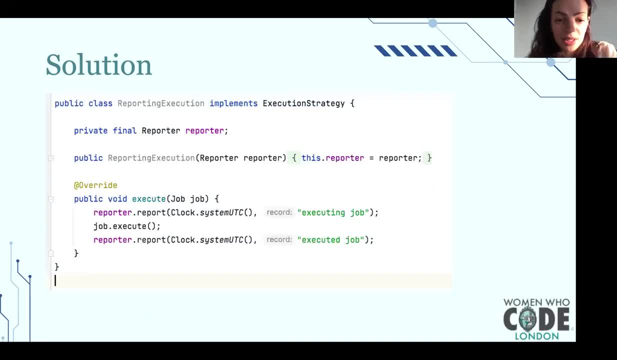 and we say that now we have job runner, runner, runner, again job runner get this drop, and again job runner get this drop, and again job runner get this drop, and that's it. and what can be the strategy? that's it, and what can be the strategy? that's it, and what can be the strategy, the strategy with reporting. so 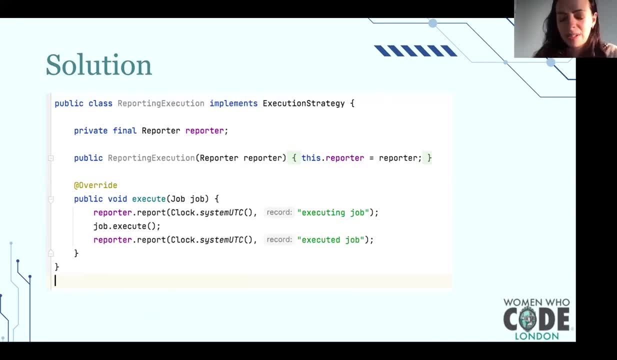 the strategy with reporting, so the strategy with reporting. so now our reporter goal, not in our previous. now our reporter goal, not in our previous. now our reporter goal, not in our previous. style style: style session: collector class with this job session. collector class with this job session. collector class with this job. it's goal to execution strategy. 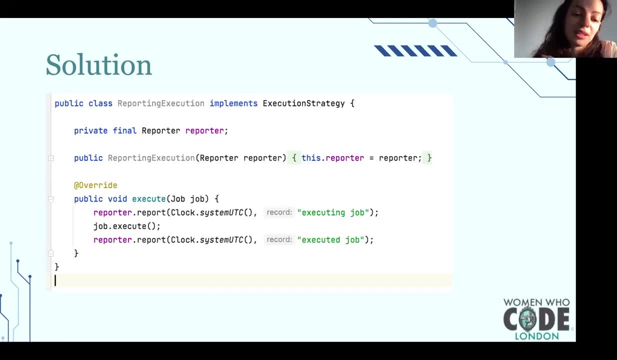 it's goal to execution strategy. it's goal to execution strategy. and now we say, and now we say, and now we say that, execute that, execute that, execute. a job with reporter, a job with reporter, a job with reporter, we can do it by reporting. we can do it by reporting. 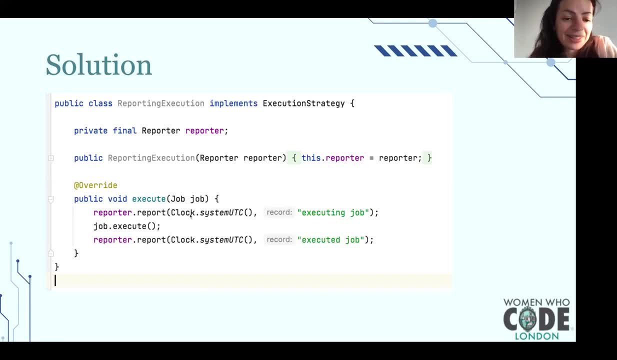 we can do it by reporting, and then we execute job, and then we execute job, and then we execute job. uh, yeah, i hope i hope it's clear. uh, yeah, i hope i hope it's clear. uh, yeah, i hope i hope it's clear. let's look at delaying strategy: delaying- 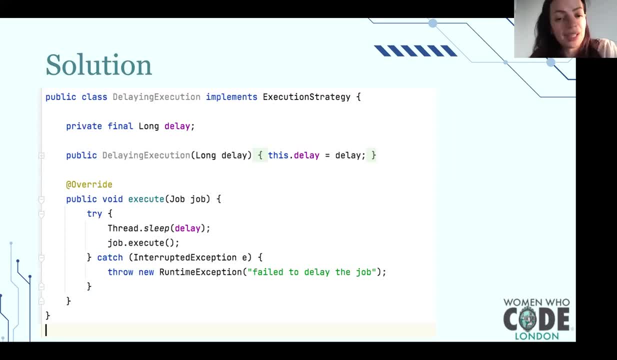 let's look at delaying strategy- delaying- let's look at delaying strategy. delaying execution, execution, execution. now we say that you know we want to. now we say that you know we want to. now we say that you know we want to delay our execution, delay our execution, delay our execution and we put the parameter long delay. 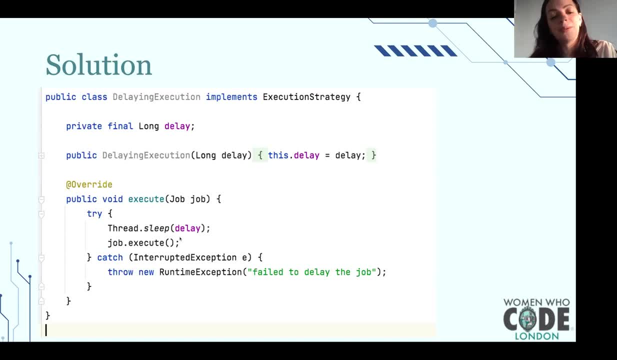 and we put the parameter long delay and we put the parameter long delay and and we put the parameter long delay and and we put the parameter long delay and we say that. we say that, we say that, okay, we will sleep before this before. okay, we will sleep before this before. 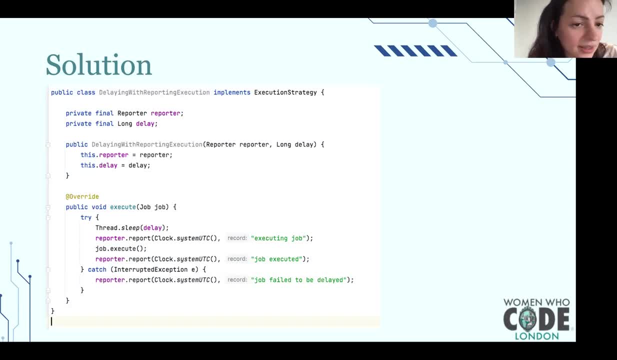 okay, we will sleep before this, before execute, and we even can execute and we even can execute and we even can combine with strategies so we can create, combine with strategies so we can create, combine with strategies so we can create. a new one delaying with reporting, a new one delaying with reporting. 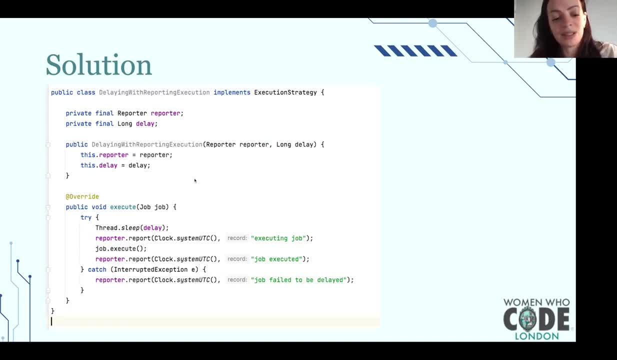 a new one, delaying with reporting, execution, execution, execution. put there both reporter and delay, and put there both reporter and delay, and put there both reporter and delay. and now we say: now we say, now we say first of all we delay, then we report, and first of all we delay, then we report, and 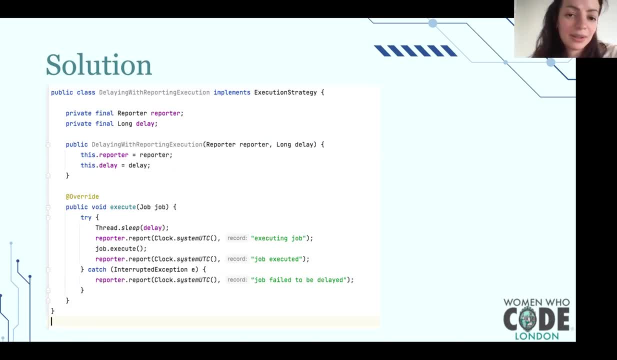 first of all we delay, then we report and then we execute, so we can combine them by then we execute, so we can combine them. by then we execute. so we can combine them by new execution strategy. new execution strategy, new execution strategy. okay, i hope it's clear. i hope it's. 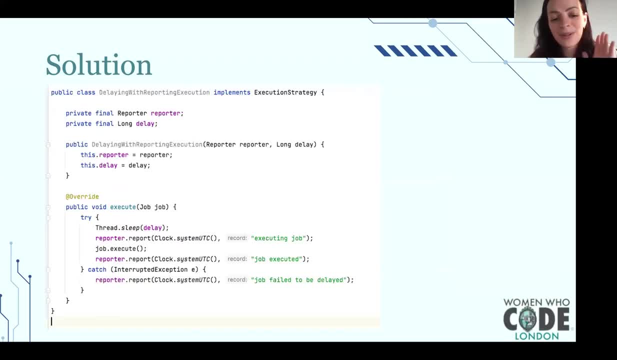 okay, i hope it's clear. i hope it's okay. i hope it's clear. i hope it's like it's clear what is strategy like. it's clear what is strategy like. it's clear what is strategy. it's super real life examples. it's super real life examples. 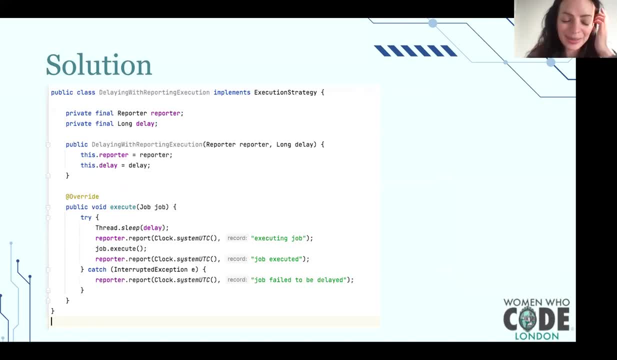 it's super real life examples, so it's not. it's super real life. so it's not. it's super real life. so it's not. it's super real life examples. that's why they probably be examples. that's why they probably be examples. that's why they probably be more complicated. 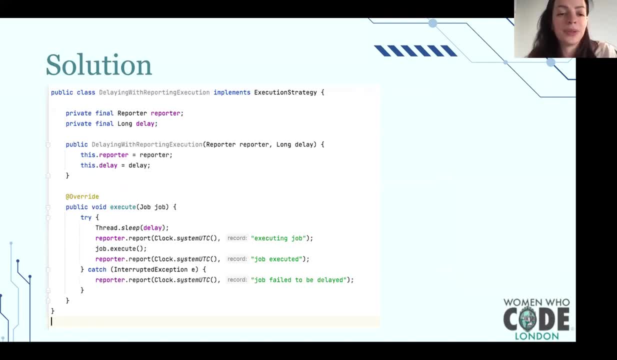 more complicated, more complicated. but i hope for, but i hope for, but i hope for. you know it will be super useful in your. you know it will be super useful in your. you know it will be super useful in your real life, real life, real life. uh, if you would like an original, 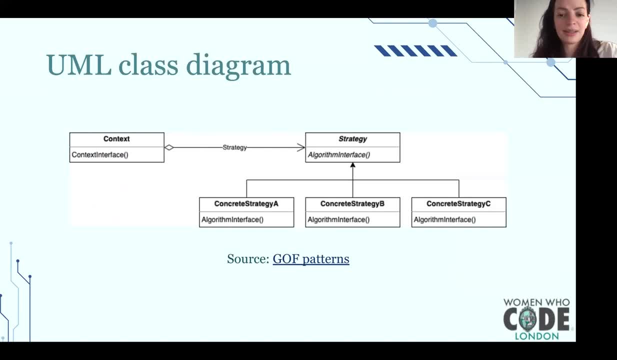 uh, if you would like an original, uh, if you would like an original diagram for any strategy pattern diagram, for any strategy pattern diagram, for any strategy pattern, it will looks like this, so you have. it will looks like this, so you have. it will looks like this, so you have strategy. 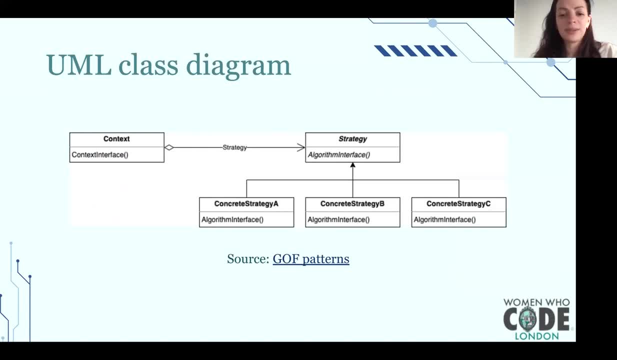 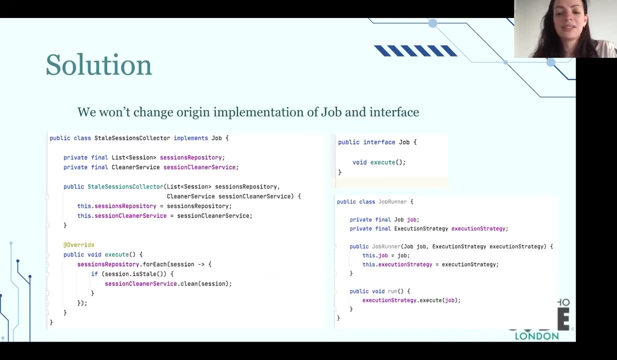 strategy, strategy and the context, and and and- okay the question for you. what is the okay the question for you? what is the okay the question for you? what is the context in our case, when we implemented context in our case, when we implemented context in our case, when we implemented it, what is the context here? 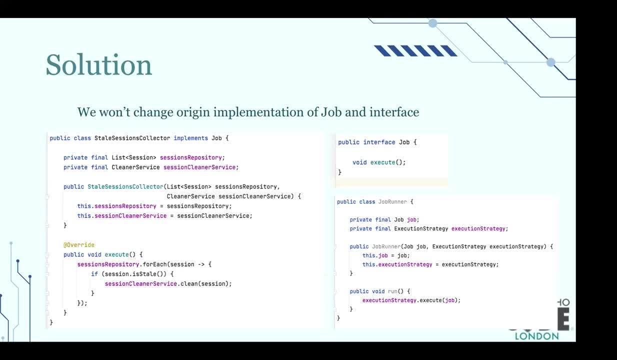 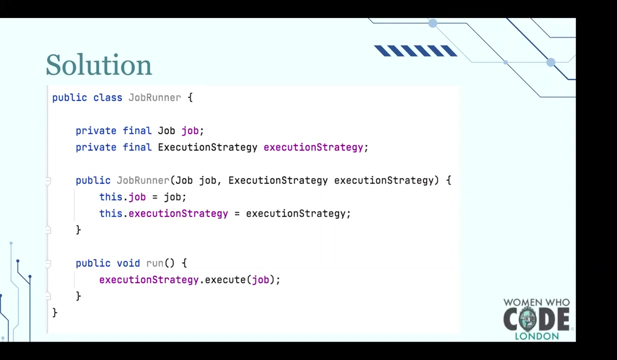 strategy goes into context, strategy goes into context, strategy goes into context. so what is the context here? so what is the context here? so what is the context here? the connection, sorry, the station sessions collector? no session collector, just job. I think execution strategy is the context, no strategy. 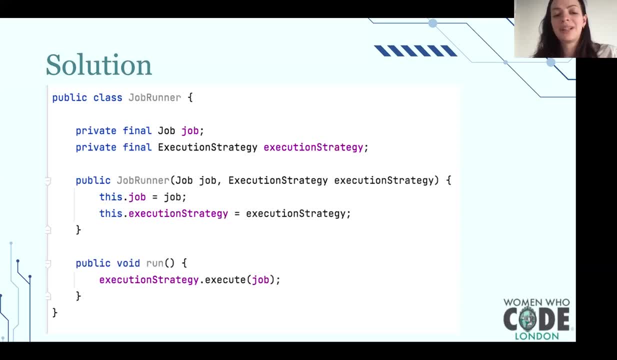 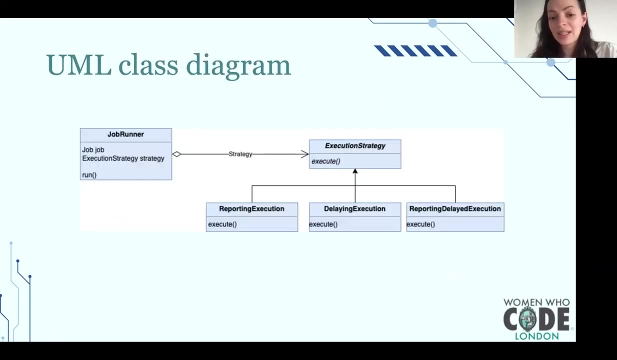 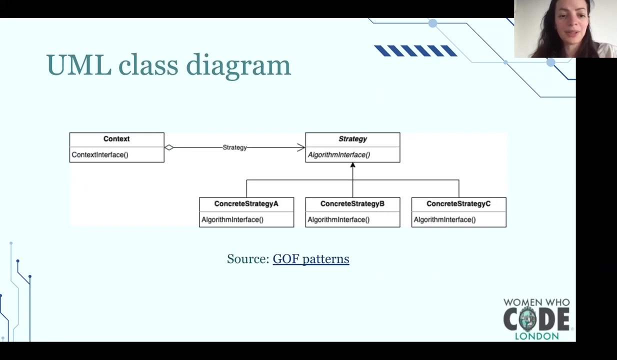 but strategy part of context. so job runner, yes, this is the answer. yes, that's correct, perfect. so in our case, job runner is our context and execution strategy is strategy that can be implemented to be reporting delaying. reporting delays anything you'd like. I wanted to put it here because when you look, 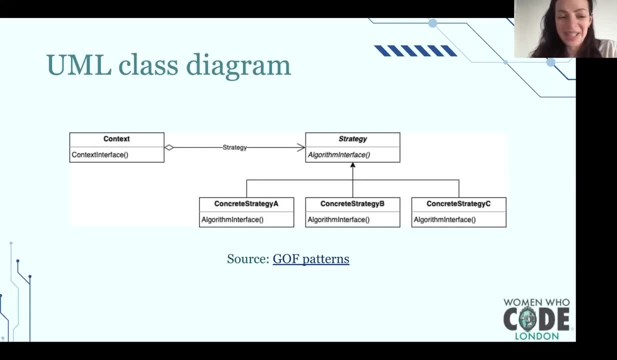 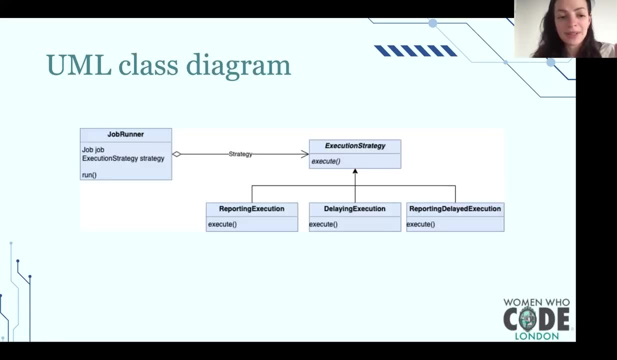 at this diagram, you think: well, really, what is the context? and it's tricky to understand this pattern. but this pattern can simplify your life in an incredible way, like you can start to apply everywhere strategy. it's really powerful and it really makes your code base really flexible. 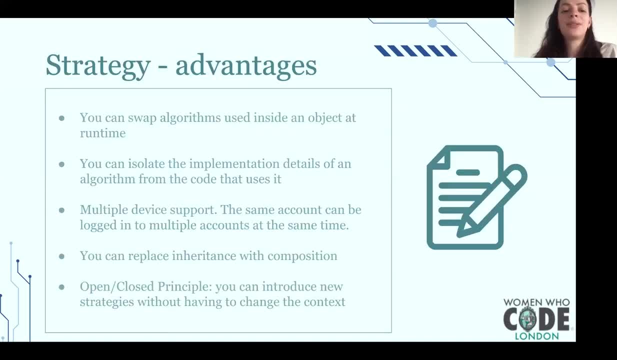 so advantages: you can swap any algorithms. you can do strategy execution with reporting without reporting, delaying everything you like. you can isolate the implementation delayed so we don't need to put reporter at original job because well, job doesn't care about any reporter job, just want to do. 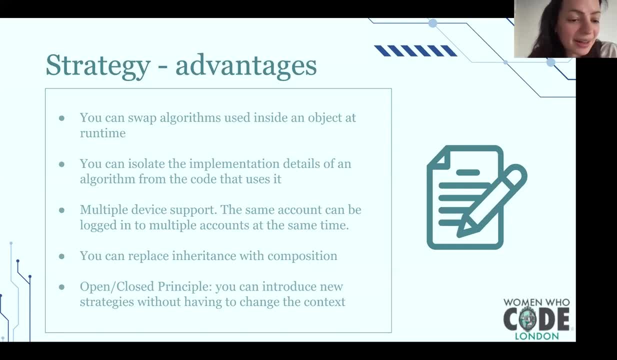 their job, so you isolate them. multiple device support. that means that, uh and Okay, it's about another example. So, for example, if you had devices as a pattern, as a strategy, you can use multiple devices. You can replace inheritance with composition. 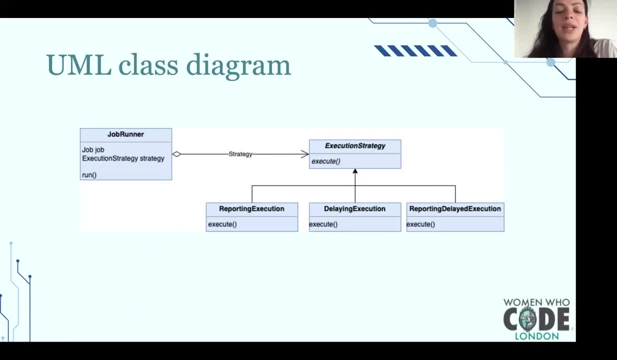 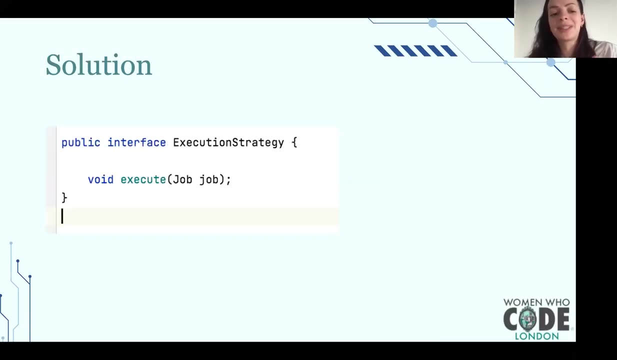 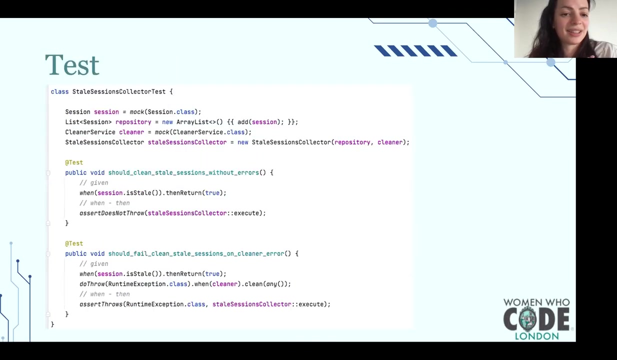 Yeah, what is it about Composition when execution strategy becoming part of your drop runner- And, yes, that's, you could also. Well, there will be. there was another way to do all of these things. Who can provide some idea, like just just here when we wanted to extend our job? 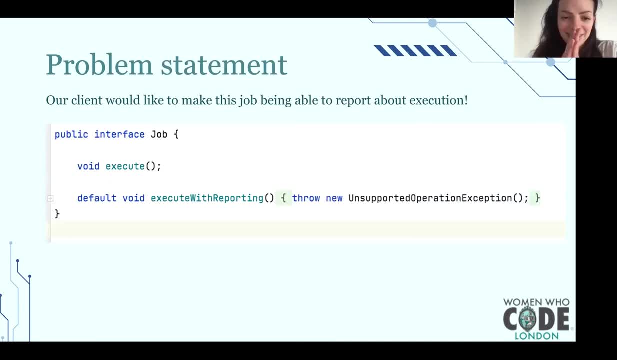 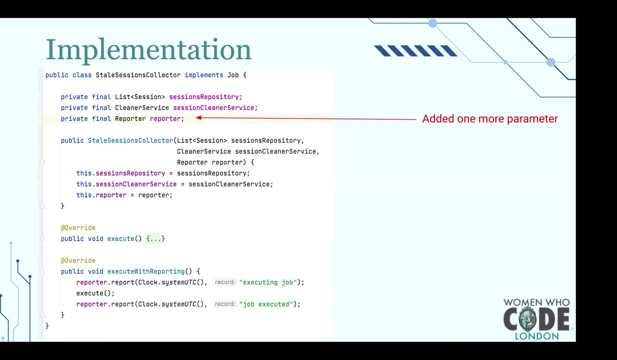 What else could we do? Any ideas like there could be another way. I guess there's also decorators. Yes, that's true, We haven't covered the greatest in this track. We will cover in next session And we touched it a little bit. 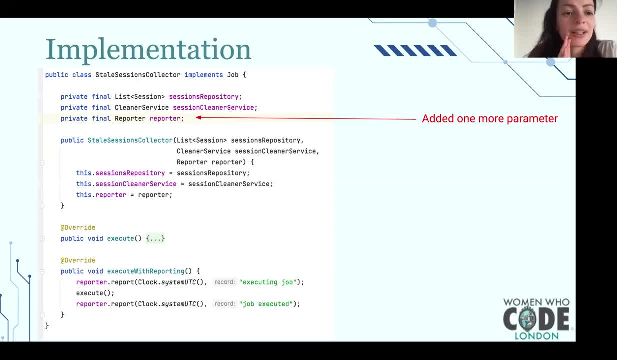 We touched it a little bit in solid principle session. This is true And decorator also a pattern that could allow to do it, And you could extend style session collector to style session collector with reporter And then you could also extend it into session. 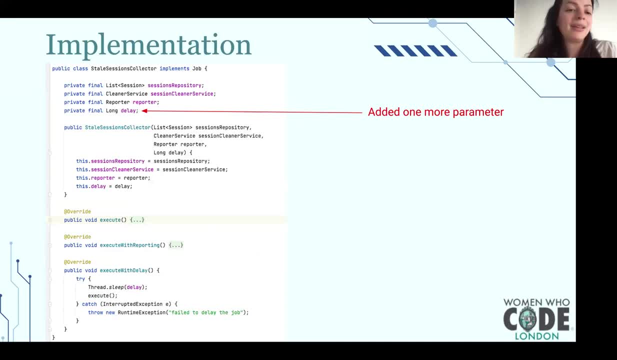 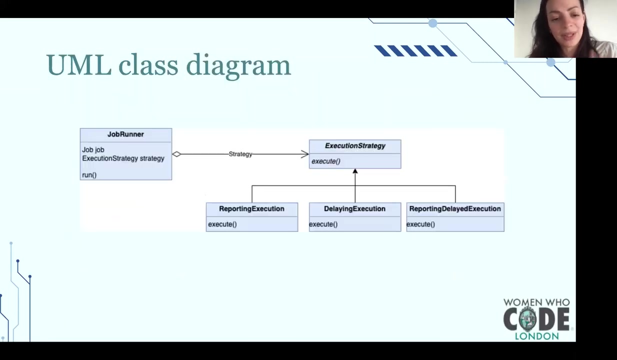 Session collector. delay is delaying extend sale. session collector. Yeah, In this case you just have execute method and you just can do not even override the same method, But you put another method, like you do create stale session collectors. That's right. And if you apply a strategy pattern- why I wanted to do it? because I wanted to say the fourth statement. 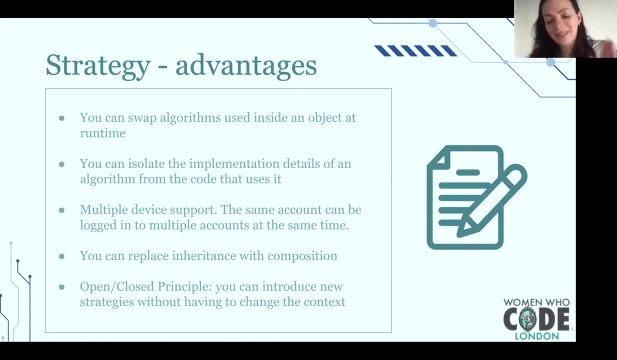 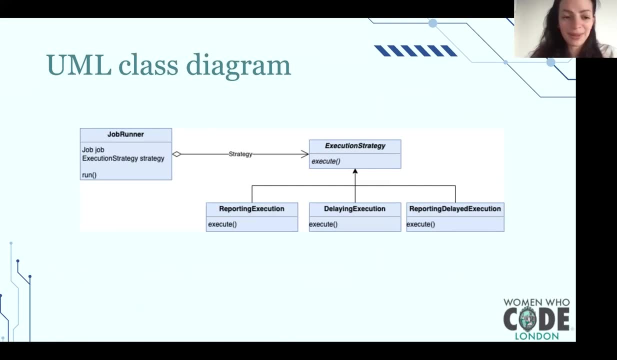 You can replace inheritance with a composition. Personally, I don't like inheritance And also I read in effective Java by blog that inheritance is evil. So this pattern allows you to use composition. You just complete execution strategy in the context, which is job runner. 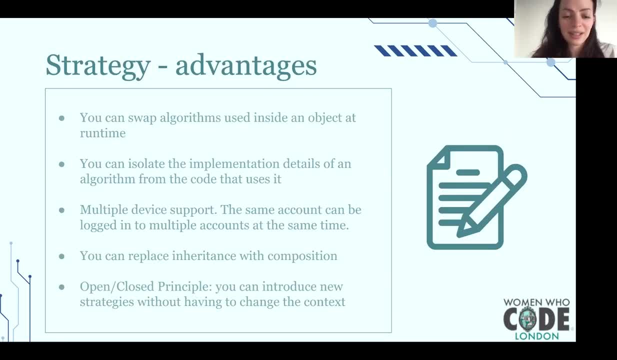 And you don't have all this pain that inheritance Can bring at the end. And the open, close principle, like the implementation of strategy, or basically closed that method to use, it is open. I would say like this: Yeah, And you don't need to change the context. 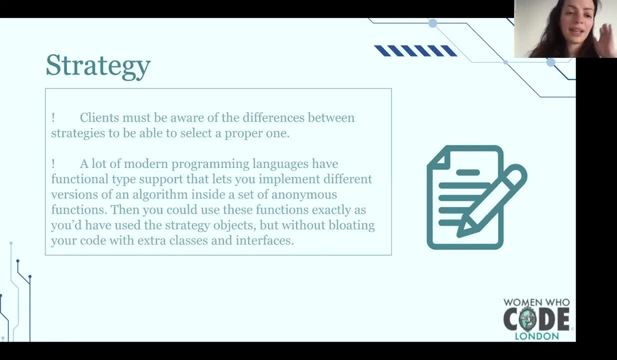 That's also important- And the problems that you can Just don't know that there are already strategies that you need. You just do not understand by the name of the class. So the other developer comes and brings one more strategy, The other developers create three more strategies. 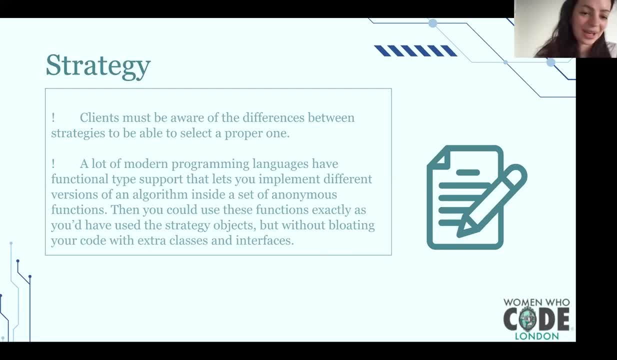 And there are a lot of strategies. Okay, That could happen. A lot of modern programming languages have functional type support. Yeah, So you can use that. You can use lambdas. You can program in Scala without strategy, Because you just create new functions. 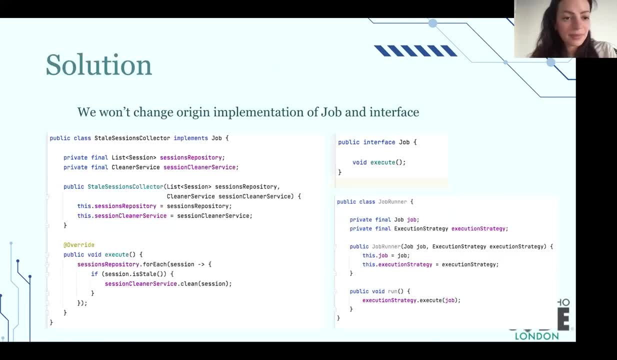 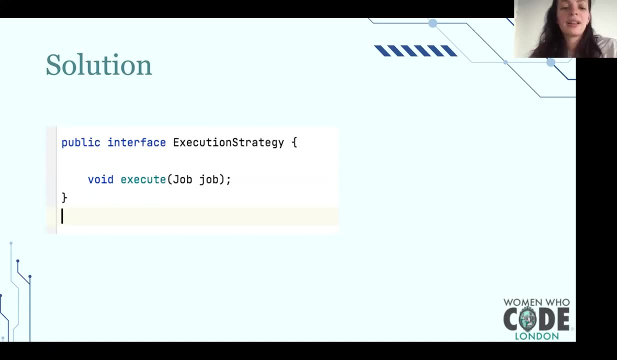 Also, even with strategy, That can became just functional interface, Because we have only one method basically. And well, I wouldn't say that actually this draw Like this is the flow of the pattern. But yeah, If you Programming in functional language. 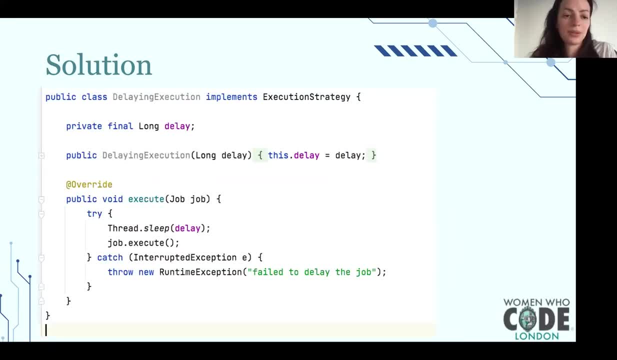 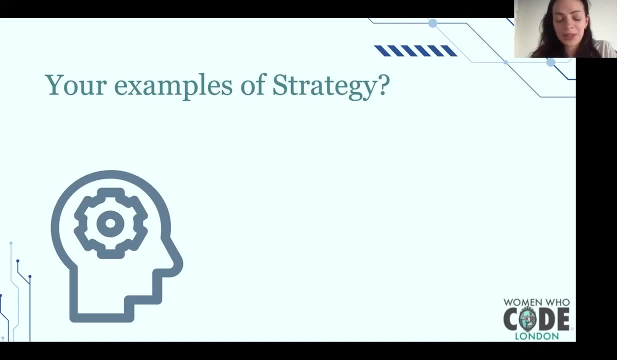 Probably you don't need to use strategy Because you just use your lambdas. Yeah, If you have something in mind, Probably you already meet somewhere in the code base Or some Like 20 seconds, If you have Example. 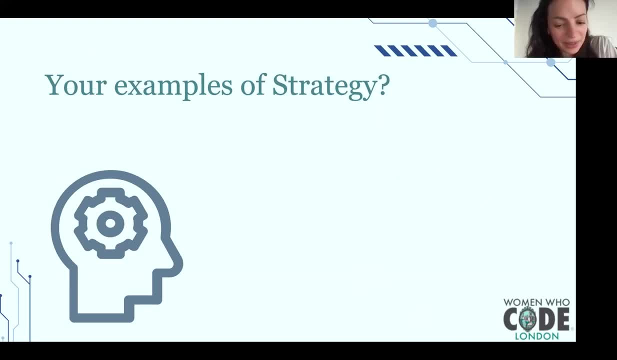 Yep, Anyone wants to say anything? Comparator also Can be seen as a strategy, Exactly. Thank you. Yes, That's true. That's Basically The strategy to compare elements in Collections in Java. Yeah, That's true. 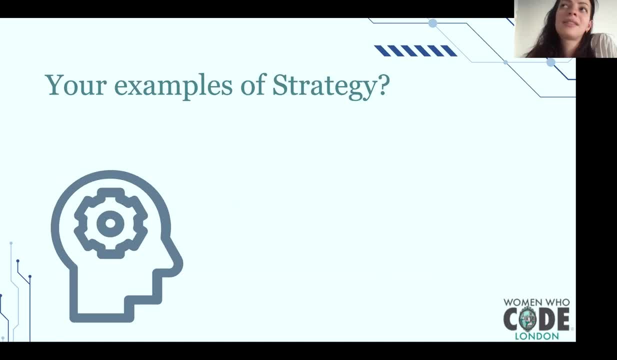 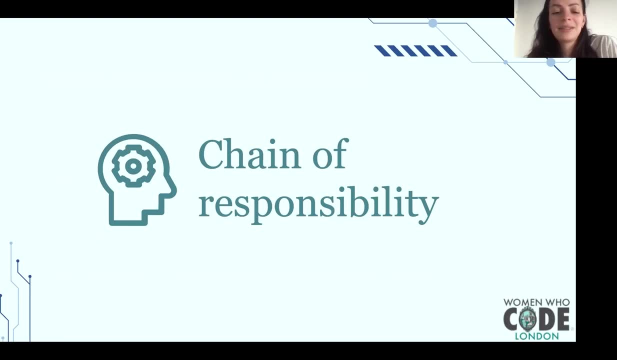 Okay. So Yeah, We have also Channel On object oriented Programming track In our Slack, So Let's share Examples there as well. After this session And next pattern: Chain of responsibility. Well, I would say that 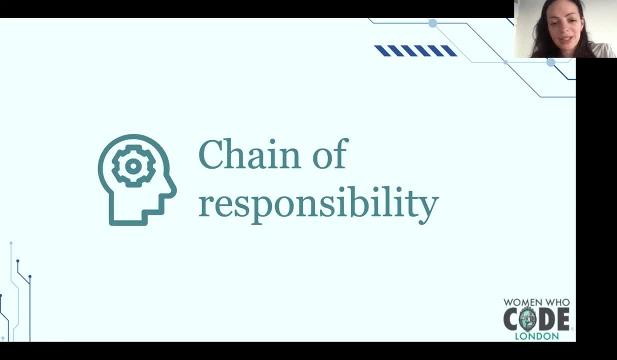 I used it In my experience. In my practice It's allowed me to simplify Code A lot And I will show you Example. It's very close to The things that I did in my experience, So Yeah. 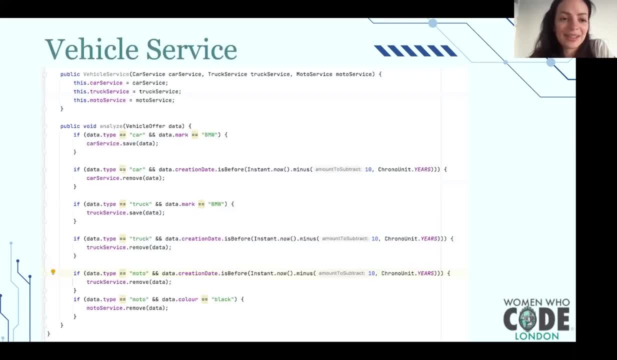 That's, That's Interesting Pattern And Let's look at it. So, Problem statement, Vehicle service. And It's Accept A Problem Statement, Vehicle service And Vehicle Offer. You Can. 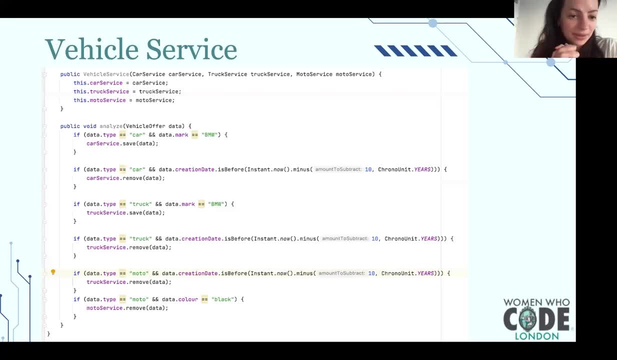 Think About It As A Platform That Accept Different, Different Offers To Sell Them. Basically It's Like eBay, But For Vehicles, For Example. Probably You. 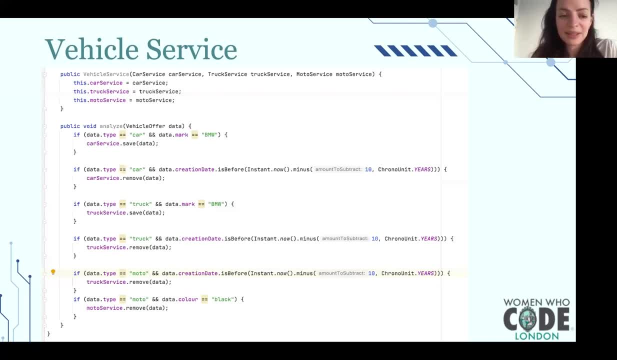 Know Some Country. I Don't Know Exactly, But That's The Statement. Like You Need To Analyze This Offer, You Need To Think About. Like. 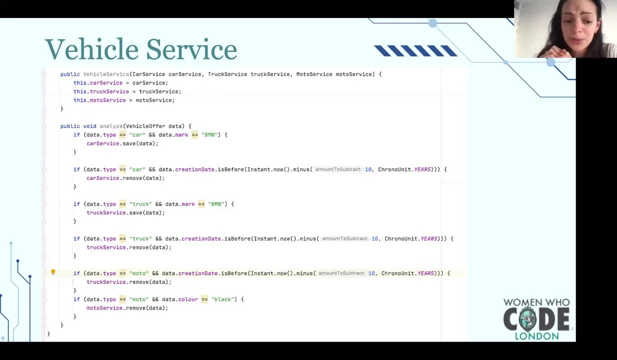 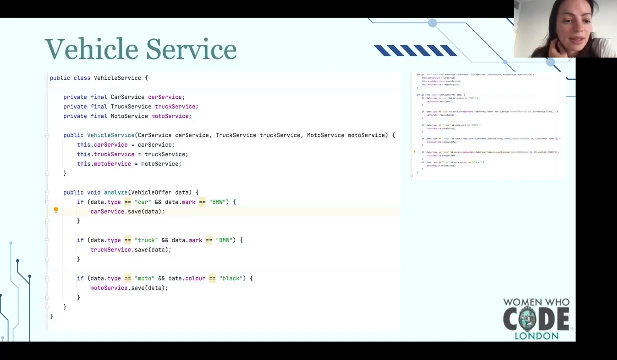 You Have A Lot Of Offers In Track Service, Which Responsible For Track, Which Will Render Them For Tracks, And The Same For Motor Services, And 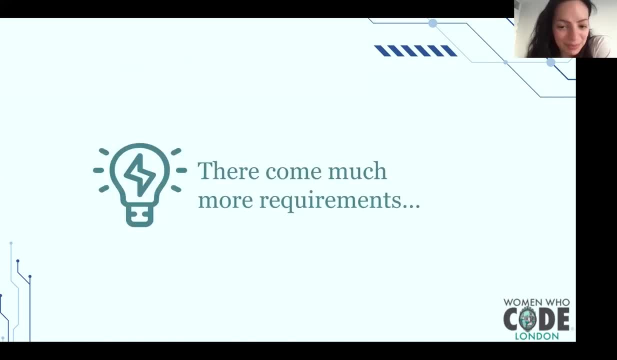 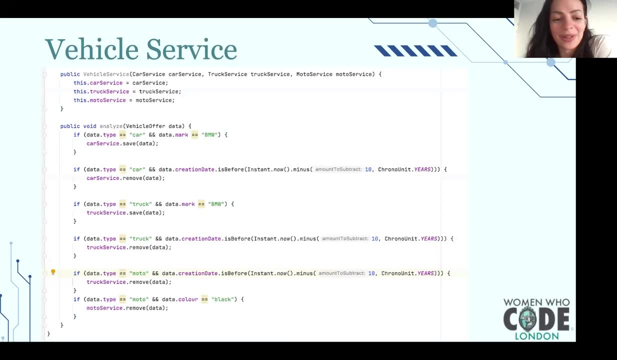 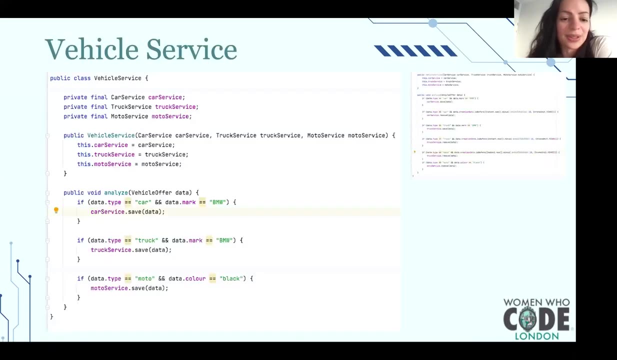 Oh My God, I Think I Changed A Little Bit Different Conditions, Like If It's Car And If It's Being. You Save It Like Was. 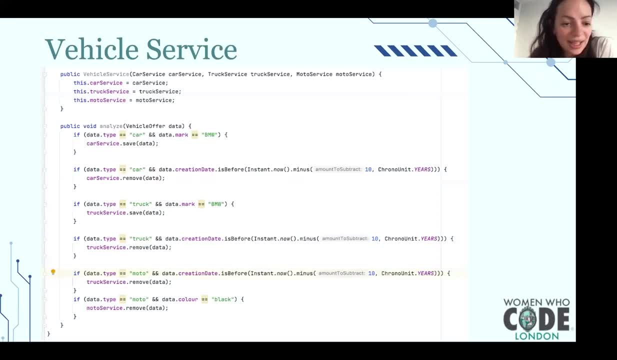 Probably The First, The First Requirement: If It's Track And Being Saved, If It's Deleted, Then We Delete Them If We Have Track And Basically, 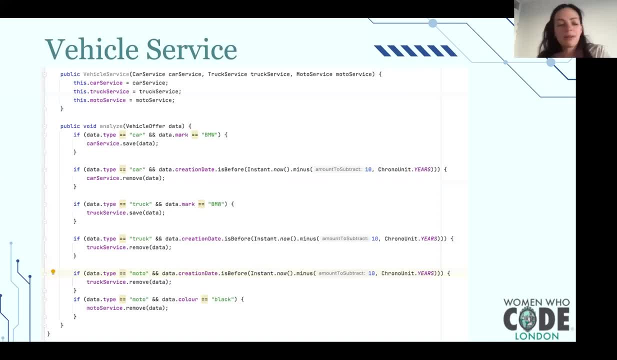 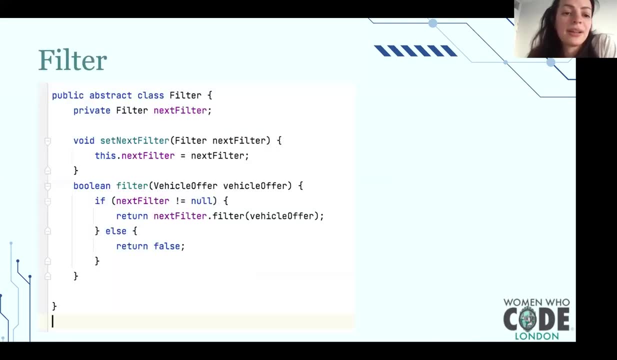 Creation Date Of This Author For Example Five Years Ago. Then We Remove It, And For Motor, For Example. So It's Very Interesting, I Want. 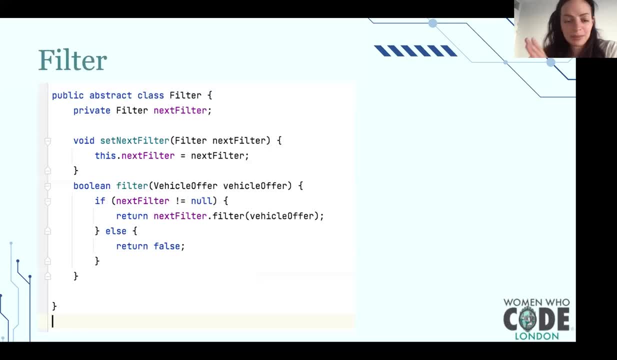 To Create Filter And I Want Also Have Next Filter. Let's Think That The Order Is Super, Is Super Important For Us, So I Want. 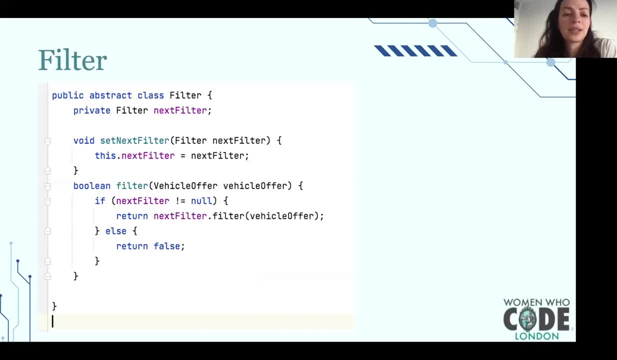 To Create A Interface, Or, Even Here, I Created It As An Abstract Class, Because I Want To Say, Like You Know, This Filter It Always. 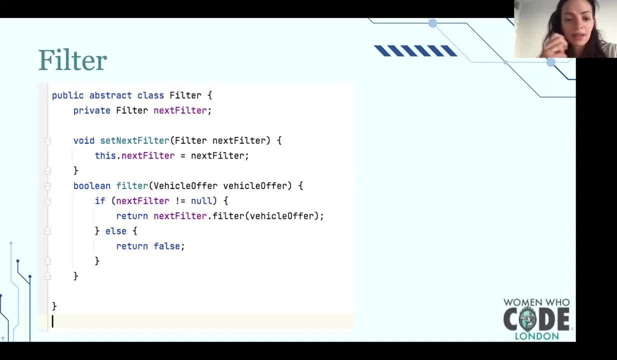 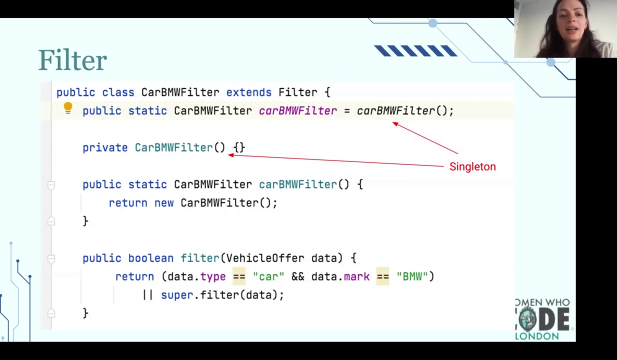 Has Next Filter And And Basically That's It, Yeah, And Also We Have. We Also Have To Apply Our Conditions. What Is Our Next Filter? 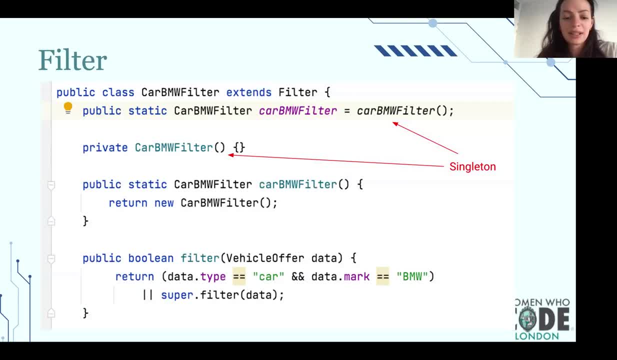 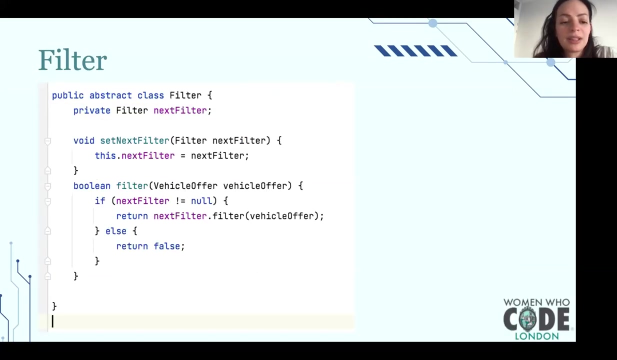 Now I Implement This Filters, So This Is Filtering. Ah Yeah, Okay, That's, That's Right, Everything Is Right. So If My Data Applied, I Return. 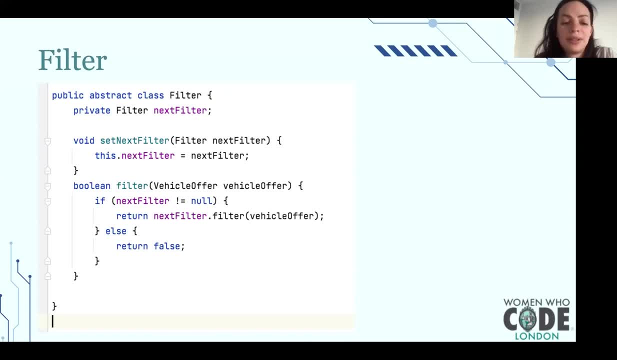 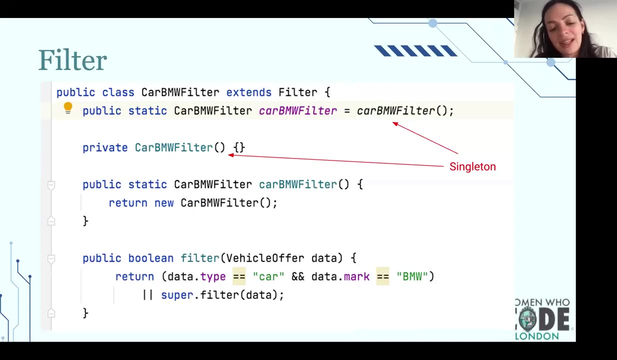 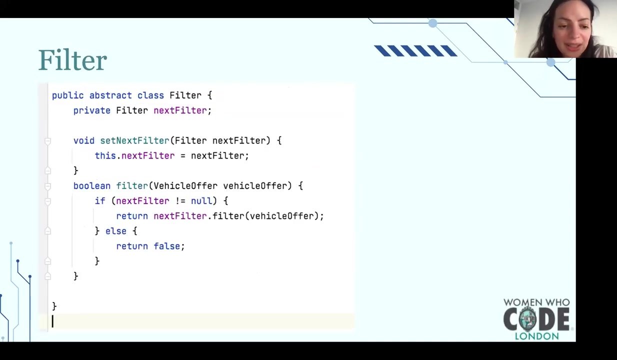 Them. If Not, I Return Filter From The Super Class And I Believe It's Beautiful Like Yeah. You Just Provides Logic For Your Filter And 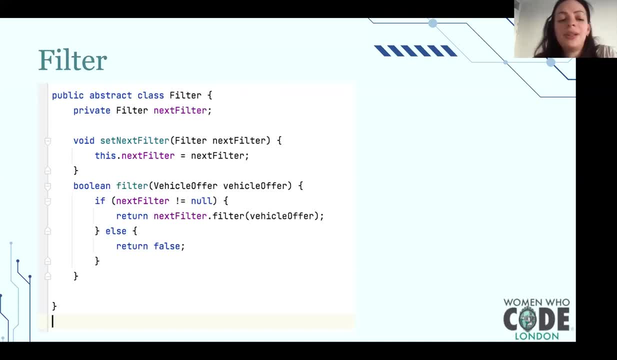 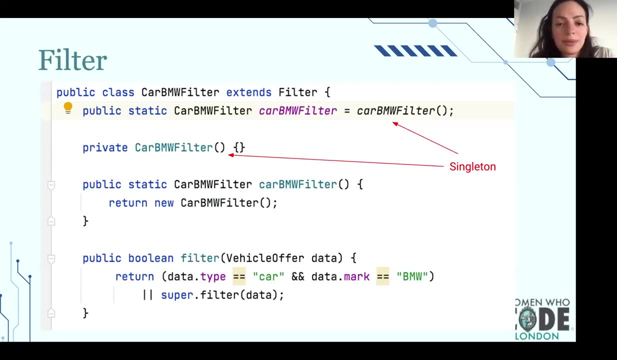 You. Otherwise, You Ask The Filter That Is Super, Super Class Or You Could Create Here, Because You Implement After Class. Yeah, And I Also. I 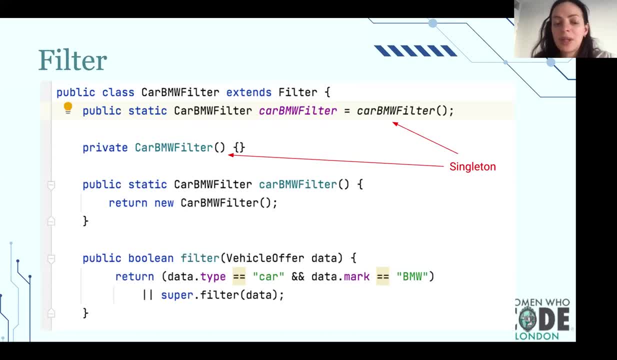 Promise That We Will Repeat Solid Principles And Creation Of Patterns. So Here Is Creation Of Pattern, Which Is To Create A Single Tone With Static. 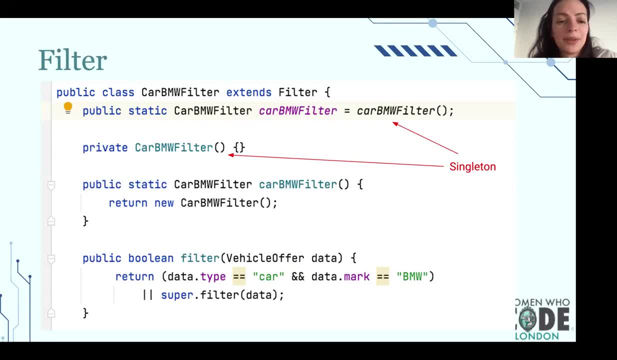 Method And Private Constructor. Actually, I Found This Example In Effective Java By Bloch. And Yeah, You Just Create Private Constructor Which Will Be Public. 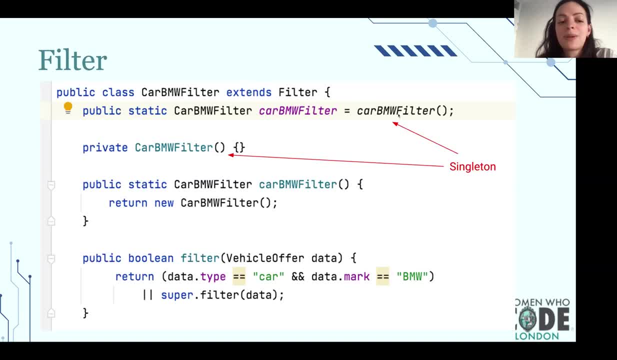 Static Field And You Create Your Constructor. Because It's Private, No One Else Can Access It, And Because It's Static, It Will Be Created On. 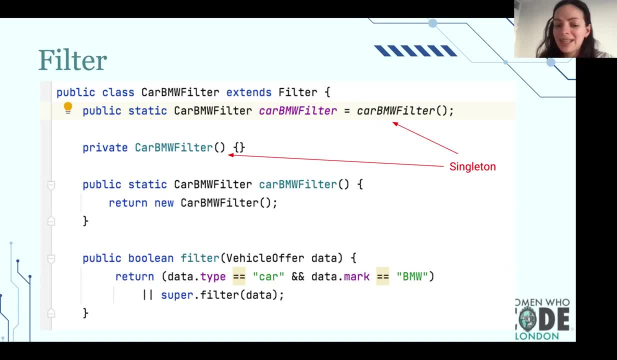 The Class. So This Is How To Create Single Tone: By Like Several Lines, And You Can Guarantee That No One Else Can Create This Class. 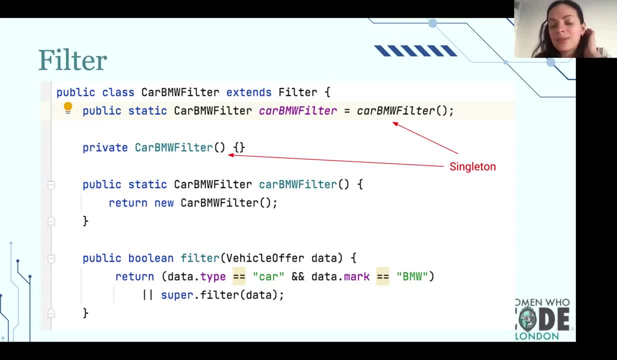 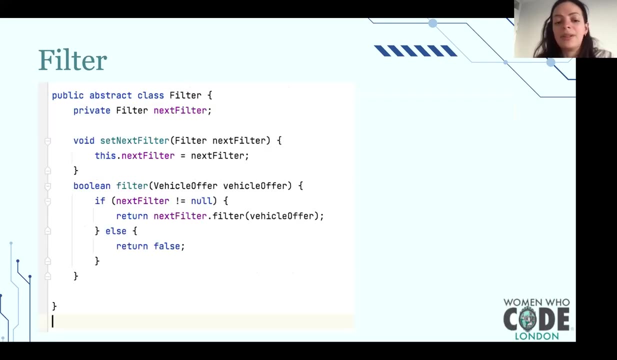 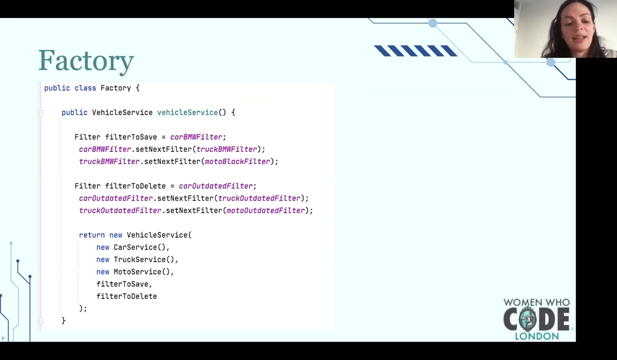 It Will Be Only A Single Tone, And Here I Have Filter Function. As I Already Said, I Have Implementation Of Basically What I Mean By. 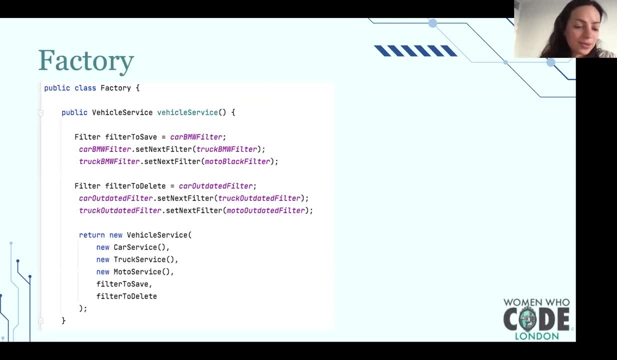 Filter And I Post On It To Delete And Filter To Save. Basically I Said There Are Next Filter. First Of All I Say That Filter. 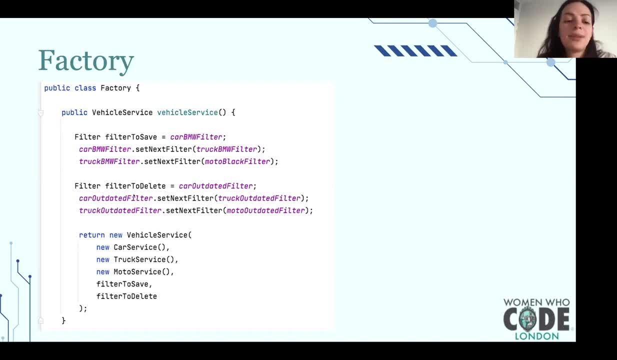 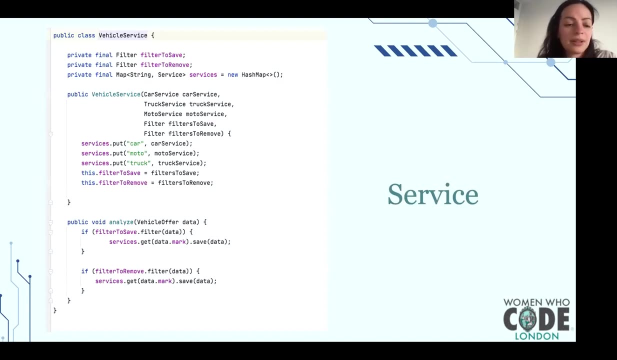 Car Being, Then Second Next Filter For Truck Being And Data. And That Is It Now. That Is How Looks My Vehicle Service After My Refactoring. 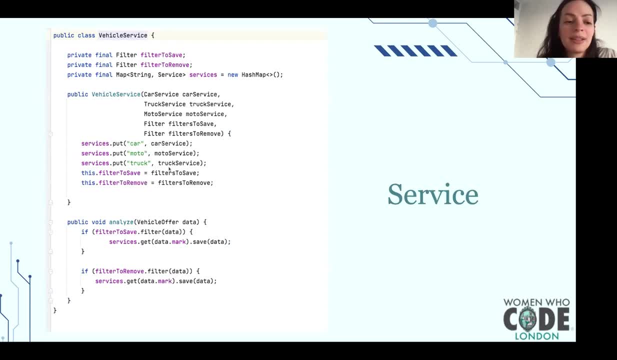 I Also Did Some Trick Here. I Said Like: Okay, I Already Know, That Is Like I Would Filter Data And If Filter Applied, I Saved. 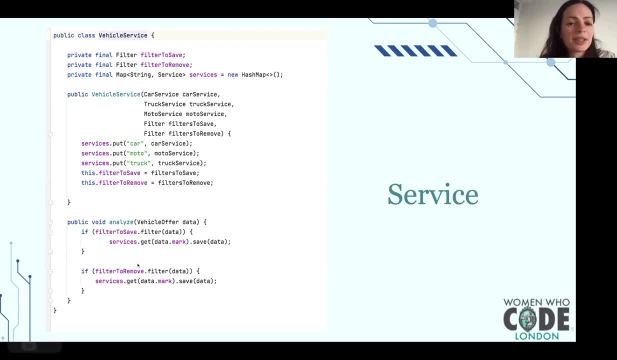 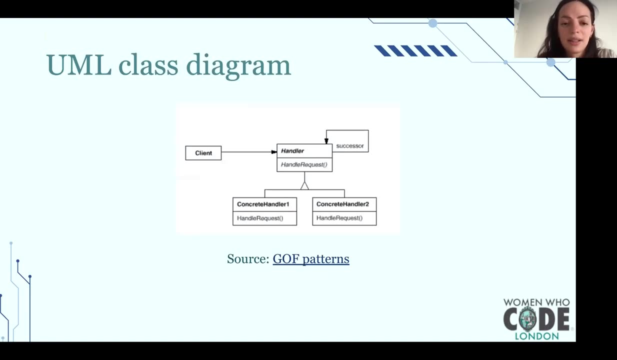 Which Service? Well, It Depends On The Mark. I Just Get Mark And Save It In The Class Diagram. So What We Are Doing In Chain. 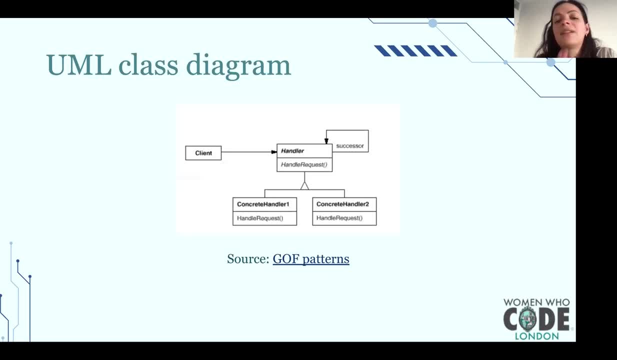 Responsibility Pattern. Basically, My Filters Are Handlers And I Have Handler As An Interface Or Abstract Class And Contract Handler To Which Is Track Filter And 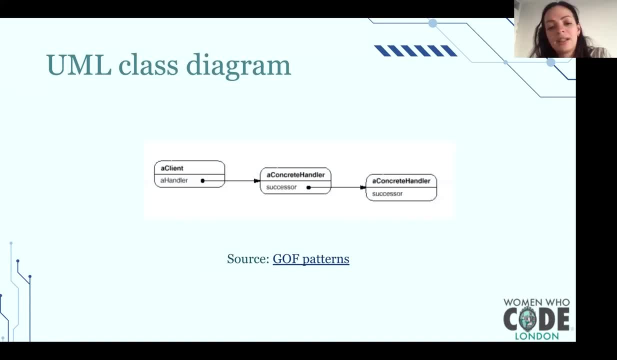 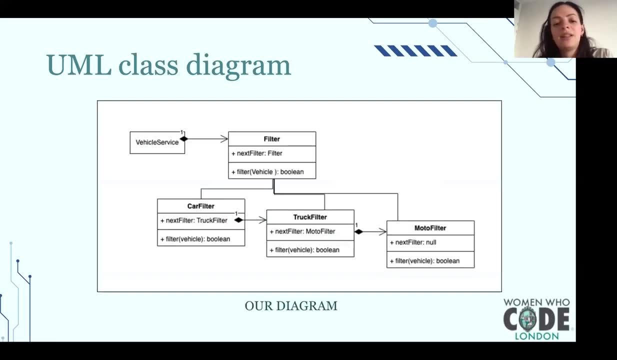 My Client, It's My Vehicle Service, Yeah, And Also These Handlers. They Have References To Each Other And If I Have Different Implementation, Which Applied? 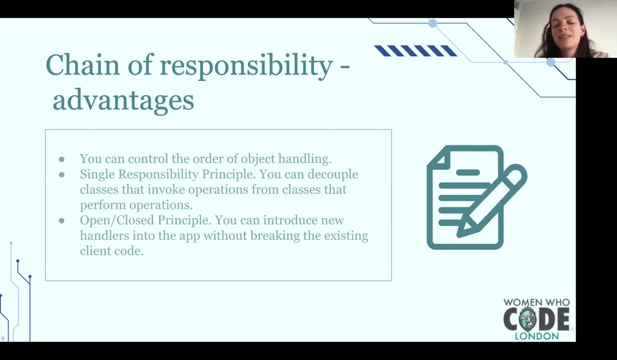 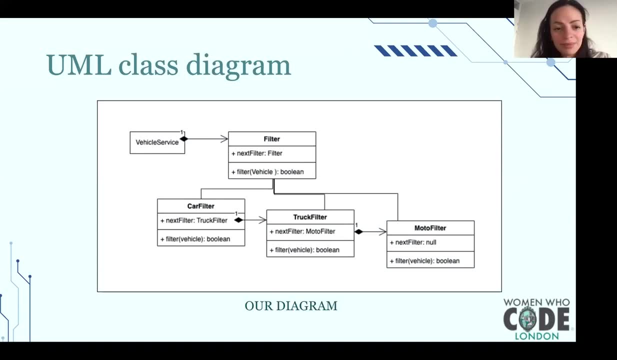 One By One. Okay, Who Can Tell Me Where It Will Be? Even More Efficiency. If You Have Any Idea Like What Else You Can Do. 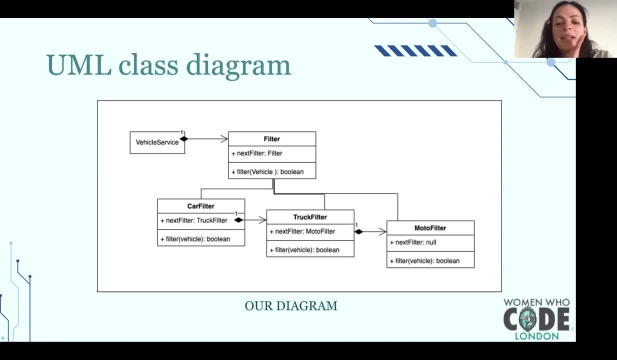 I Would Say That It's Very Powerful When You Really Need Strictly To Apply Different Changes. For Example, You Have Authorization For User If You. 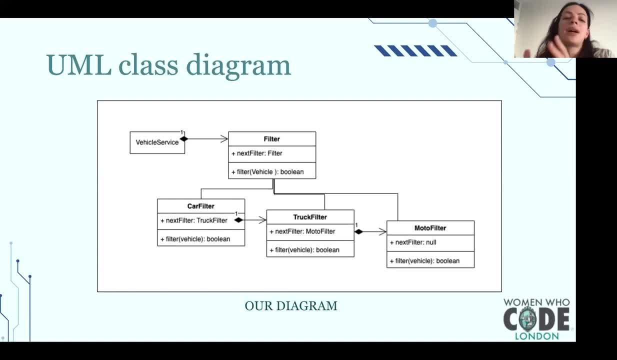 Will Google For It Authorization And To Go Through Two Steps To Verify User. They Need To Do A Lot Of Steps And All The Steps. 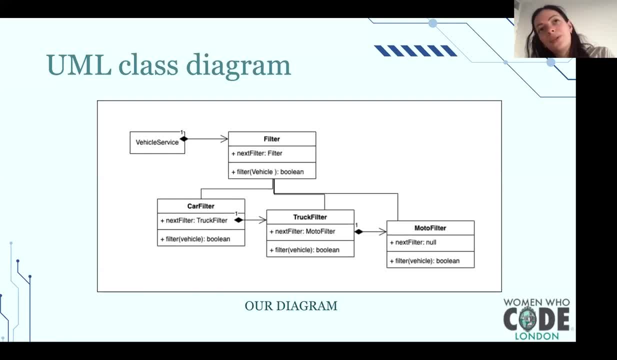 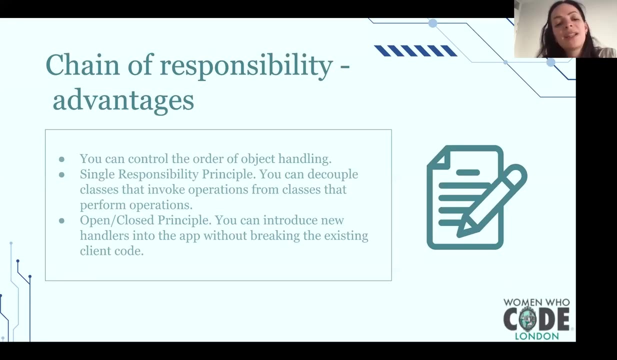 Can Be Part Of The Long Chain If You Use Your Went Through All For All These Steps Chain Of Responsibility. So Advances Is That You. 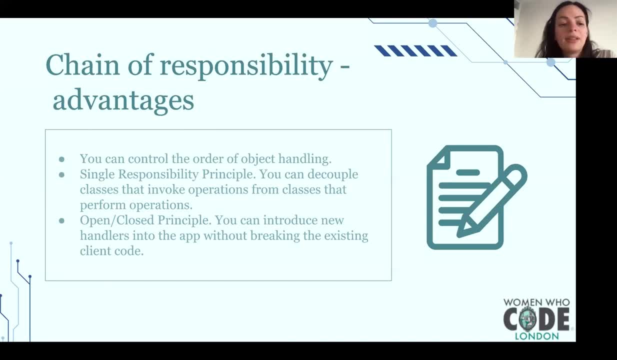 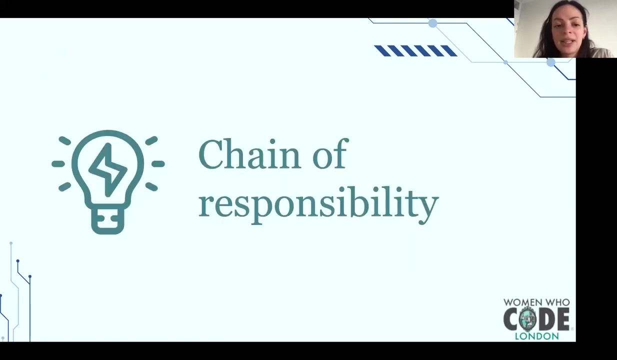 Basically Control The Order. You Can Strictly Say That This Is A Step Of Operations, Often Close Principle. You Can Introduce New Handlers And You 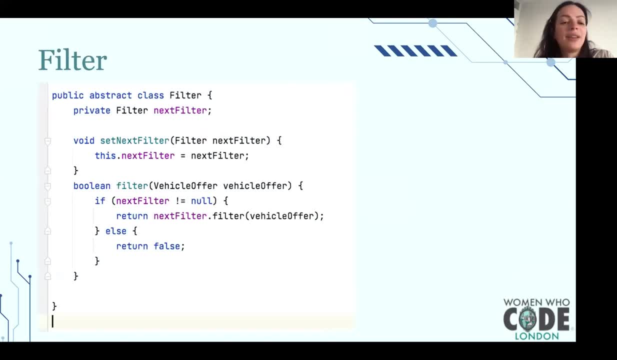 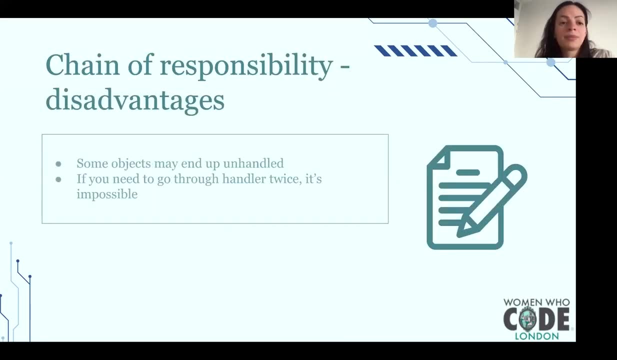 Don't Need To Change Anything In Your App. You Just Put New Filter, New Handlers, For Example. Some Of Us May End Up Unhandled, Like 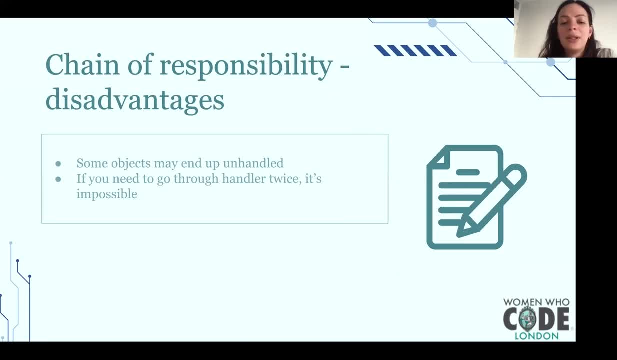 They Dropped At The First Filter, But Basically They Couldn Be Dropped If They, If They Need Another Filter, And With This Pattern You Can't. 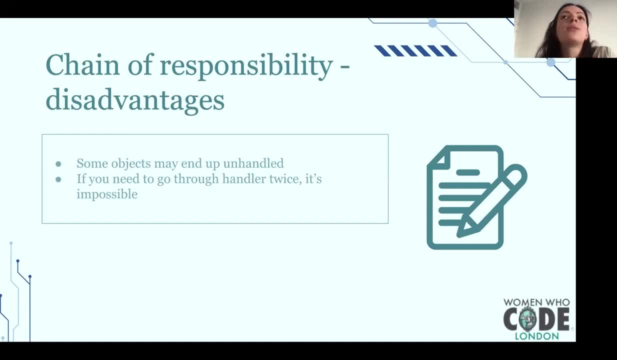 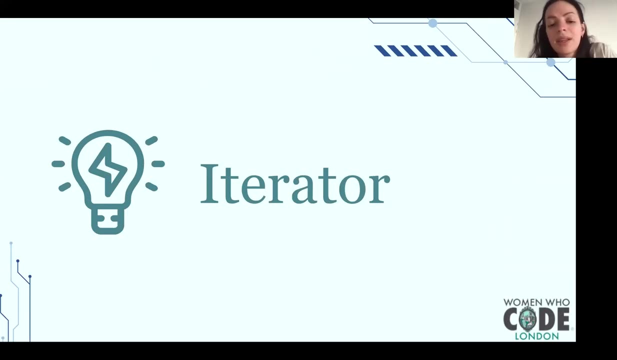 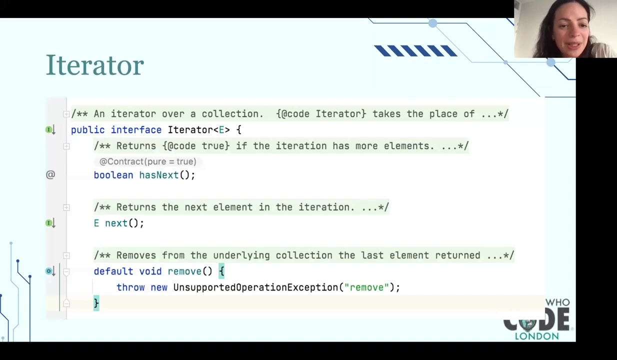 Go Twice Through The Same Step. You, Or You Need To Put It As You Need- To Create Always A New Filter, If For People Who 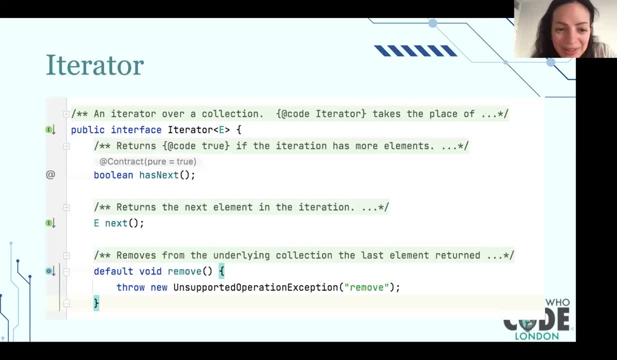 Are Familiar With Java Because We Have Implementation Of This Pattern Exactly In Our Java Utility Library And Almost Everyone At Least Once Heard About. 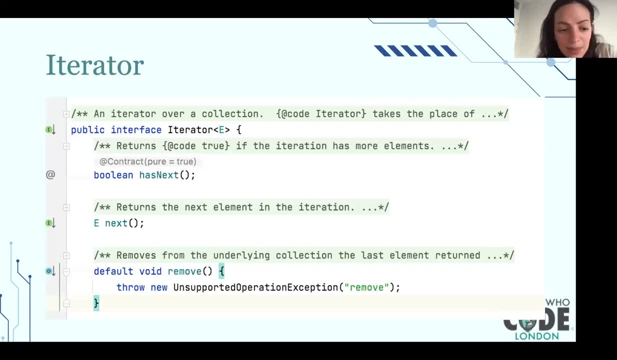 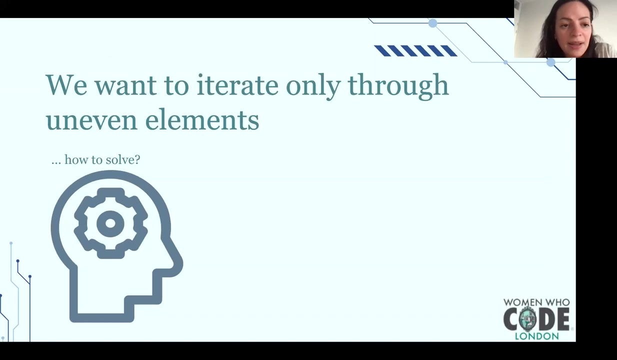 It Has Like Has. Next Method: It's Allow You To Know If You Have Something Next In The Collection And Then If You Aware That. 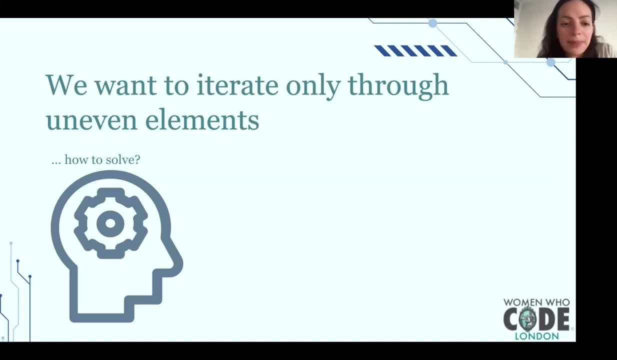 There Something Next You Can Go To This So For You To You Know What Is It Is. This Is A Kind Of A Strategy, Maybe. 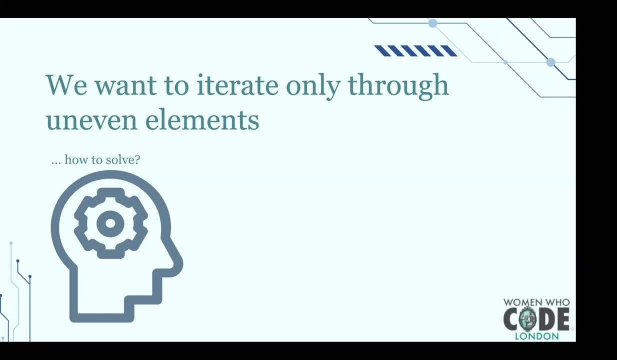 We Have. They Supposed That We Have Inter Int Implementation, extra behavior which we would like to add. So I would say that we need a context and we will have some in that context, some kind of execution. yeah, 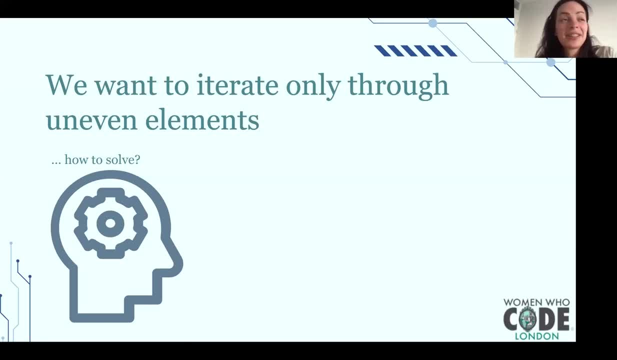 Okay, that looks interesting And, as I said, as only your variable strategy pattern, you would like to use it everywhere. Believe me, that's true. And yeah, it's the first idea to use strategy. This always happens with people who learn strategies. 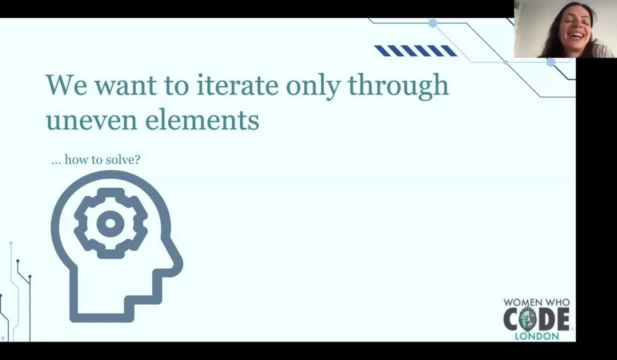 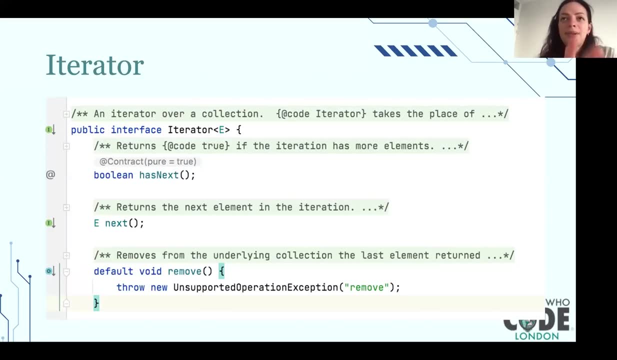 They want to apply them. it's everywhere, Okay, well, not exactly. We need to implement the same behavior of the iterator. So, basically, the pattern will be the same, but we need to go just next And we need to check if it has next. 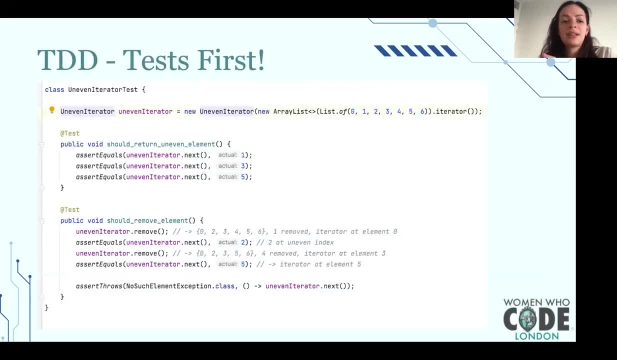 but the thing that changed that we need to go two steps instead of one steps. And let's start with TDD. Well, I love this task because I even was asked in an interview. at interviews, they asked me how to implement an event iterator. 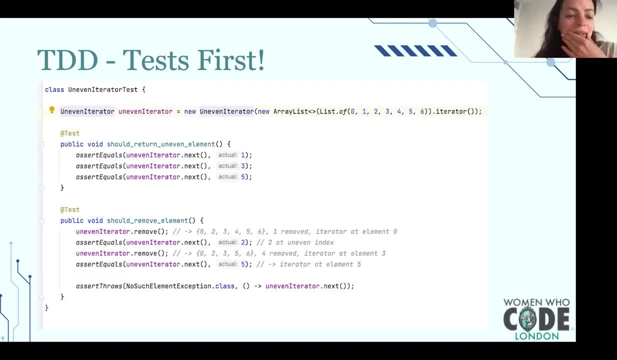 And let's check how we would like to do it. What exactly is the behavior? What do we want? What are the parameters that we are going to see at the end And we say that, okay, we have this, an event iterator. 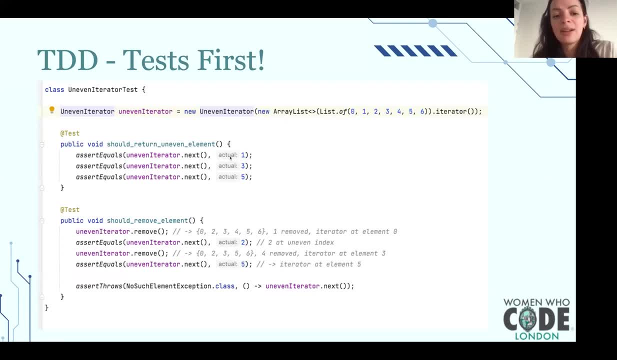 And when we get next method- we wait that- we will go at the position of one. If you will use just a regular Java iterator, you will be on the position zero. So zero one, two, three, four, five, six. that's you. 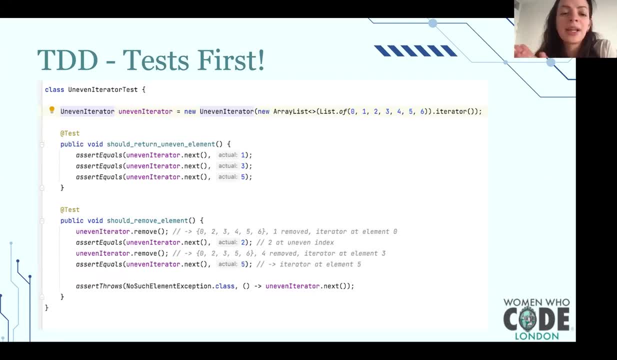 That's something that that you know. that's a good thing Java iterator will give you. But here we want to be at the next position, at first at one and the next at three and the next at five. That's what we expected. 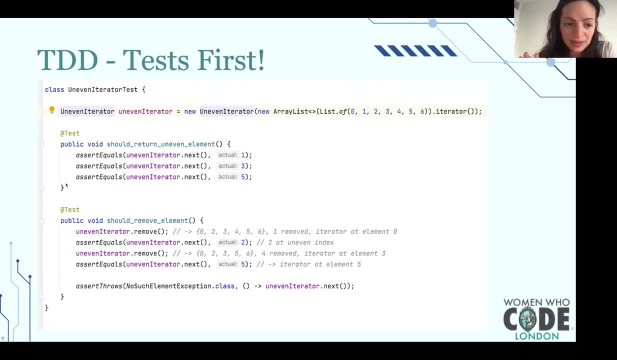 And we write tests, like you know. this is what we expected. Should return an even element And also we want to remove element and that's also should be an even element. So I put comments here. So if you remove, we expect that you remove. 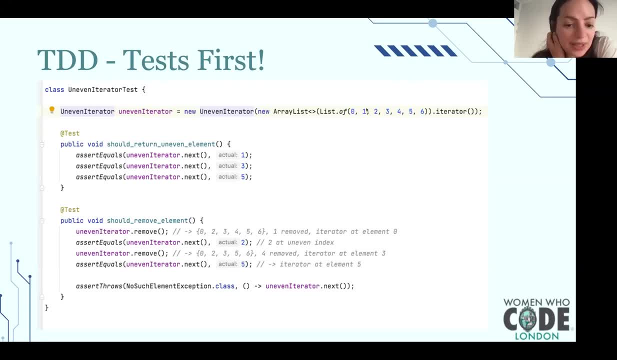 not the first element, but the second. So you removed one, One removed and iterator becoming at the previous step. So it's at the element one, And now, if we want to go next, we do again two steps. So we be coming at an even index, which is three. 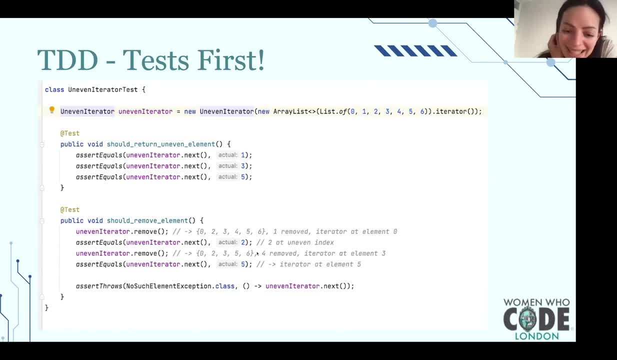 but the element is two And yeah, if you remove again, we remove exactly four, because again we do two steps, because every time be on an even index, And we remove four And in this case iterator at element three. 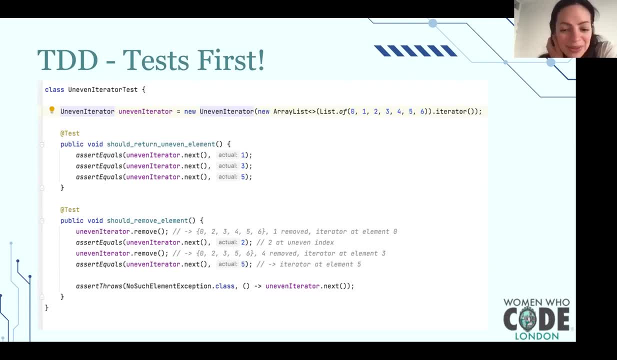 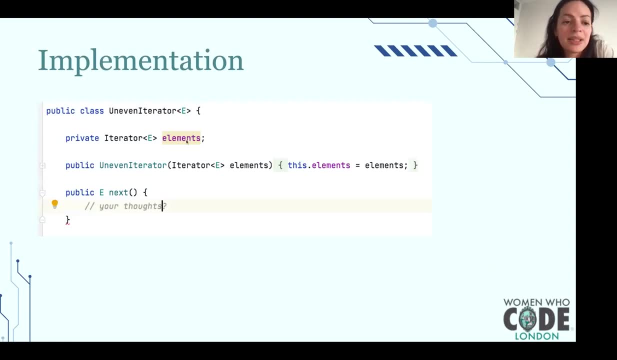 So I will send you a presentation So you will be able to go through it again And let's look at implementation. So an even iterator, we can use iterator there. but we will do some tricks, Your ideas, how we can do it by two steps every time. 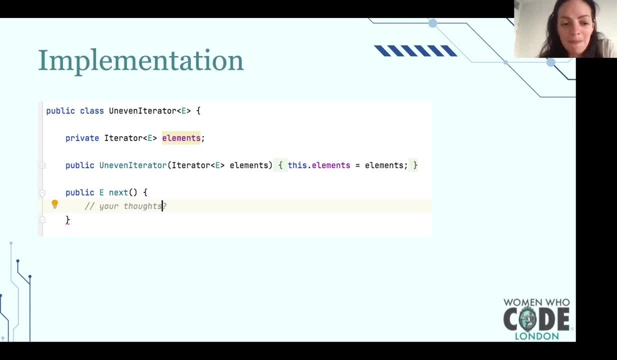 Well, the trick is simple: We just do two steps. We check if elements which already iterator has next and just do step, but do not return element. If there are no element, we throw no such element exception, Because this is basically what we are going to throw. 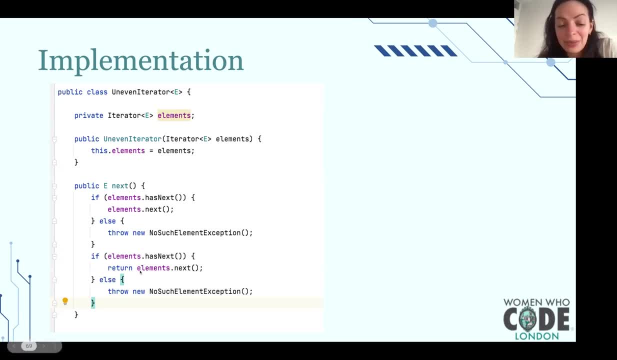 And then we check again. So we have two steps And that's it. We just do two steps but return on the second step. In this case we have an even iterator, So we can be sure that we always go through an even elements. 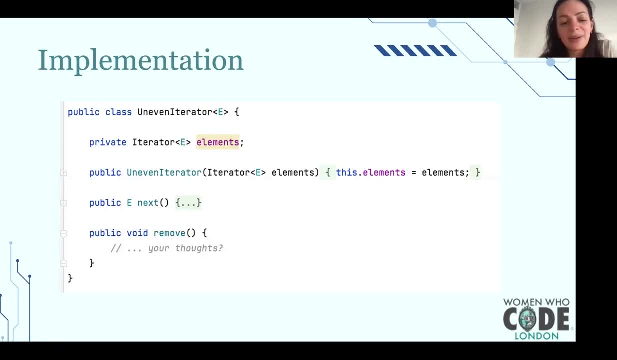 Now, Now we implement it. next, How we would implement remove. And if it fails for remove, what do you think? Can we remove the first element from this? But in this case we will remove just the same as iterator remove. Well, actually, there are no pit fails and it can be the same with that next method. 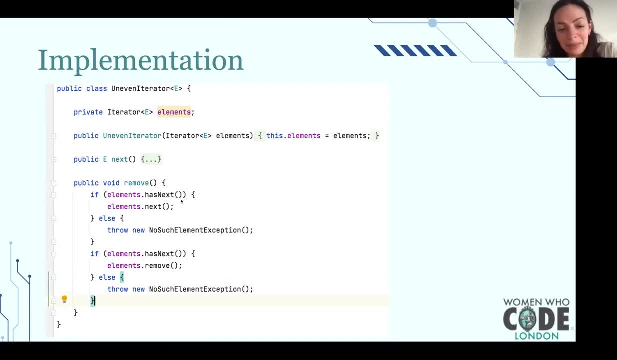 We just check if there are next element, Get with element But do not remove it. We just go again And again we check if there is next element And then only then we remove it. So we just do extra step in the first element. 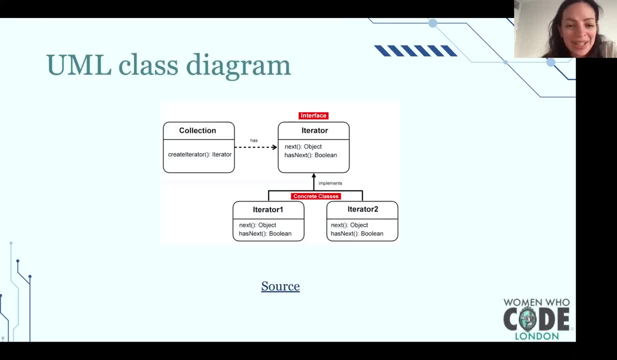 And that's it, And it will work. I checked my test. My tests were green. Yeah, So how it looks like for the first element. Yeah, So you have the diagram. So you have iterator, interface, iterator, first implementation, second implementation, and both of them has next and has next. 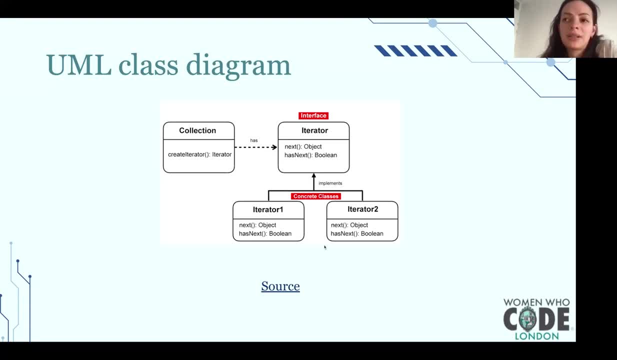 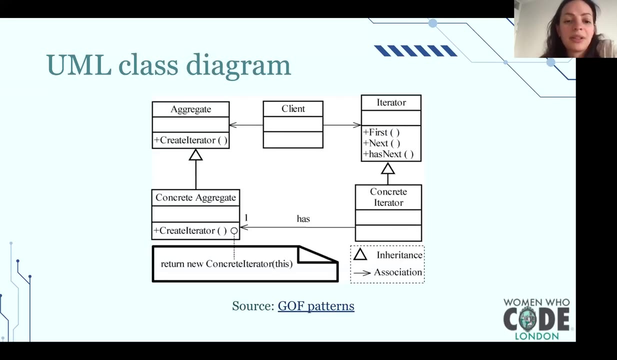 If you check all these iterators that Java collection have, they have implementation as inner classes And you put them in some collection. basically Yeah. So if you would like to look at how we would use them, we always have clients that have iterator and aggregate, which create iterator. 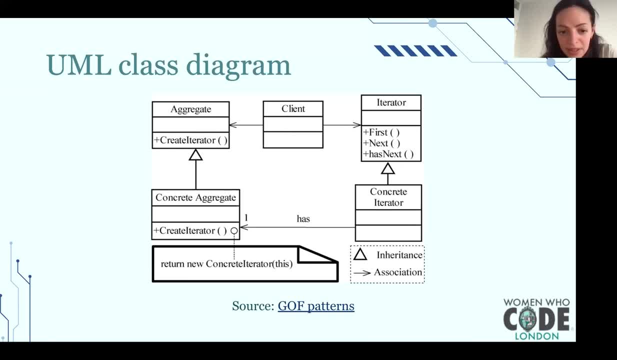 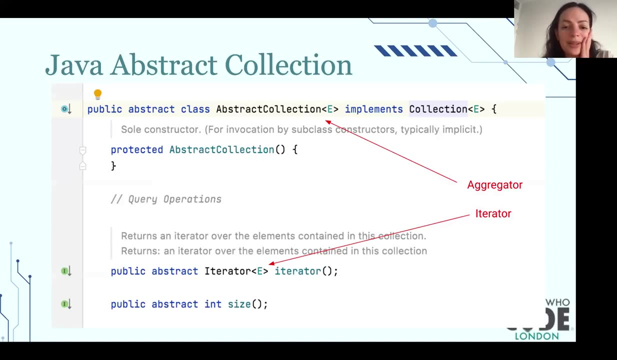 Yeah, If you check libraries in Java like ArrayList, LinkList, you will see how this pattern by these diagrams And I put it here. So in Java you have abstract collection, This is aggregator And it has iterator inside as composition. 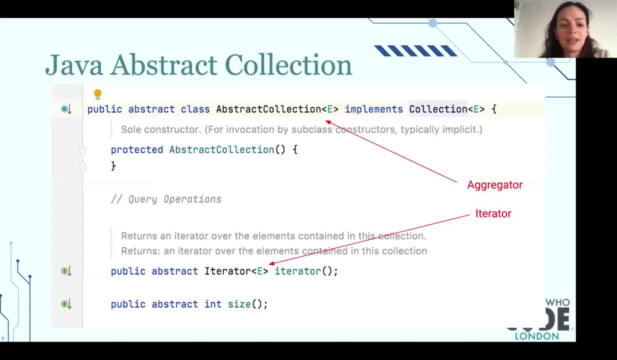 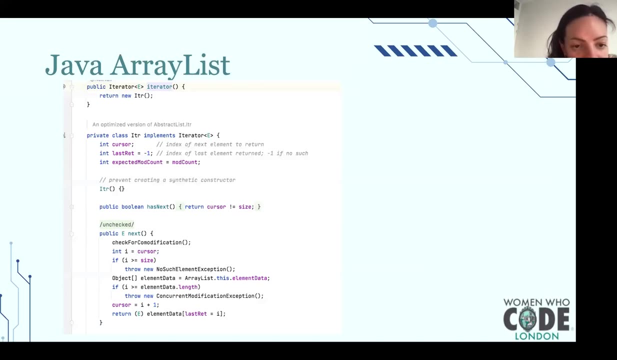 Yeah, So what we can see here is the same And yeah, So basically in this abstract collection we create iterator. Yeah, And I put the example here. So this is Java list And this is what we can see for implementation of iterator pattern. 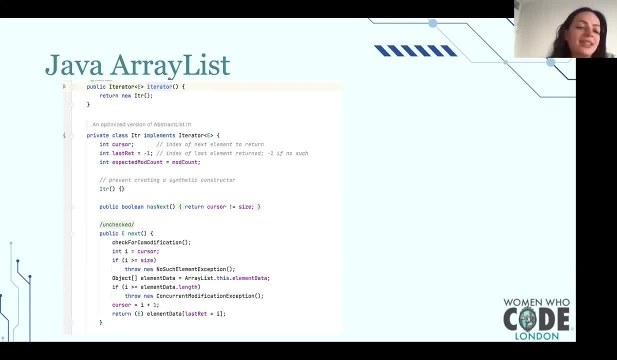 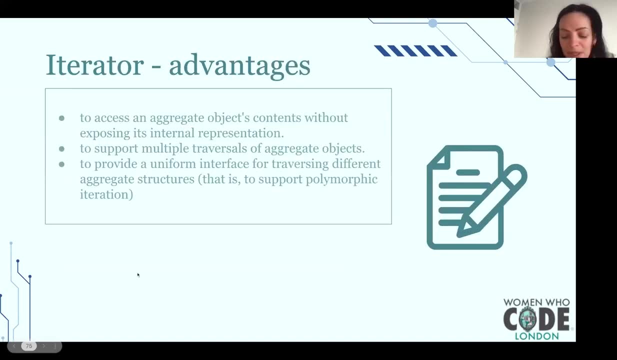 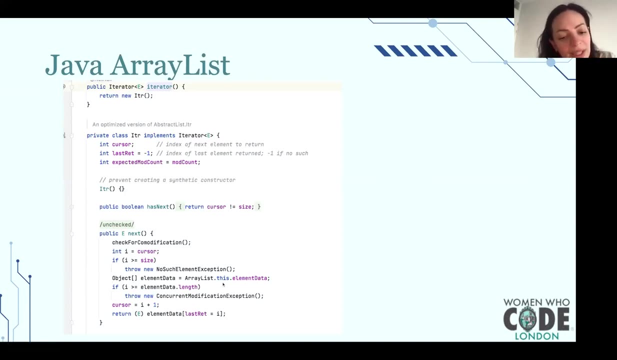 So basically, Java list has array under the hood, So iterator goes through this array of objects. So if you look at the line here, this object with array- You will see that this is basically the collection that we are going to iterate through. 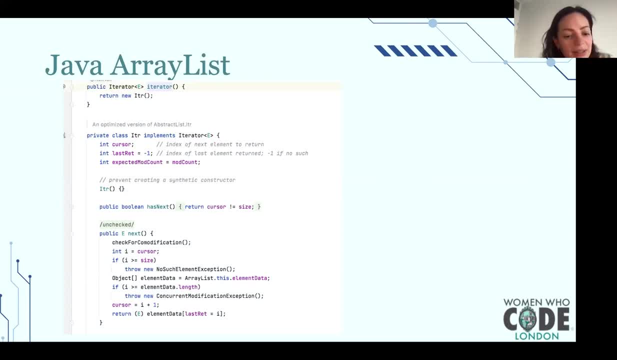 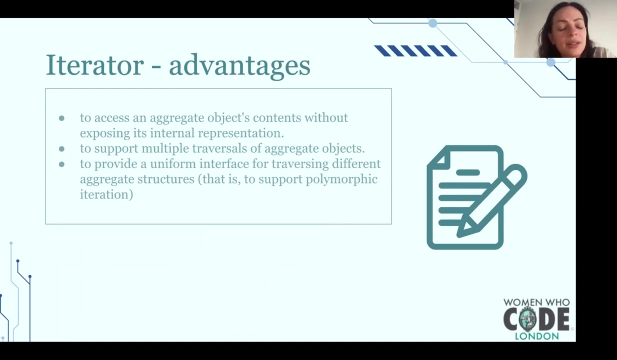 And it trying to do here just full cycle But return next element by the next index And it has indexes like the cursor inside. So this is how iterator implemented in Java. So what is another use? You can use iterator if you implement some map interface. 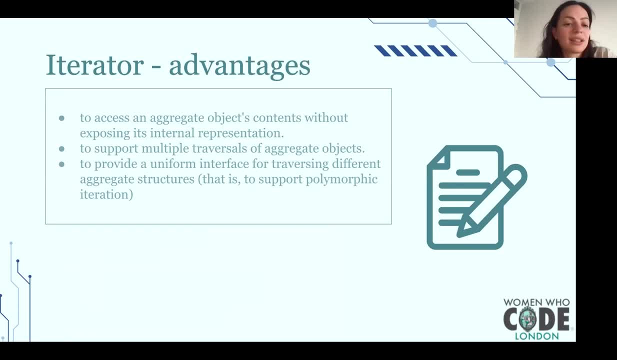 And you would like to provide the next step for your traveler. So traveler just need to get next method And that's it Like yeah, you can imagine you have traveler And it looks like this And it only check if it has next location to travel there. 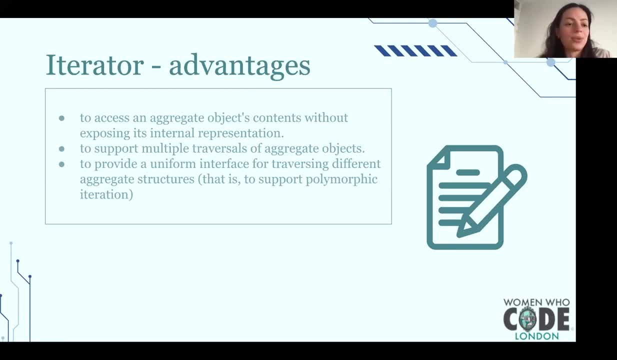 Or it already went through all locations So can go and sleep And if it has next location it just go to next location. That's it, So you can support multiple traversals of aggregate objects. Aggregate objects is your collection. Multiple traversals means that iterator and uneven iterator. 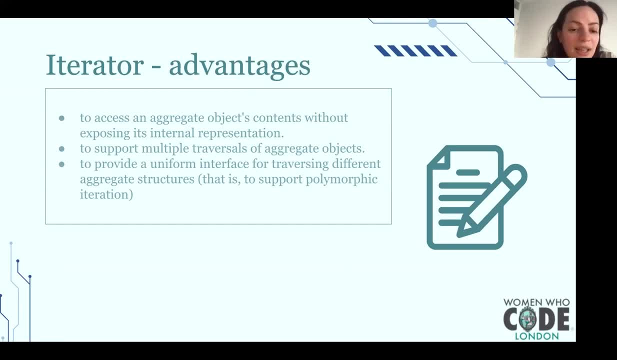 You can have also uneven iterators And idea of this pattern to provide uniform interface for traversing for different aggregate structures. And that's basically what they did And that's basically what Java used. Java used this uniform interface And disadvantages. Blind with pattern can overkill you. 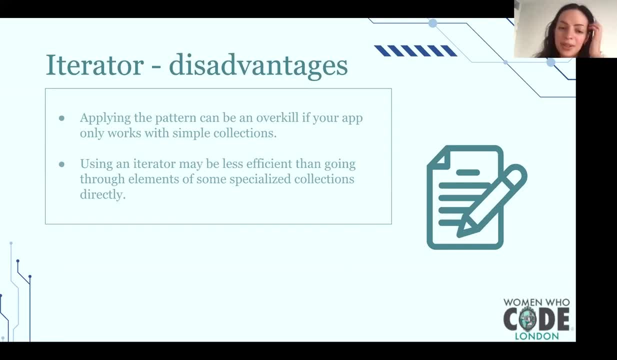 Because, yeah, if you have just simple collection, maybe you need just iterator that already implemented And also collections by default. they have some optimizations, So probably it's always better to get already implemented iterator from collections That's already implemented And do not implement this pattern by yourself. 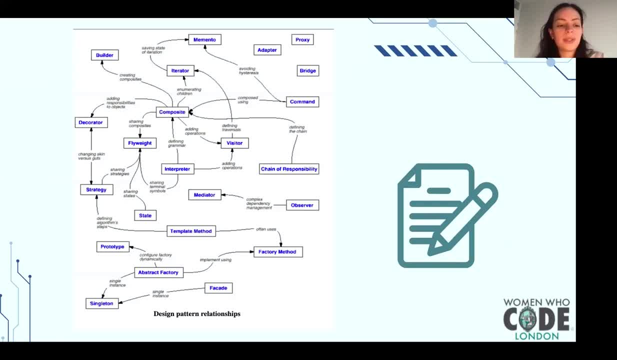 Yeah, Okay, So well, on these sessions we covered already singleton, abstract, factory facade, prototype, factory method, singleton, Yeah, Builder. And today we covered strategy, We covered chain of responsibility, We covered state And we covered iterator. 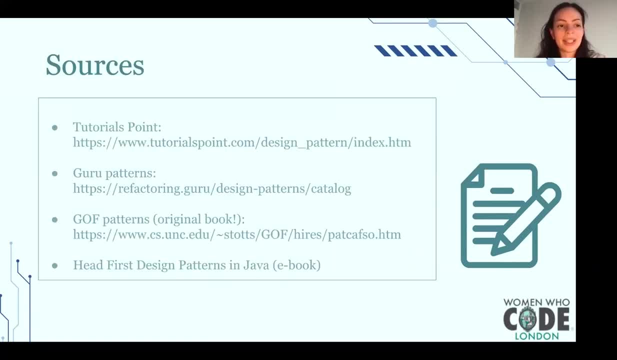 And I hope you liked it. This is sources. This is tutorials point, My favorite in this list. They have very related to real life examples: Group patterns- Very beautiful examples as well- Gov patterns- Well, you don't need to buy original book. 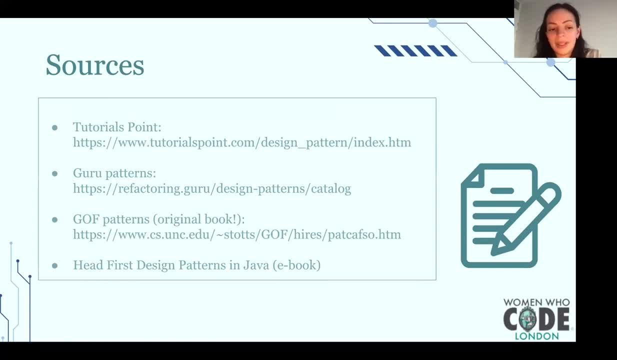 They have very the same thing on the site. And, yeah, you also can refer to head first design patterns, Which is ebook. It can be found for free And you just need to try to find. And they also have very good explanations on design patterns in Java. 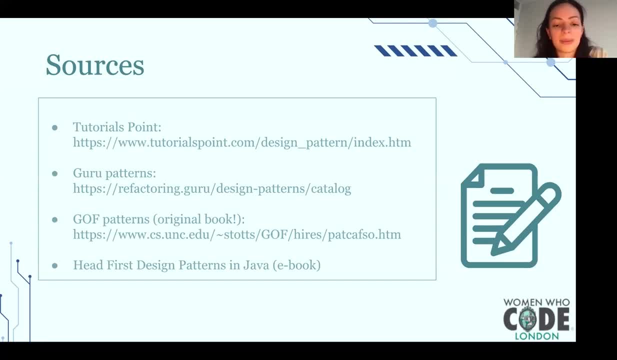 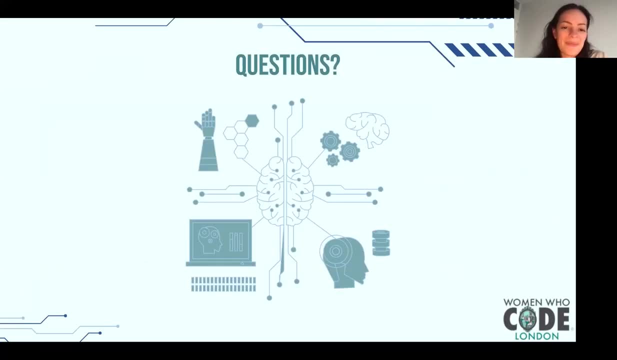 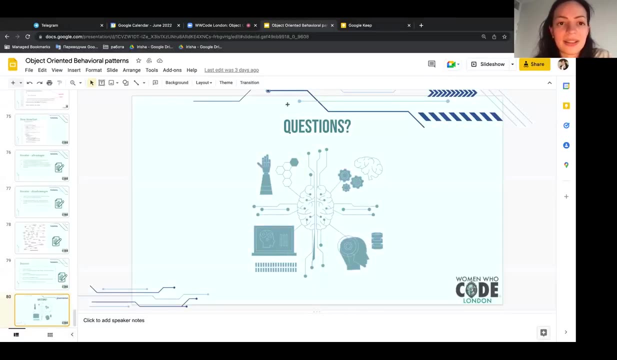 And for design patterns in object oriented programming. Okay, Do you have any questions? Okay, I will stop my presentation. Wow, Thank you for surviving. For people who left here: Oh my God, There was a lot of comments. Oh, I'm sorry. 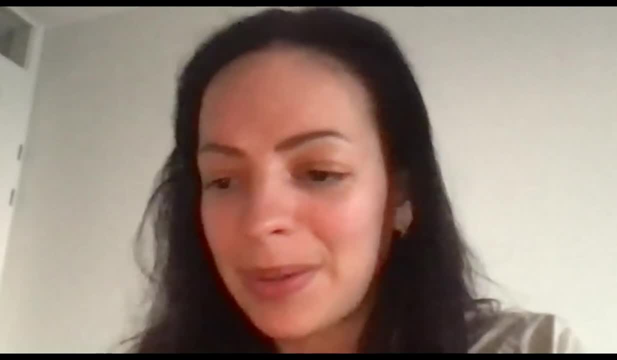 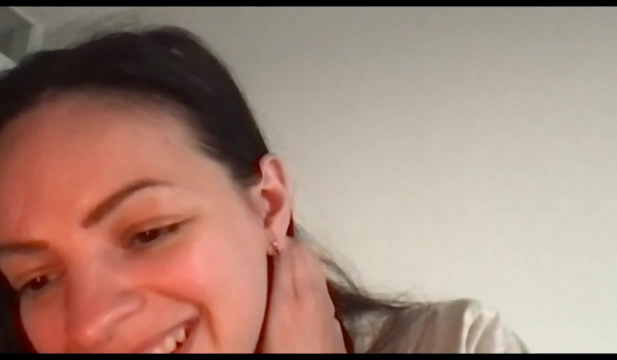 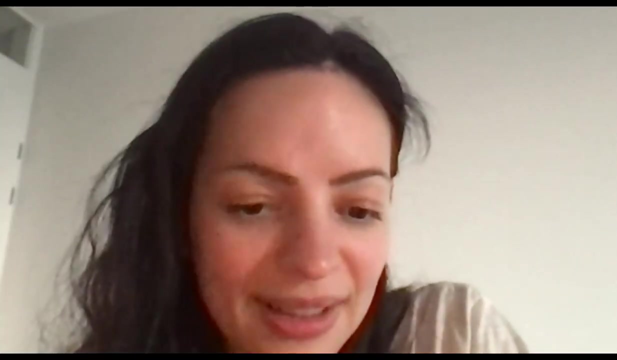 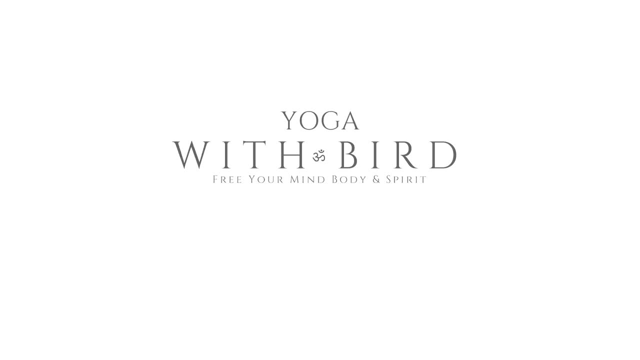 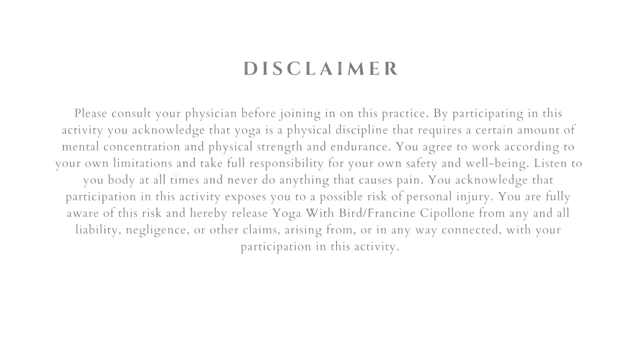 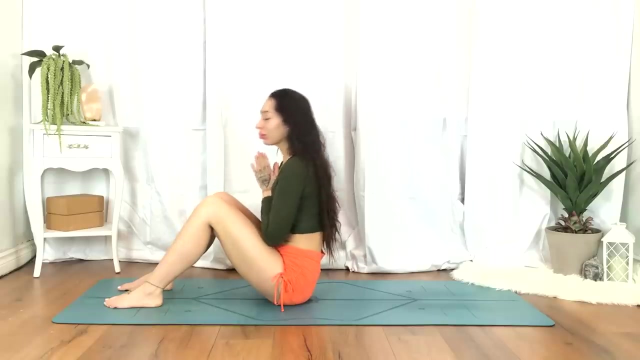 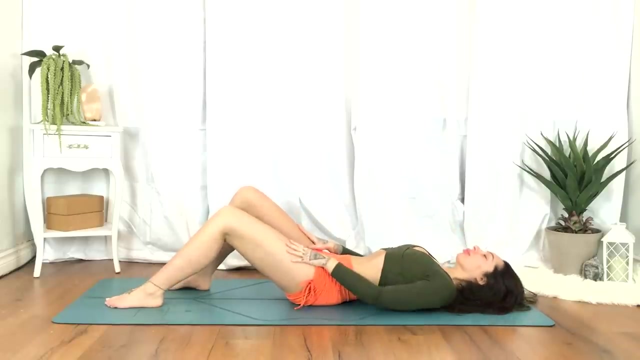 Welcome and good morning. This is a 10 minute morning yoga routine that can be done in bed or right on the mat, Focusing on shaking out that achy back, all those achy sensations in your back muscle and the spine and the neck, shoulders, so you can move more freely throughout your day. Let's begin on our backs, elbows in line with the shoulders, and begin rocking the knees. 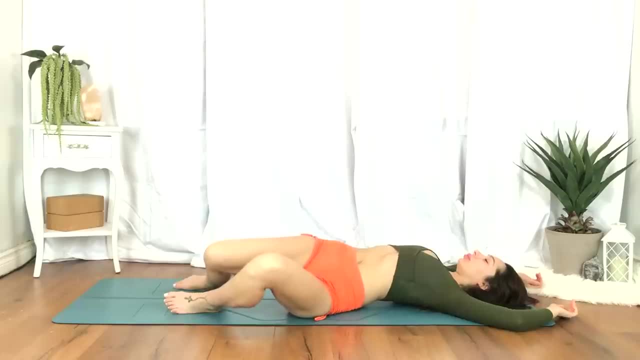 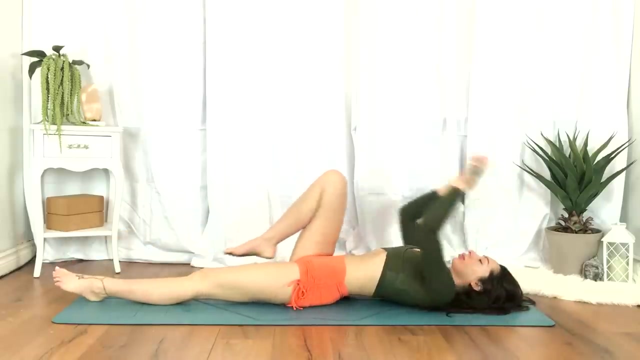 side to side. Straighten the left leg, hugging the right knee towards the chest- Rest here. or begin to draw the knee towards your armpits, just pointing that knee up towards the armpit here, just to open up that hip, that lower back, creating that space in the body. 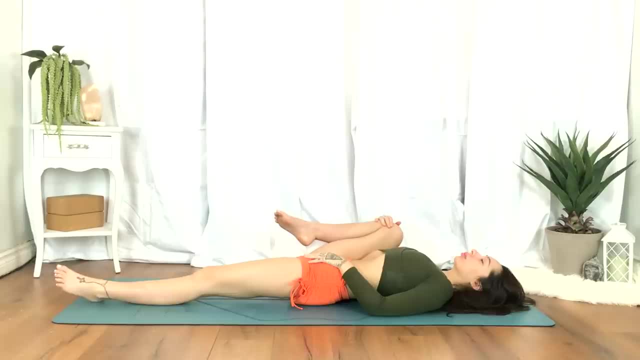 And we'll release, switching legs, hugging that left knee towards the chest, And again, you can rest right here if you'd like to get a little bit of opening in the hips. here You can start to draw that left knee towards the chest. And again, you can rest right here if you'd like to get a little bit of opening in the hips. here You can start to draw that left knee towards the left armpit. And again, you can rest right here if you'd like to get a little bit of opening in the hips. here You can start to draw that left knee towards the left armpit.